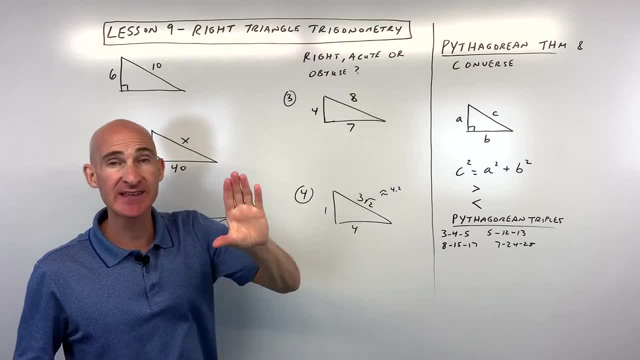 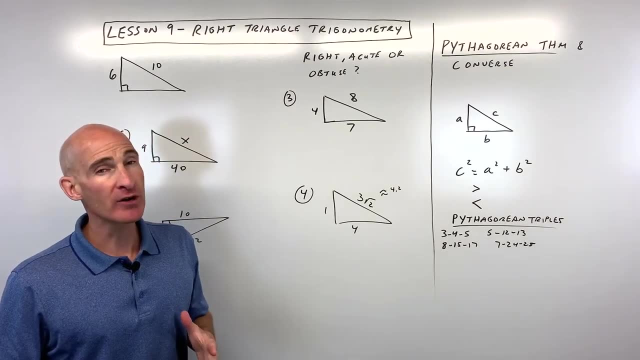 about, And more specifically, we're going to be working with right triangles where it has that 90 degree angle, But the very end of this lesson we're going to talk about triangles that are not right triangles as well. This is an important lesson because you're going to be using this. 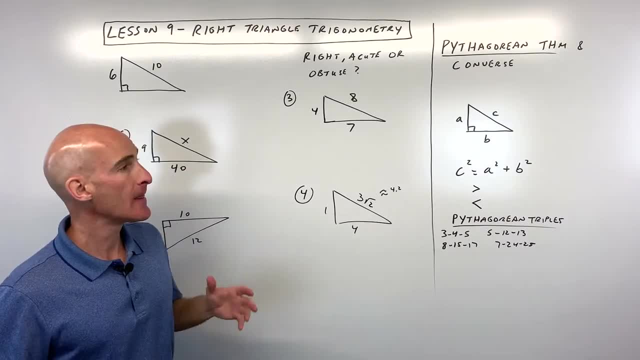 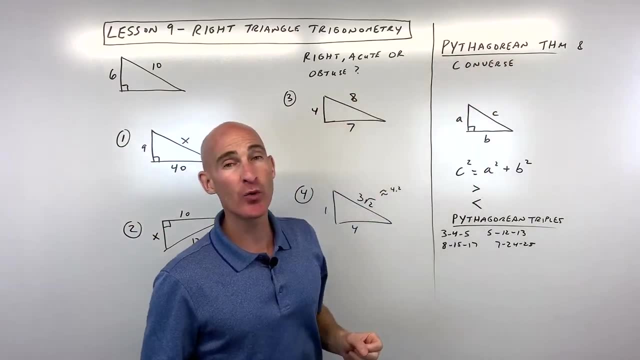 when you get into algebra two and trigonometry and precalculus. So these are kind of the building blocks. So let's start off by talking about the famous Pythagorean theorem and its converse. So what exactly is the Pythagorean theorem? Well, the Pythagorean theorem says that when you have 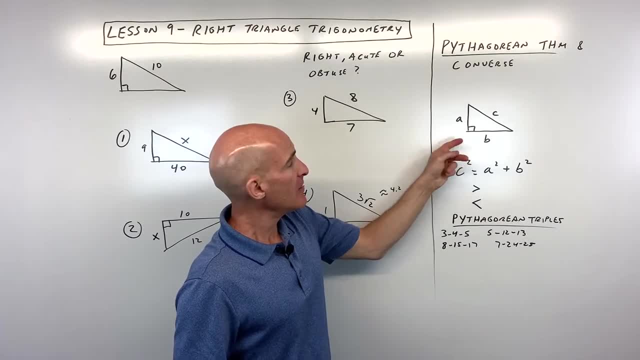 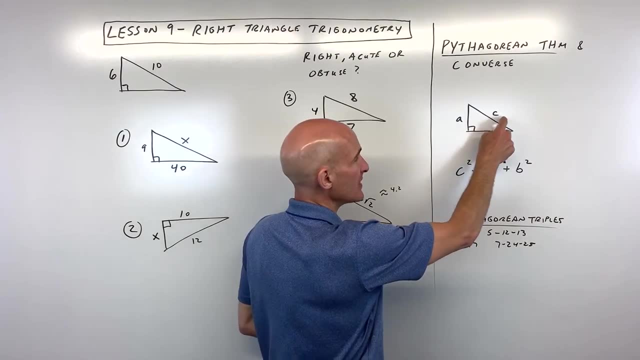 a right triangle, see a triangle with this 90 degree angle that there's this relationship between the sum of the squares of the legs are going to add up to the hypotenuse squared. Okay. so said another way: a squared plus b squared. 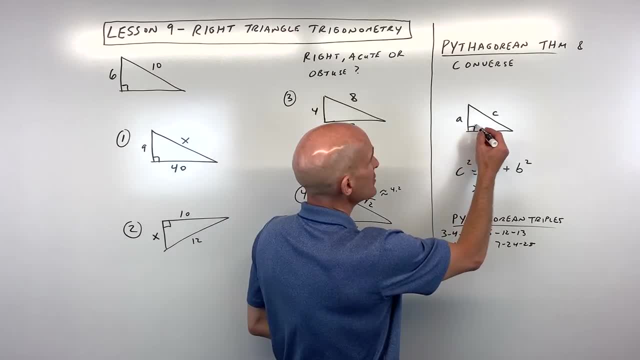 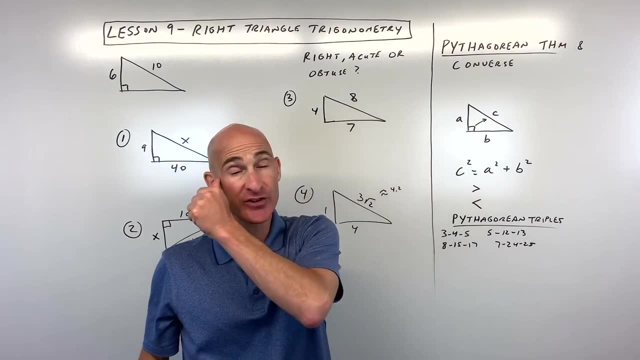 is equal to c squared. Now, remember the C is always going to be the side that's the longest side, it's across from the right angle. So if you know two of these sides, you can find the third side, the missing side. it doesn't have to be, it can be any two sides. you can solve for that. 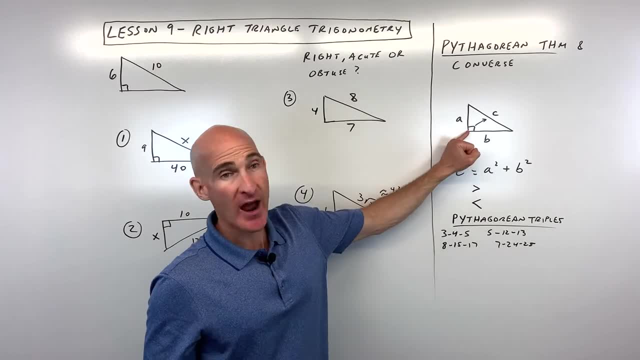 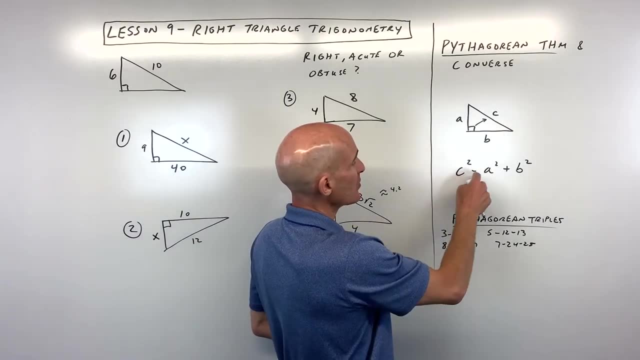 missing third side. Now, if you don't know if it's the right triangle, like say, for example, that right angle, if I cover that up and I'm saying: Hmm, this is triangle, right triangle, well, I can just test it. If c squared is equal to a squared plus b squared, then we know it is a. 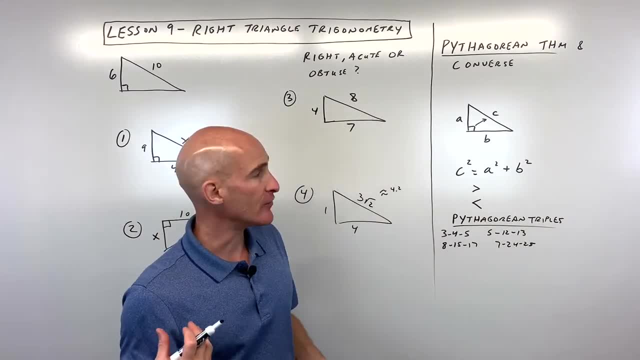 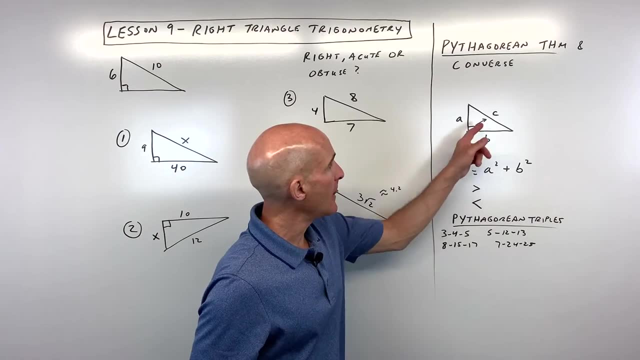 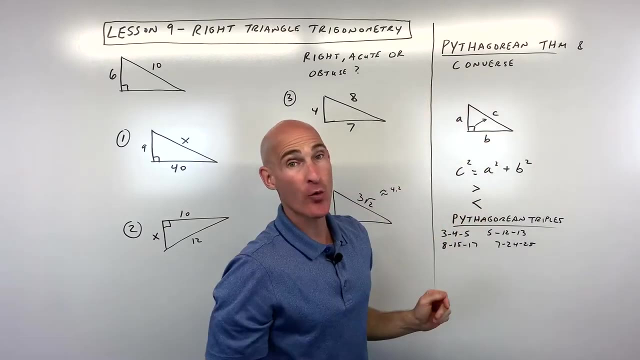 right triangle. So that's saying it in reverse, that's the converse. Now there's also these Pythagorean inequalities where, if c squared is greater than a squared plus b squared, imagine if this side here got longer, longer, longer. what's happening to this angle? it's opening up wider, wider, wider. 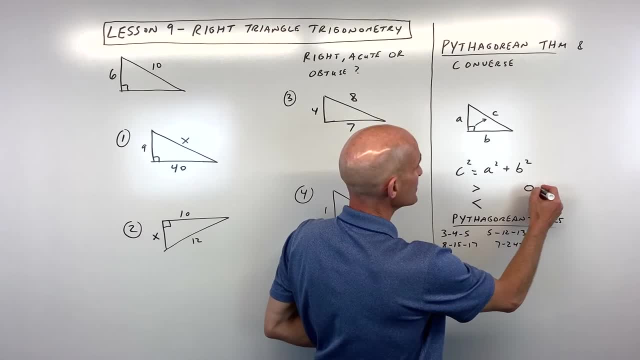 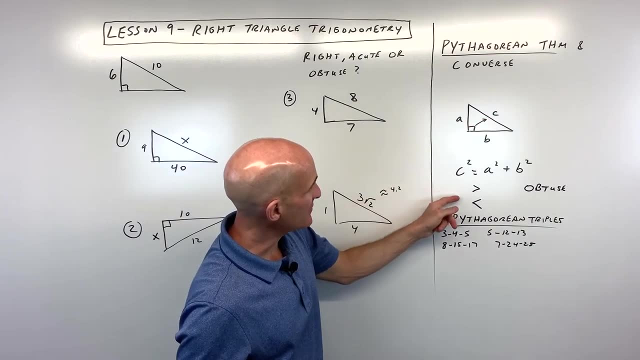 So when c squared is greater than a squared plus b squared, we say it's going to be an obtuse triangle, meaning it has an angle that's greater than 90. And if c is- I'm sorry- if c squared is less than a squared plus b squared, imagine if the c side got shorter, this angle be less than 90,. 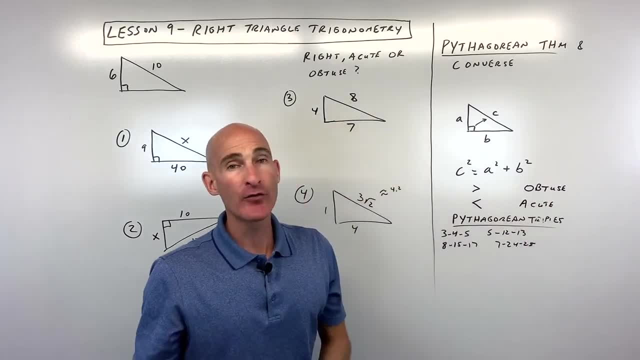 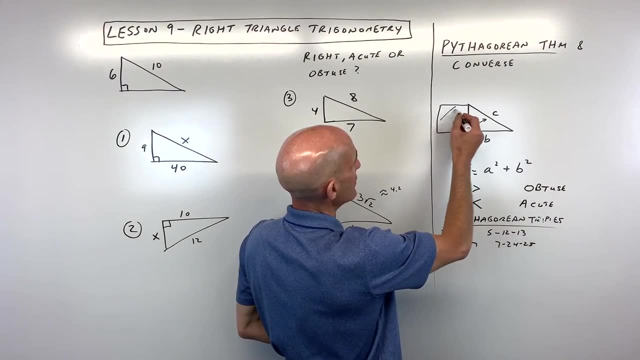 we would say that it's an acute triangle. Okay, now, if you want to see this visually, if you were to find the area of this side like, make us into a square, like a squared, that's the area of this square plus the area of this square, b squared, that's going to equal the area of this square. 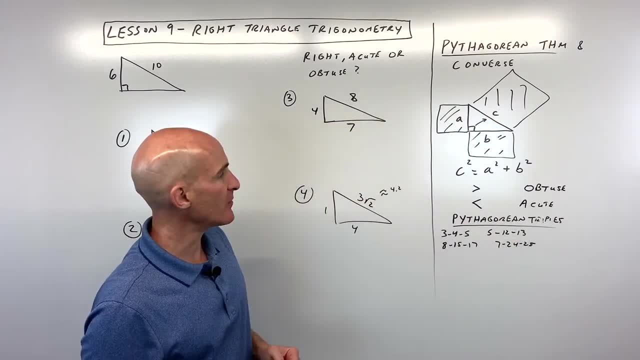 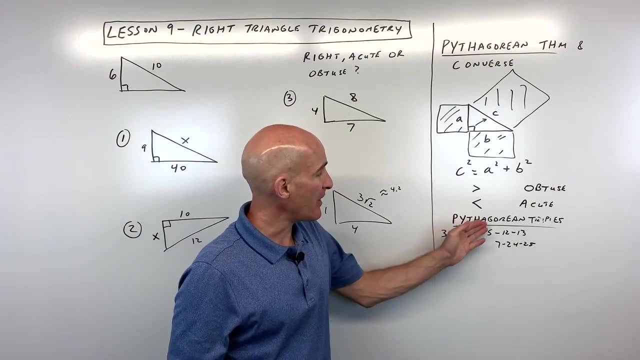 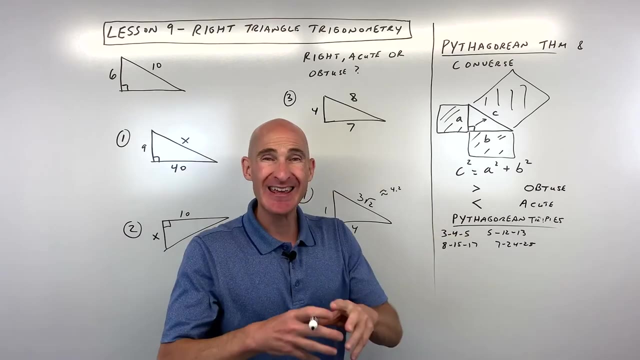 Okay, so that's kind of a geometric visualization of the Pythagorean theorem. When you work with these Pythagorean theorems, sometimes what comes up are what are called Pythagorean triples. What's a Pythagorean triple? Well, triple means three right, And it's when the side lengths are integer. 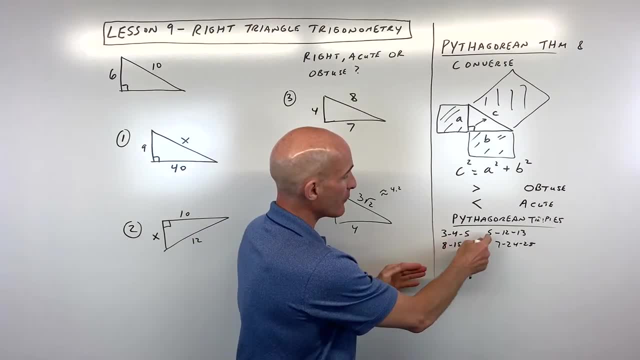 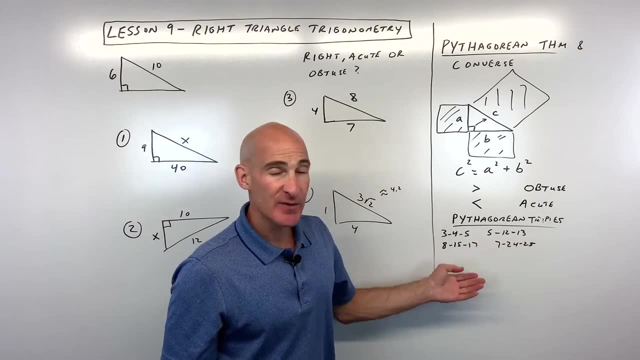 values. So they work out really nice, like three, four, five or five, twelve, thirteen. You don't get any decimals or fractions or square roots, So these four are really good to memorize because they come up a lot in problems, And I'll show you an example of how you can utilize them. 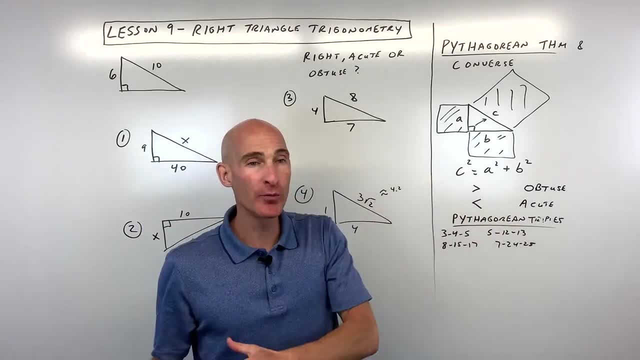 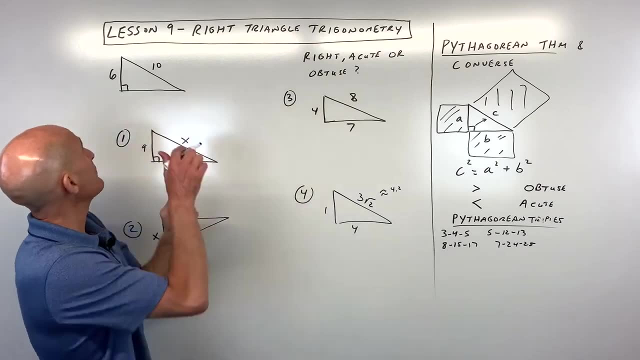 Because these Pythagorean triples- you can also have multiples meaning, like if I had, let's say, I multiply these all by ten, thirty, forty, fifty would also make a right triangle. So say, for example, like this one: 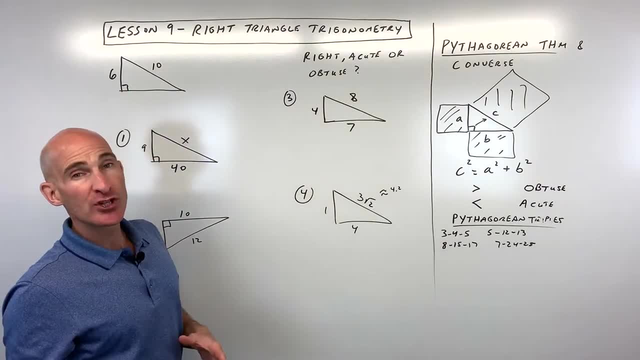 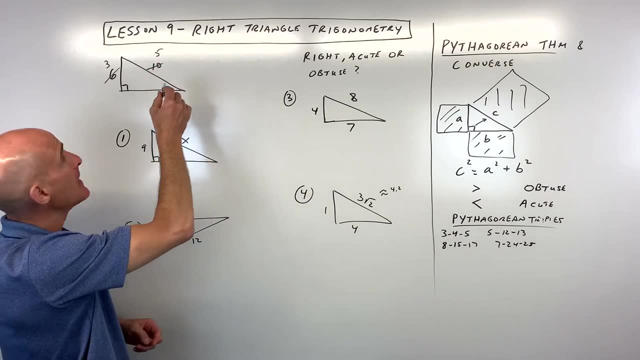 we've got six, ten and we're trying to find this missing side. What you can do is you can say: well, it looks like two goes into six three times and two also goes into ten five times. So I can see that this is a three, four, five Pythagorean triple. Okay, this first one here. 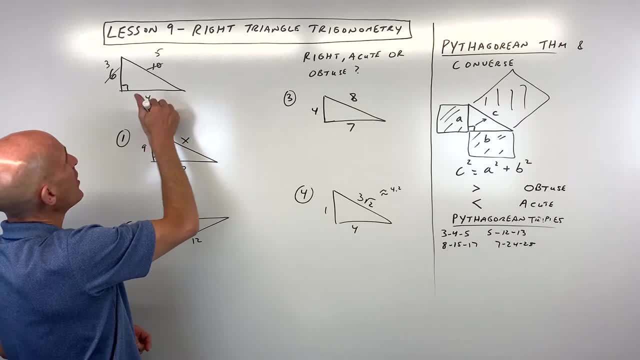 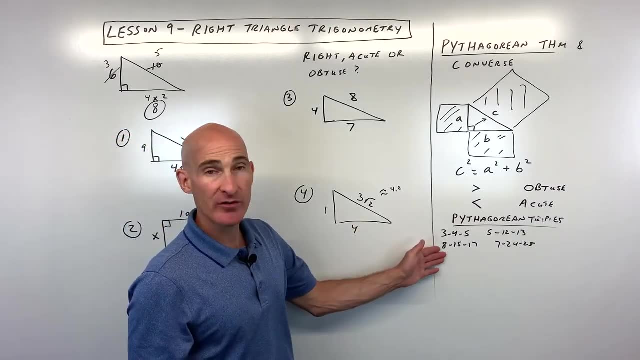 But because I doubled both of these, I'll have to double this one as well, and then I'll divide this by two. So that means this missing side length is eight. So it's just a quicker way of finding the missing side, if you remember these Pythagorean triples. 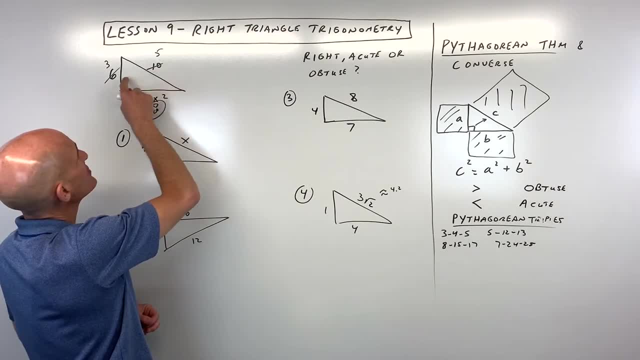 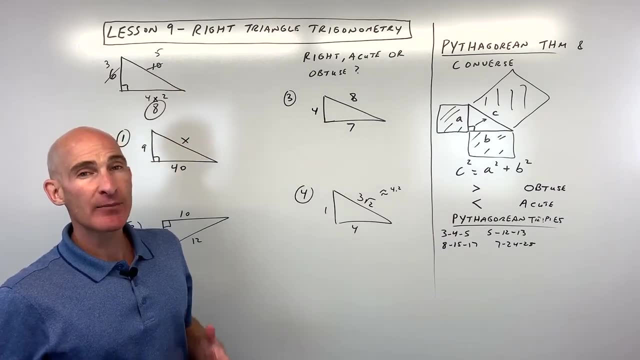 and if you can recognize them, You want to find the greatest factor, the greatest number that divides into here, to kind of reduce it down to these basic ones to help you find that missing side. So let's go through some examples. I'll show you how this works as we go. So for number one. 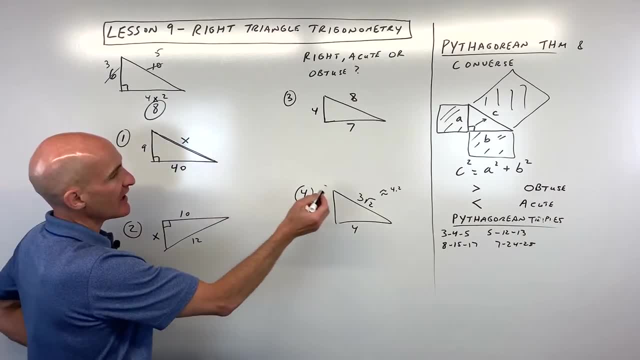 we want to find this missing side here. Now the question is: is it A, B or C? Well, you can see, it's the one that's across from the right angle. So that's how we're going to find the missing side. 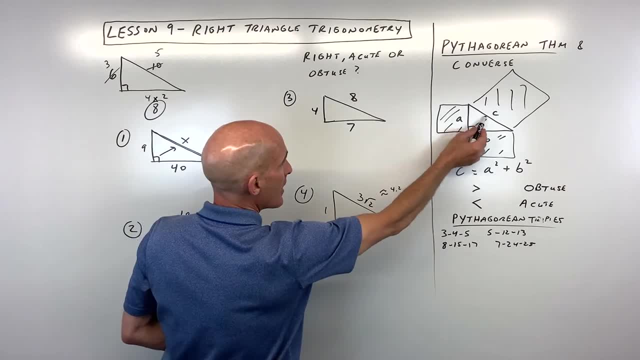 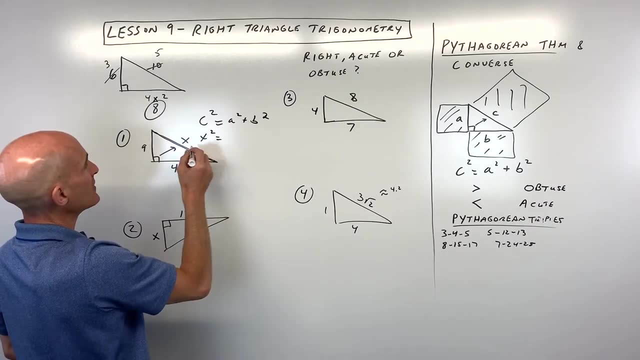 That's the one that's across from the right angle. So that's our C side, our hypotenuse. So if we write our Pythagorean theorem, C squared equals A squared plus B squared, we have: X squared equals nine squared plus 40 squared. Okay, and nine squared is 81.. 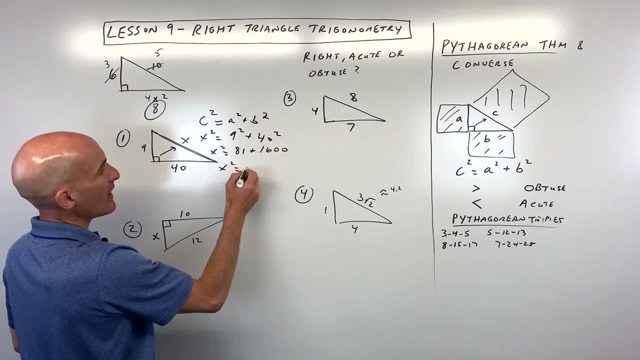 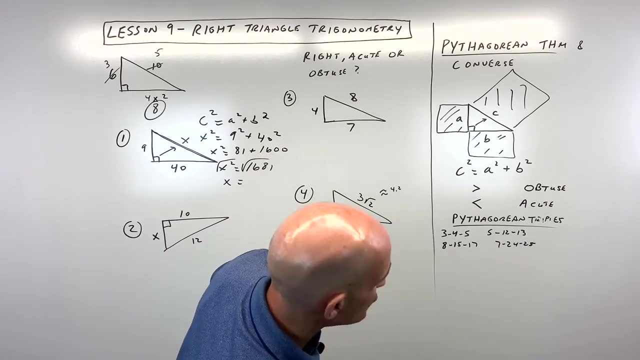 40 squared is 40 times 40. That's 1600.. X squared equals 1681.. And if we take the square root of both sides, we get- let's see what that comes out to. I believe it's 41. But just to verify. 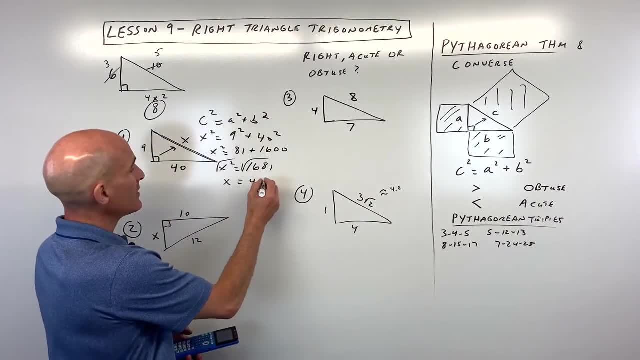 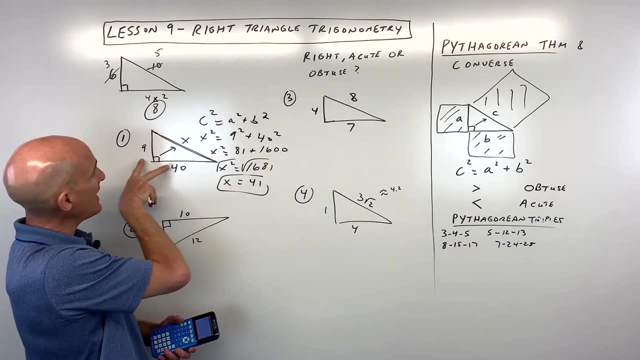 41.. So that's all you have to do Now. sometimes people will ask: you know, Mario, how do you know that this side was A and this side was B? Well, with the legs it doesn't really matter, It can be. 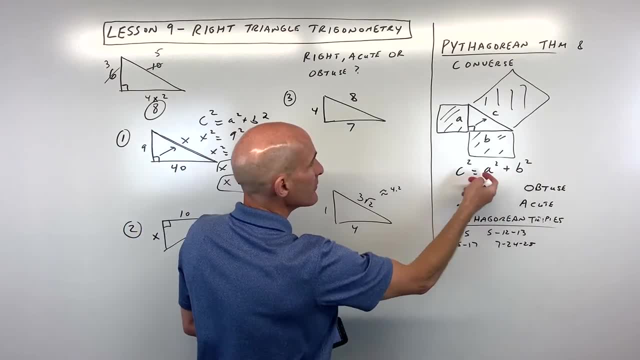 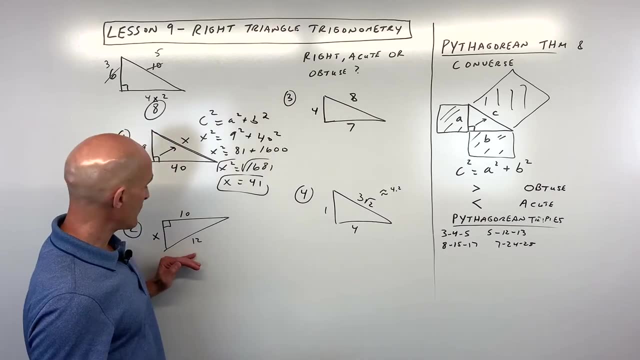 either order, because addition is commutative. But you want to make sure the side across from the right angle- that's always your C value- That's on its own, on its own side. So for number two, what do you think for this one? How would you solve for this missing side here, X? Well, 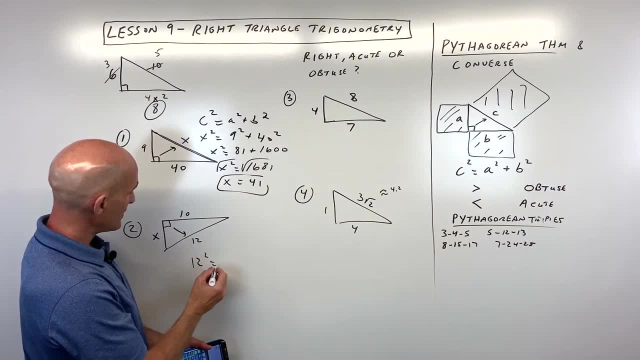 we can see that here's our 12.. So that's going to be the missing side here. And then we're going to be: 12 squared equals X squared plus 10 squared. So let's see, 12 squared is 144.. 10 squared, we. 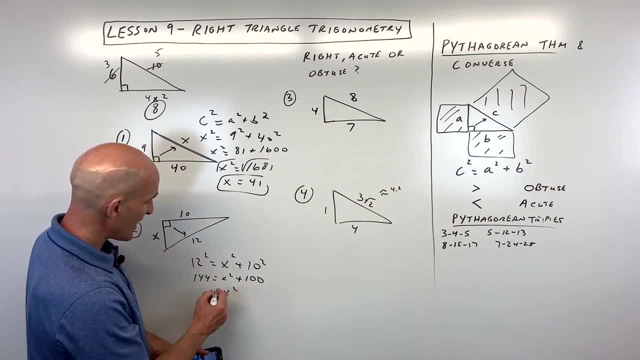 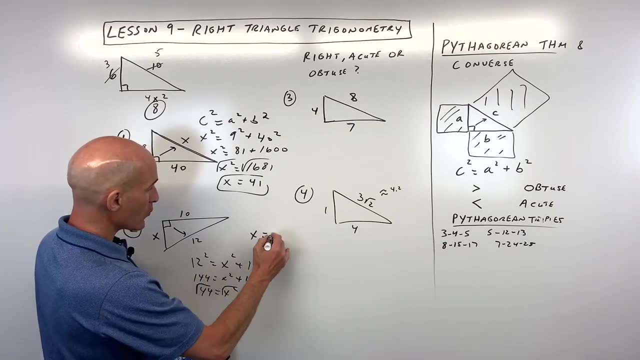 know, is 10 times 10, 100. If we subtract 100 from both sides, we get 44. And if we take the square root to get X by itself, we get the square root of 44, which is 4 times 11.. And the square root of 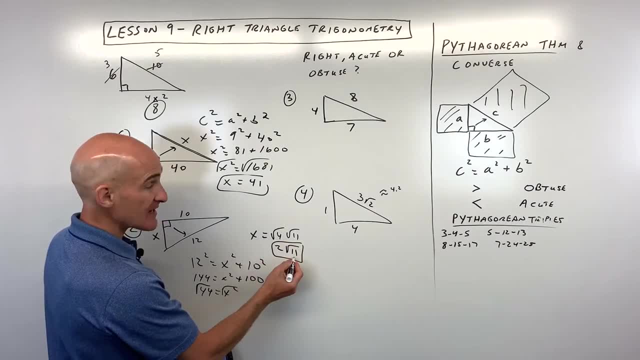 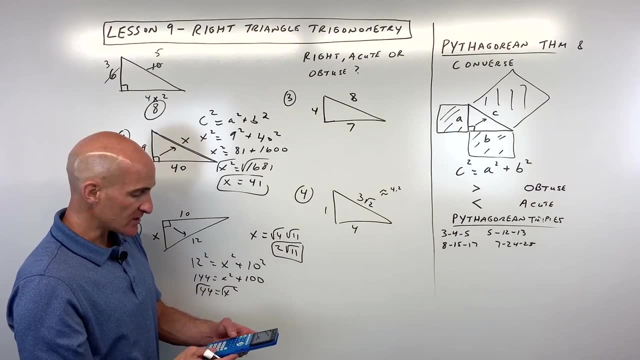 4 is a perfect square. that's 2.. With the square root of 11, that's not a perfect square. So this is simplifying square roots. It's a decimal, So I'll do that real quick. for us It's about 6.6 approximately. Okay for number. 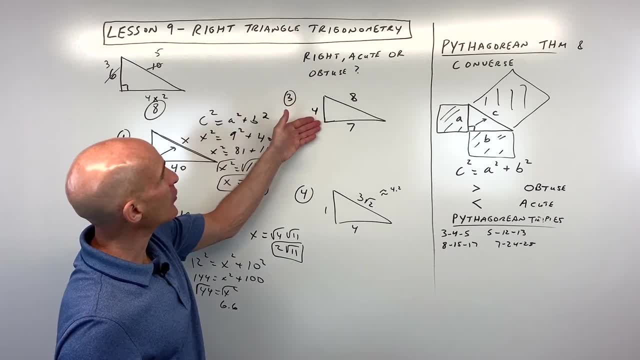 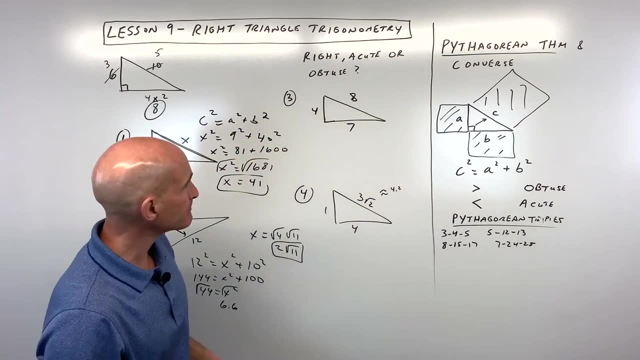 three and four. the question is, is the triangle a right triangle, an acute triangle or an obtuse triangle? And that's where these Pythagorean inequalities come into play. The main thing here you want to remember is to find the C side, And C side is always going to be the longest side In. 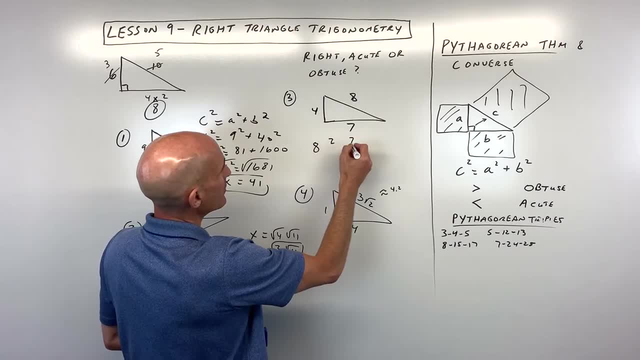 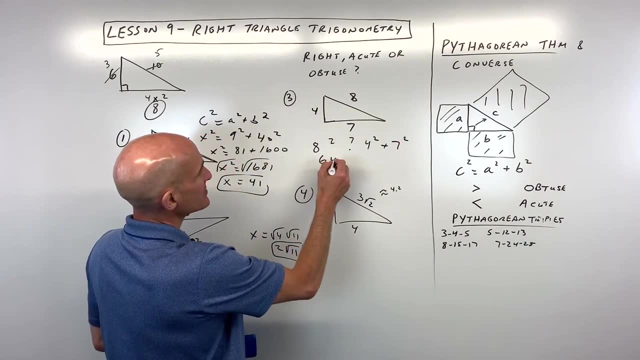 this case it's 8.. So we're saying: is 8 squared greater than, less than or equal to A squared Plus B squared? Okay, So 8 squared is 64.. 4 squared is 16.. 7 squared is 49.. This comes out to 65.. It 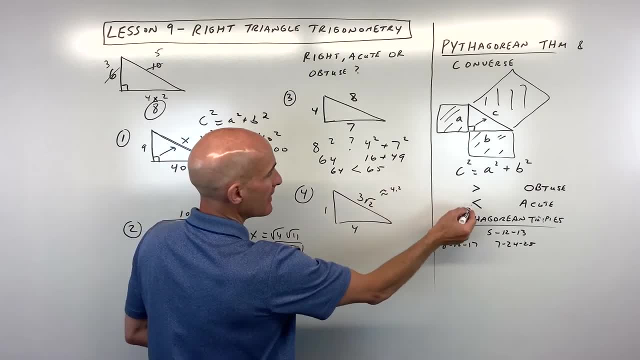 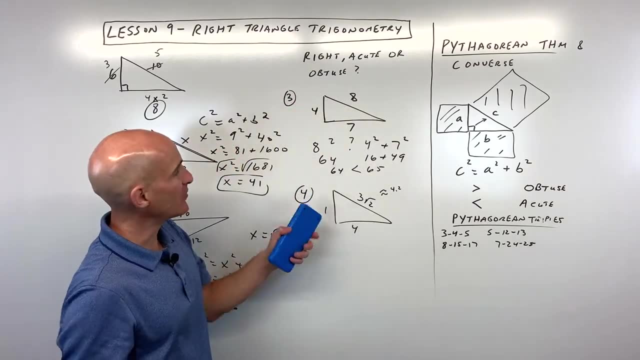 looks like 64 is less than 65. That means that it's an acute triangle. So this might be like who knows, 89,, 88 degrees, something like that. a little bit less Okay, so we'll write acute for this one Now. 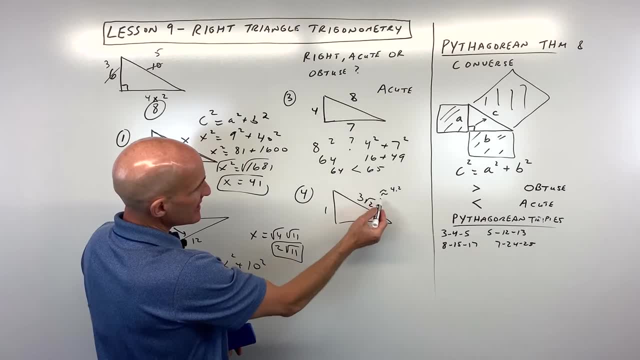 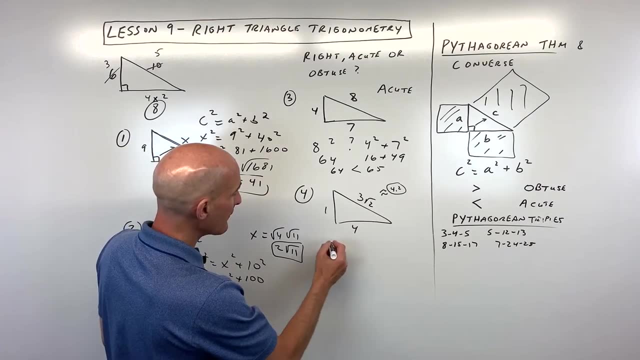 how about for number four? Well, this one, the longest side, is going to be this 3 square root of 2 side. I mean the calculator. it's about 4.2.. So we know, that's our longest side. So we have 3 square root of. 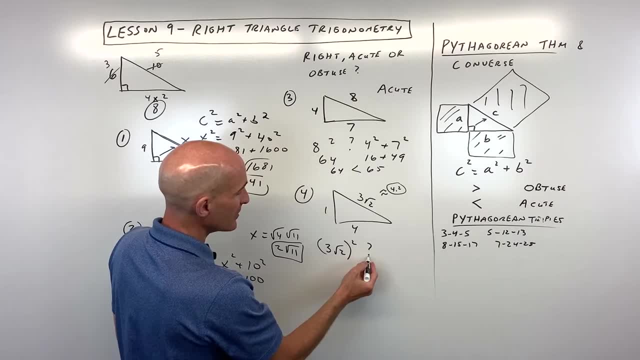 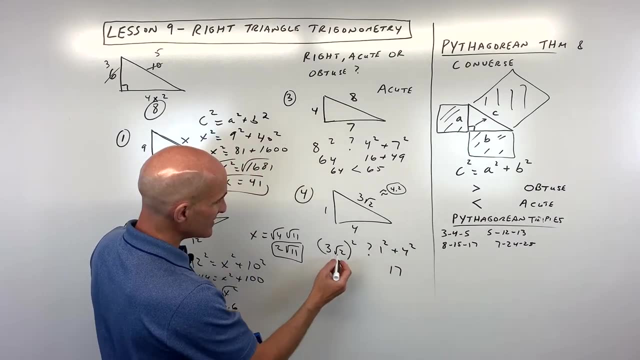 2 squared question mark meaning greater than, less than or equal to 1 squared, plus 4 squared. 1 squared is 1.. 4 squared is 16.. So if we add those together we get 17.. Here, 3 square root of 2. 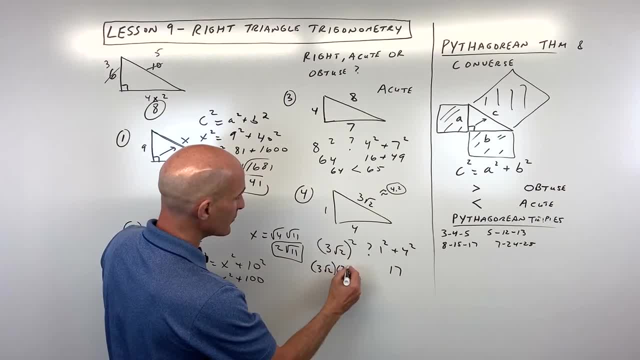 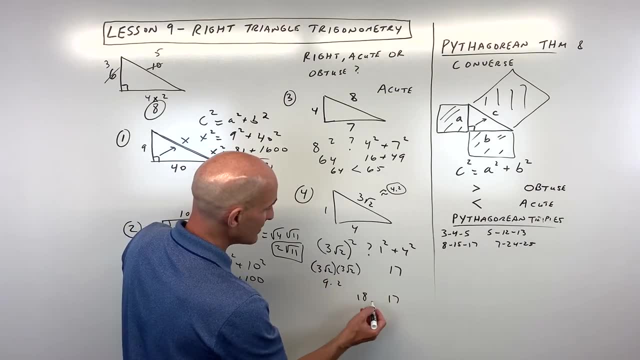 squared. that's like 3 root 2 times itself. right, when you square something 3 times, 3 is 9.. Square root of 2 times square root of 2 is 2.. So this comes out to 18,, which is greater than 17,. 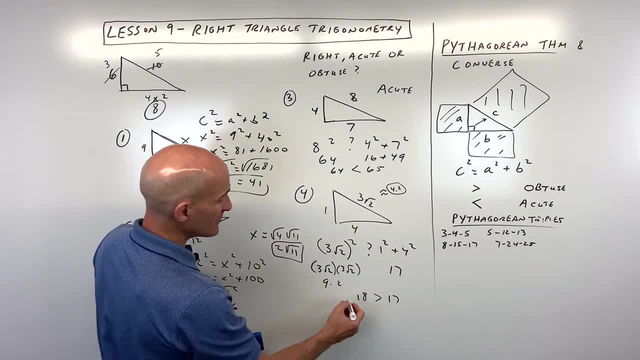 right. So we know that's our longest side. So we know that's our longest side, So we know that's 18.. So here this angle is actually going to be greater than 90.. It's going to be an obtuse. 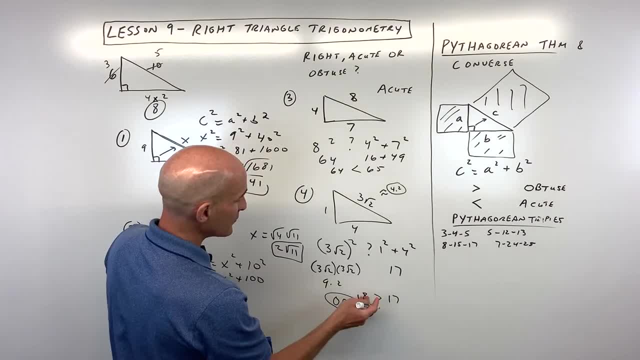 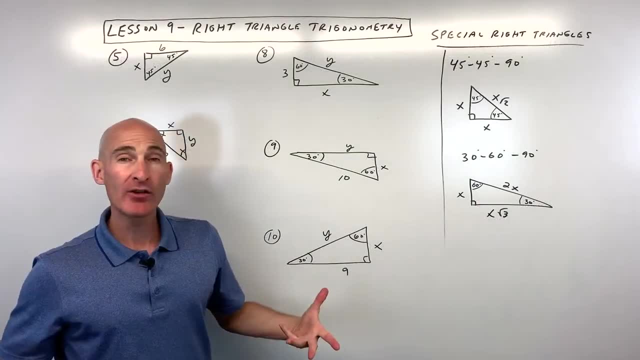 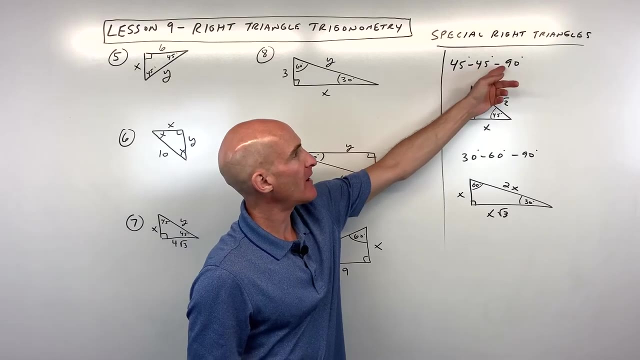 triangle. Now what would happen if it was 18 equals 18?? Well then, it would be a right triangle. So some formulas you want to memorize, Okay. now let's talk about special right triangles. So what are special right triangles? These are the triangles that are the 45,, 45,, 90, meaning that 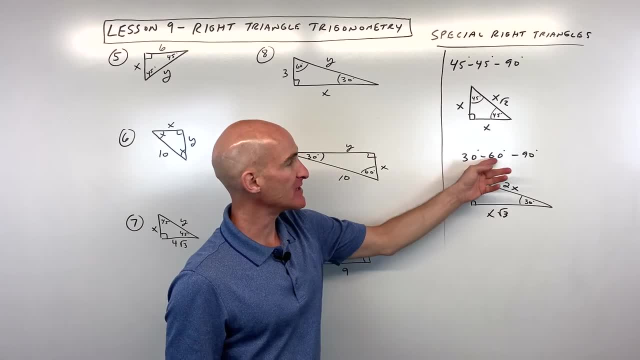 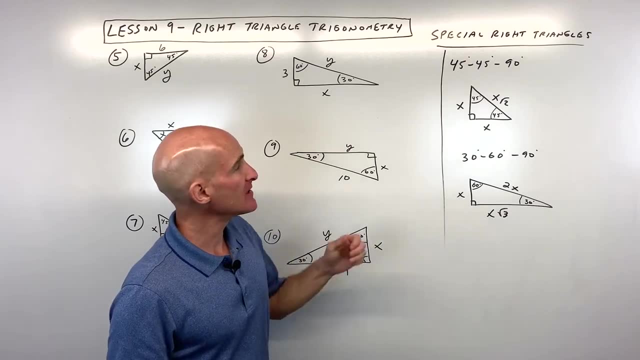 the angles are 45 degrees, 45 degrees, 90 degrees and 30,, 60,, 90. So when you see these triangles, instead of using the Pythagorean theorem, it's easy to find the missing side lengths using these. 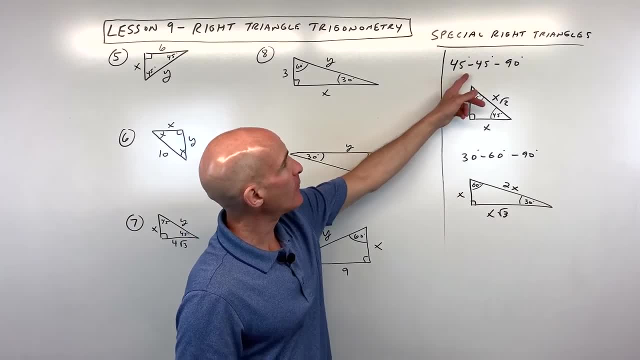 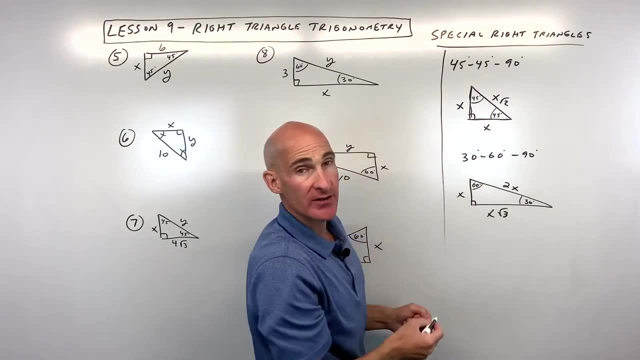 ratios I'm about to show you here in a moment. So when you have a 45,, 45, 90 triangle, the two legs, the two sides that make up the right angle, these are going to be congruent. So it's an isosceles. 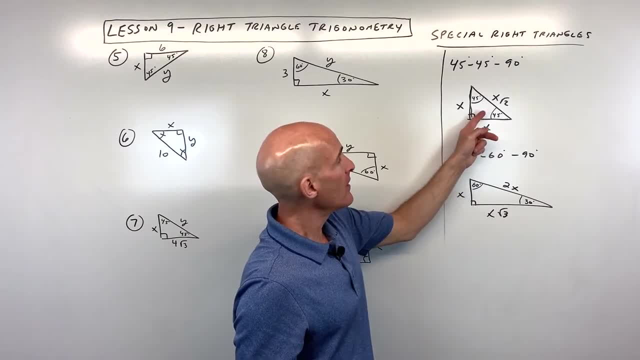 triangle. So you know this is 4, then you know this one's 4.. The hypotenuse is always going to be, whatever the leg length is, times the square root of 2.. Square root of 2 is about 1.4, so it's. almost one and a half times longer than the right angle. So when you have a 45,, 45,, 90, 90 triangle, square root of 2 times square root of 2 is about 1.4, so it's almost 1.5 times longer than the right angle. So 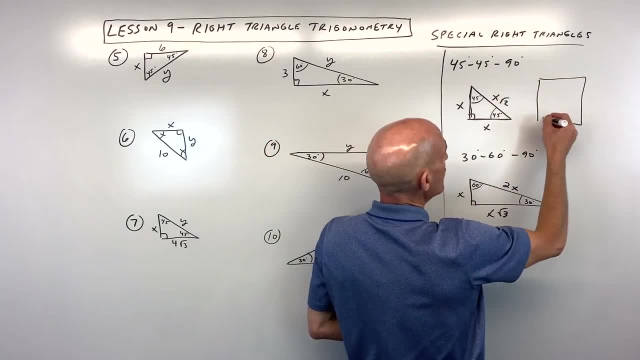 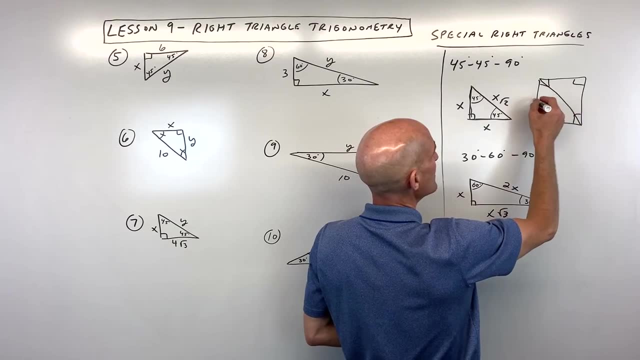 You can kind of think of this as a as a square. Okay, in a square We know we have the four right angles and if you draw that diagonal, okay, It's gonna bisect this angle. so you can see, all the sides on a square are congruent. 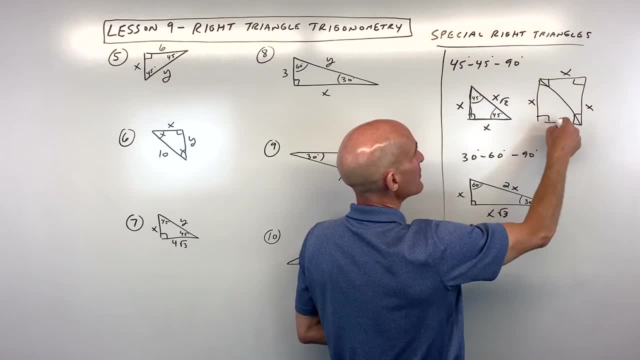 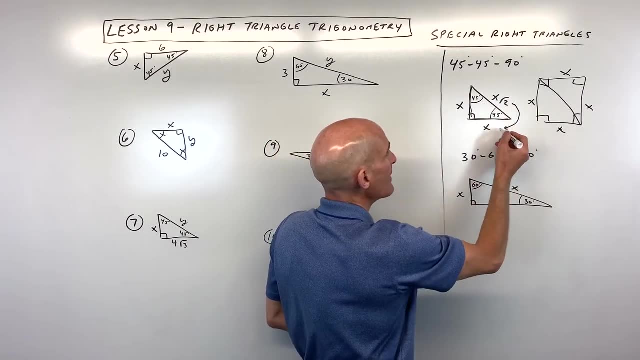 X, X and X right, and then that diagonal. if you do the Pythagorean theorem, You'll see that this comes out to X, square root of 2.. Now what happens if they give you the hypotenuse? Well then, all you have to do is divide by the square root of 2. if they give you the leg, you multiply by the. 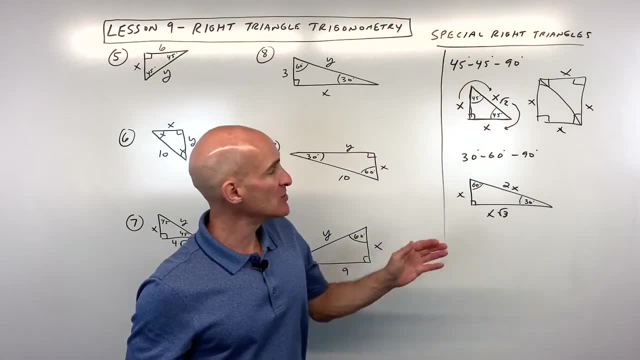 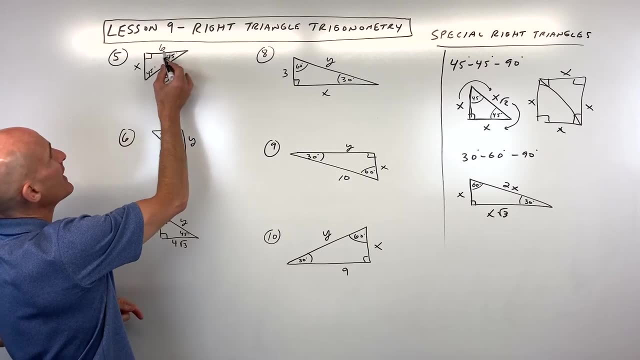 Square root of 2.. So the 45-45-90 is a little bit easier than the 30-60-90.. So let's work with this one first. So say, for number 5, here it's a 45-45-90. 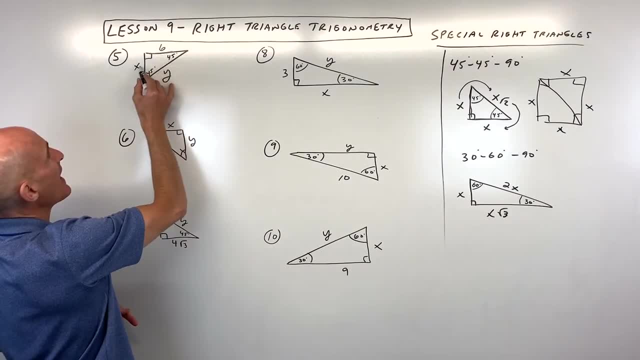 You can see that they give us the leg length of 6. We know that X is the same because the two legs are congruent. so we can say here X equals 6. and Then to get from the leg to the hypotenuse, We know the hypotenuse is always, you know, about 1.4 times longer, square root of 2 times longer. 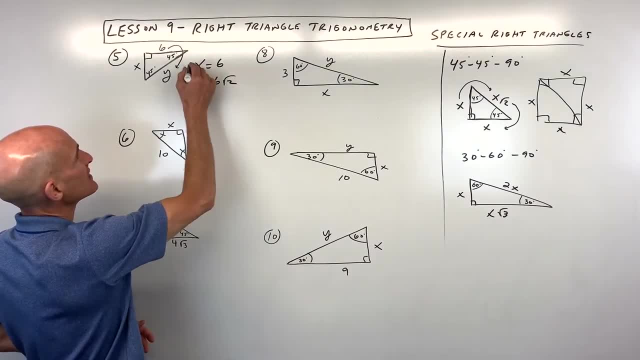 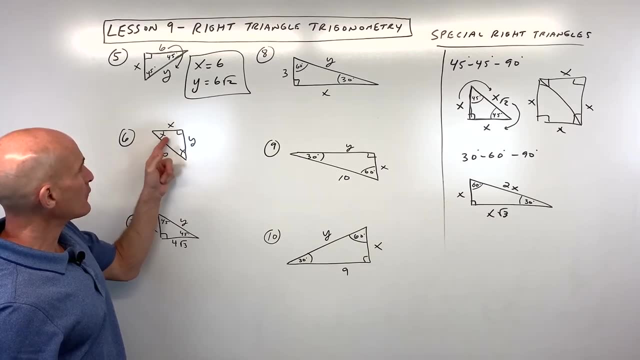 So Y is going to be 6 times Square root of 2. this is like an exact answer. Okay, let's try number 6.. This one's a little bit more challenging here. notice that they don't tell us that these are 45 degree angles. 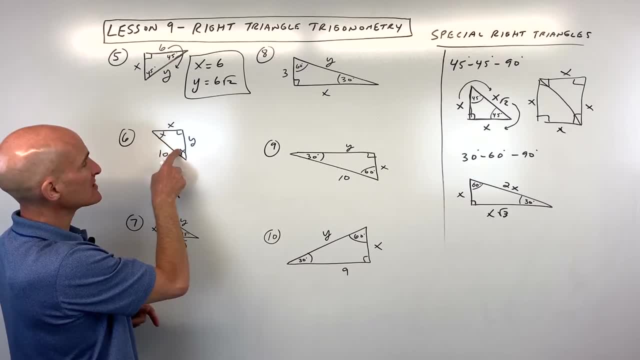 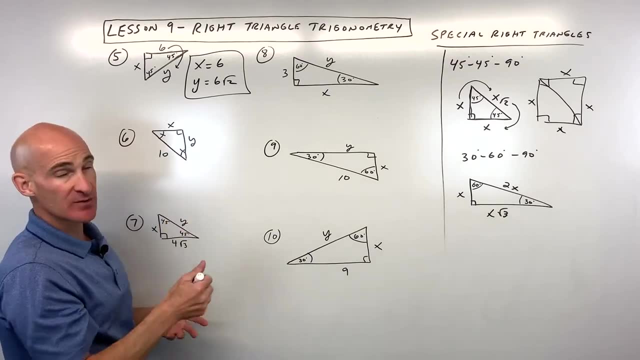 But because we can see that they're congruent to each other. We know they're the same and all the angles in a triangle up to 180. So you can see, if this is 90, these two have to add up to 90. if they're congruent, that each must but be 45. 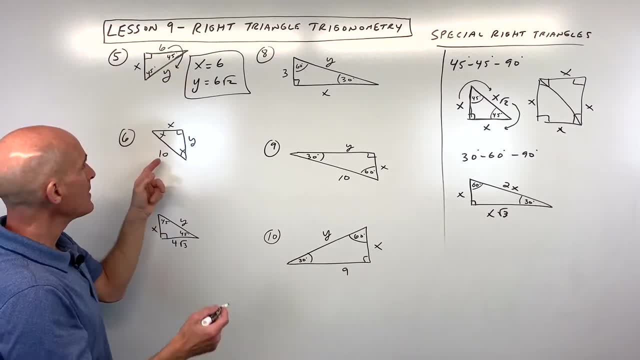 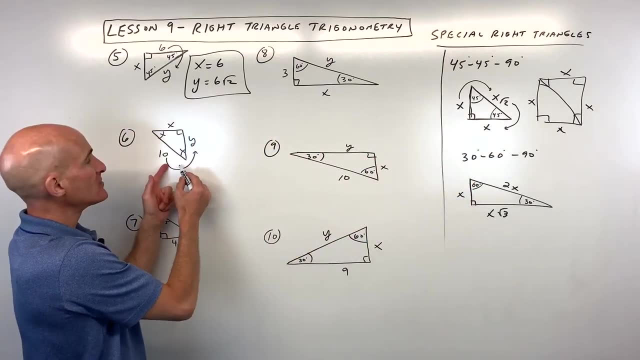 So sometimes you'll see this instead of the 45-45-90, but here what they're giving us is the hypotenuse. How do we go from the hypotenuse back to the leg? Well, we have to divide by the square root of 2. so let's look at 10 divided by square root of 2. 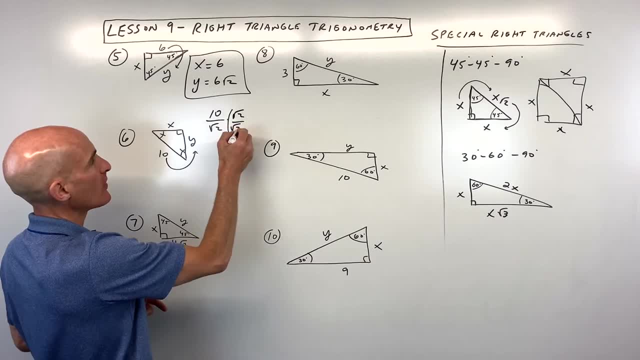 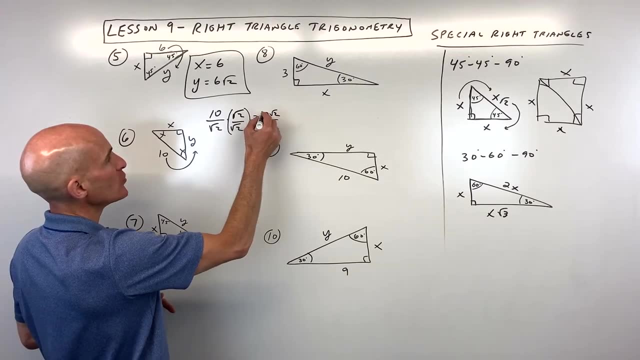 We don't want the radical in the denominator, So we're going to rationalize by multiplying by square root of 2 over square root of 2, that's like 1, So this gives us 10 square root of 2 over square root of 4, which is 2, and the 10 and the 2 we can reduce. 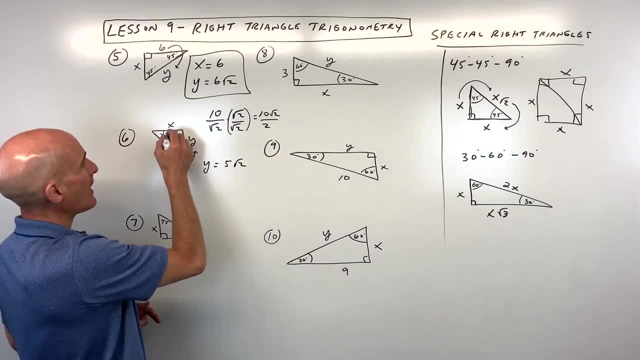 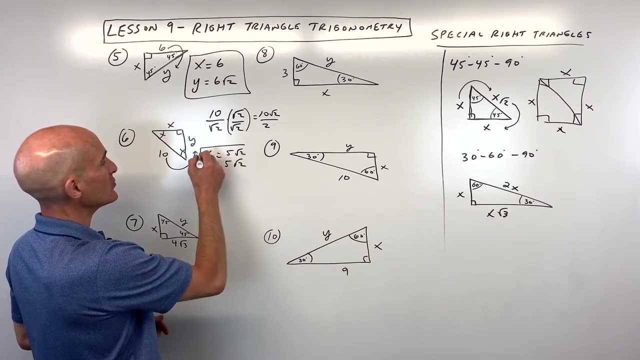 So you can see that Y equals 5 square root of 2. X and Y are both the legs or the sides. those are congruent. so X is also equal to 5 square root of 2. Okay for number 7, a little bit more challenging. here We've got another 45-45-90. 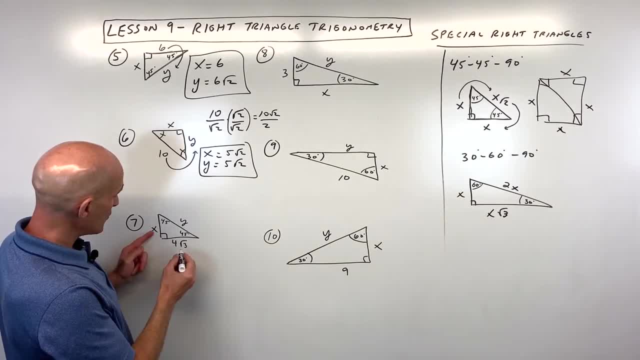 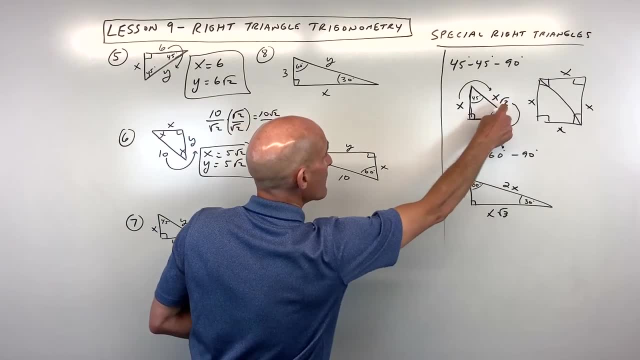 You can see they're giving us the leg length of 4 root 3. So we also know this other leg is going to be 4 root 3. How do we get from the leg to the hypotenuse? Well, you can multiply by the square root of 2. that's like about 1.4. 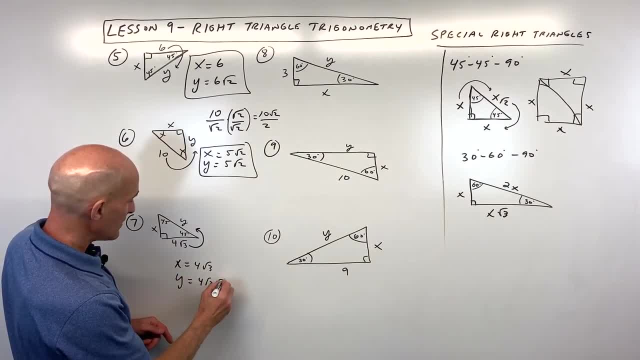 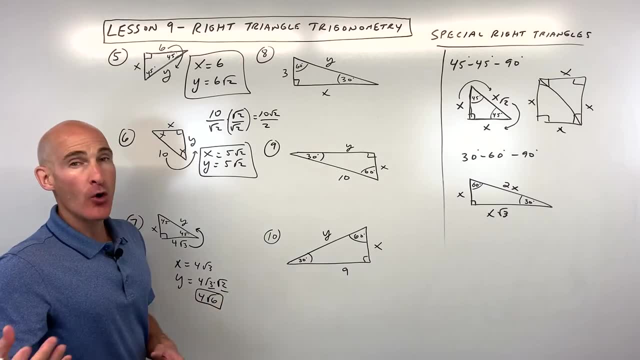 So we have: Y equals 4 square root of 3 Times the square root of 2. you multiply the 2 square roots together and that comes out to 4 square root of 6. Okay, now let's talk about the 36th square root of 2. 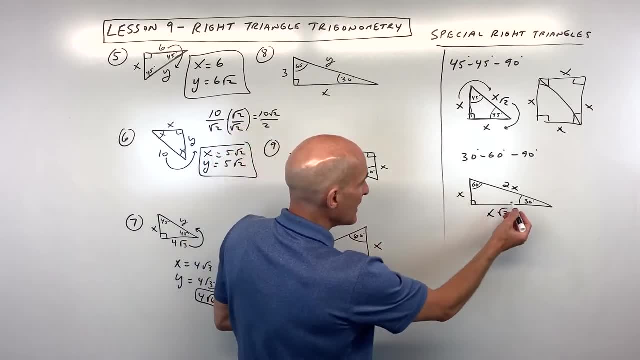 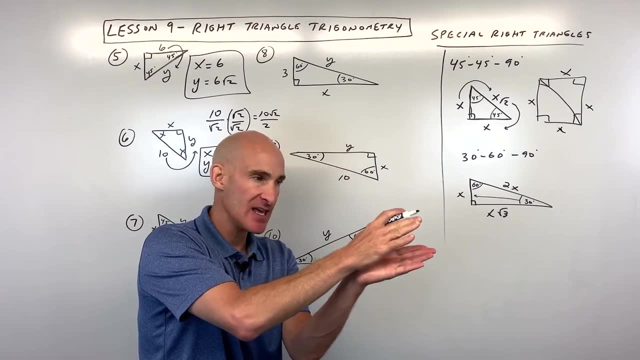 So with the 30, 60, 90, the side that's across from the 30 degree angle, that's going to be the short leg. Okay, So if you think about like a, an angle, like a hinge, if you open that up just a little bit, The side that's across from that small angle is going to be the shortest side. 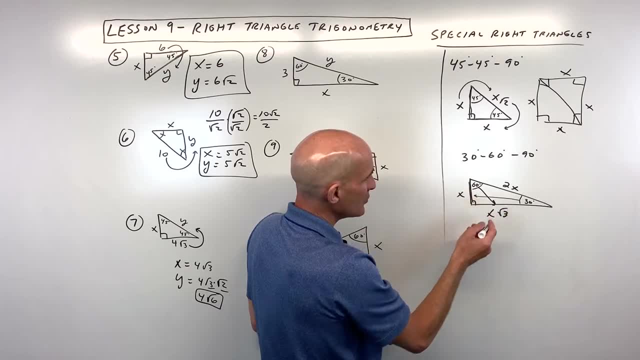 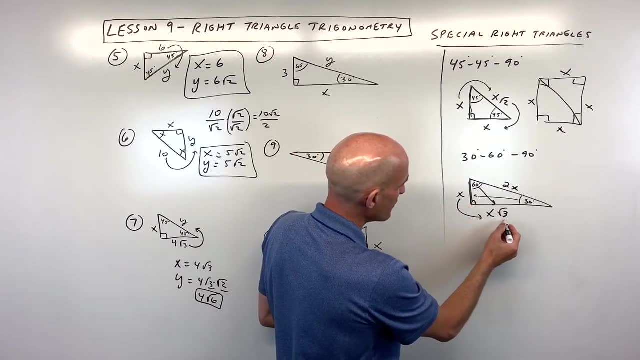 That's, we call this side X, the one across from the 60 degree angle. now We're opening up a little bit wider. That's going to be X times the square root of 3, meaning, whatever this side is, we're multiplying by square root of 3. 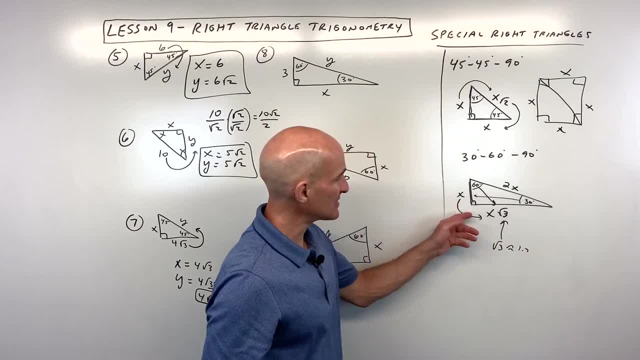 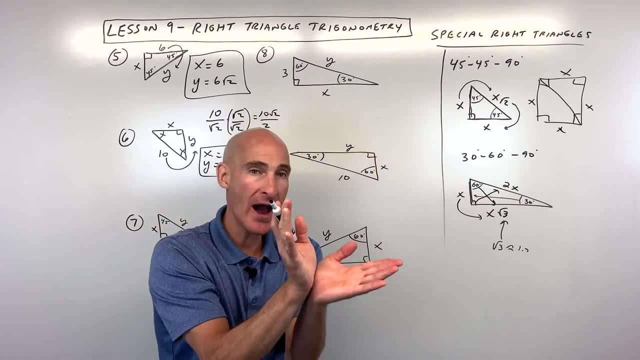 Square root of 3 is about 1.7. So this leg here is about 1.7 times longer than this leg, and then the one across to the 90 degree angle. now We're opening up even wider. that side is going to be the longest side. It's going to be 2 times the short leg, so 2x. 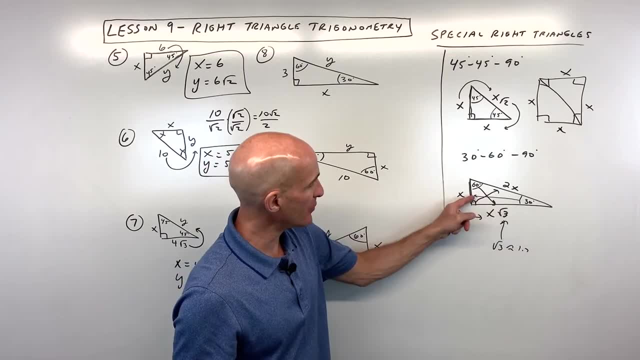 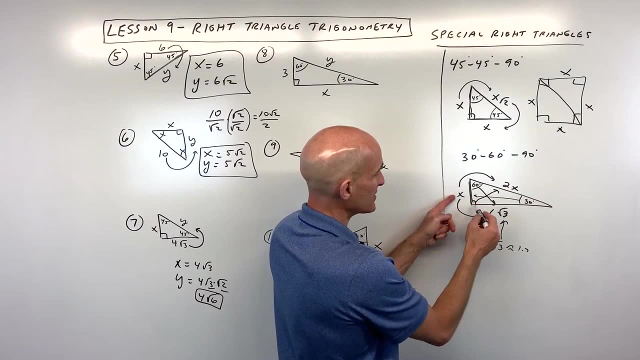 So what you can do is, if they give you the short leg and the one across from the 30, It's pretty easy. You just have to double it to get the hypotenuse, or multiply by the square root of 3, which is about 1.7. 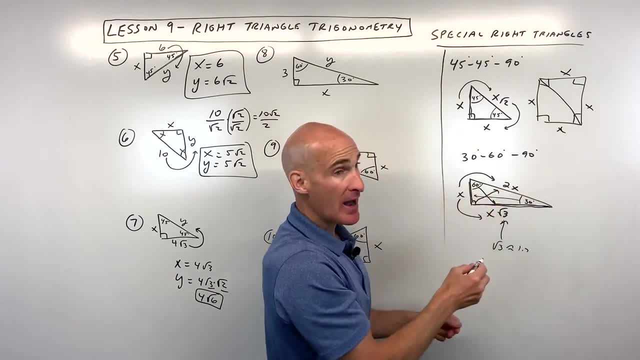 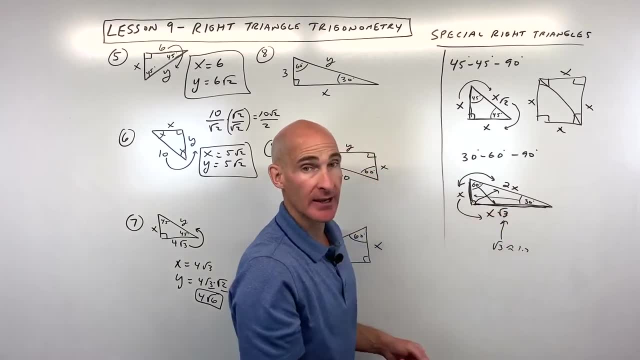 To get the longer leg. if they give you the hypotenuse, It's pretty easy. You just have to divide by 2, that'll give you the short leg, and then multiply by square root of 3, that gives you the longer leg. The tougher one is when they give you the longer leg. you have to then 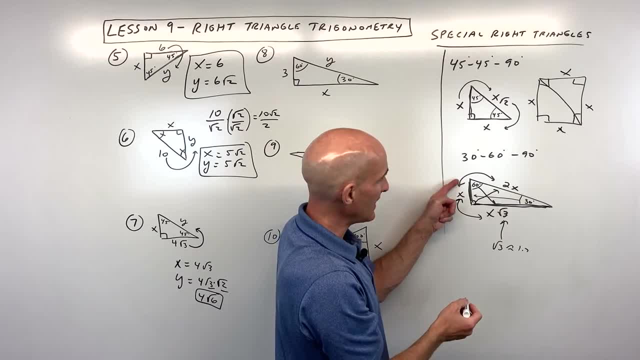 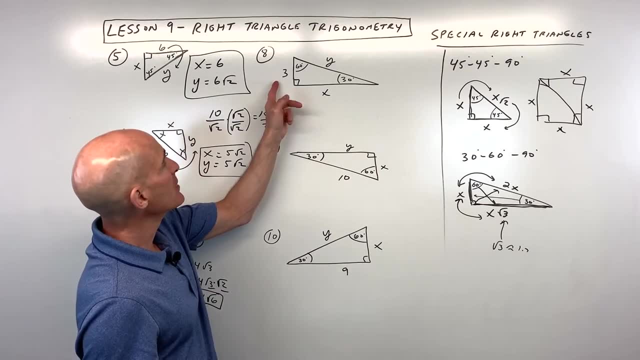 Divide by the square root of 3 to get to the short leg and then double to get the hypotenuse. Sometimes when you divide by square root of 3 you have to rationalize because you don't want that radical in the denominator. So for number 8, here, what do you think we should do? for this one, They're giving us the one across in the 30 degree angle. 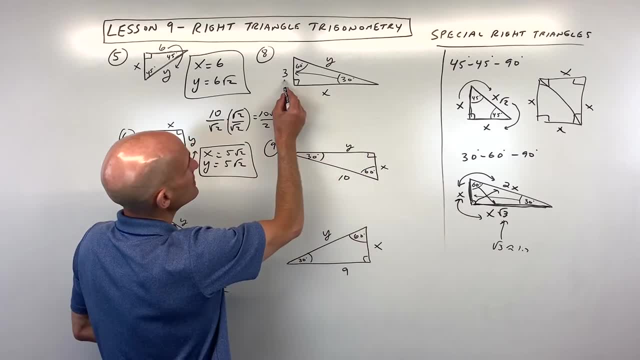 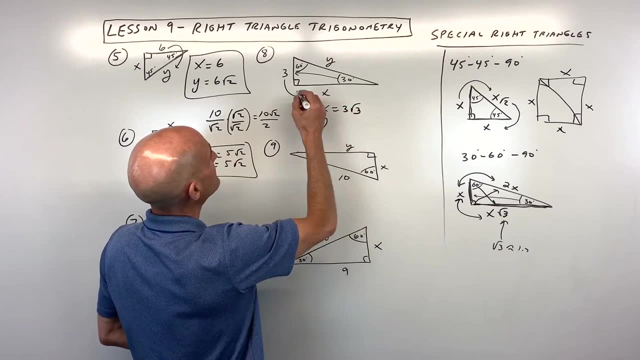 That's our short leg, That's this one here, X. so to get the to this longer leg we have to multiply by the square root of 3. so we have X equals 3 root 3, and To get to the hypotenuse we have to double that shorter leg. 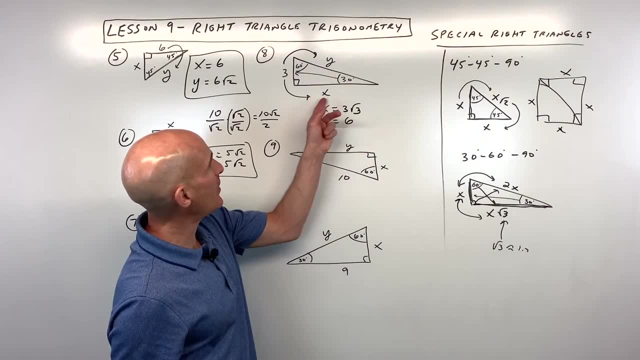 So that's 6. now sometimes students get a little bit confused because see how I labeled this X, and here in this diagram I was showing you that this is X. So just think the one across from the 30 short leg Multiplied by root 3 to get the longer leg, or double to get the hypotenuse. Let's look at number 9. number 9 is a little bit. 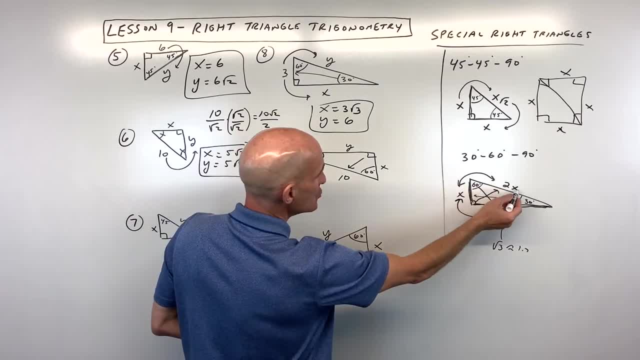 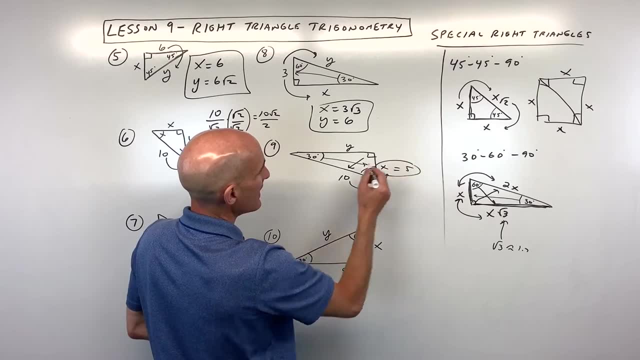 Different because they're giving us the hypotenuse. This is the 2x side. to get back to that shorter leg, the one that's across from the 30, I have to divide by 2. so here you can see: X equals 5 To get from the short leg to the longer leg, the one across from the 60 degree angle. 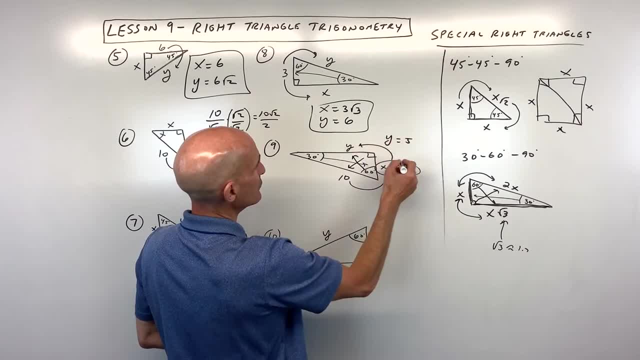 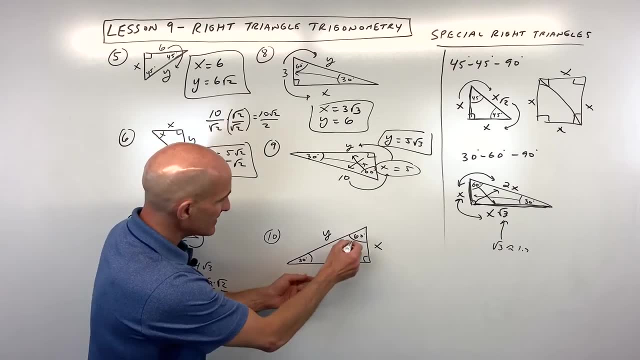 We just have to multiply by the square root of 3, so Y is equal to 5 Times the square root of 3. and for number 10- This is the toughest one that I was talking about- they're giving us the longer leg, the one across from the 60 degree angle. 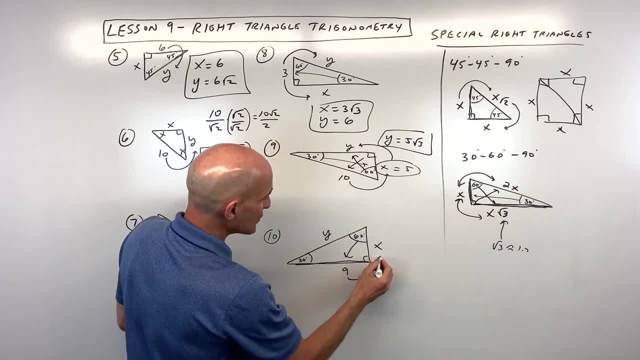 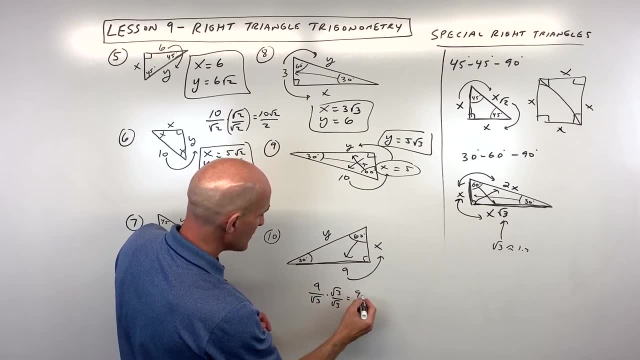 This is our X root 3 side. so to get back to that Longer leg we have to divide by the square root of 3. Of course we don't want that squared in the denominator, So we have to rationalize so that comes out to 9, square root of 3 over square root of 9. 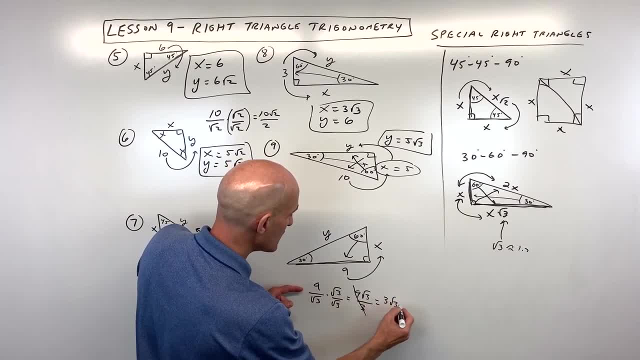 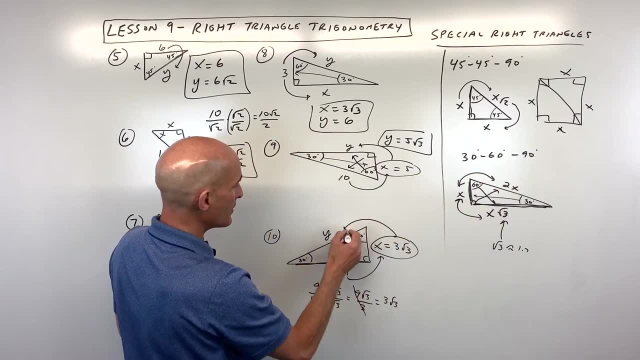 Which is 3, and here the 9 and the 3 can reduce To 3 root 3. so this is 3 root 3 for X, And then, once you have that short leg, you can double it to get the hypotenuse. Y is going to be equal to 6 times the square root of 3. 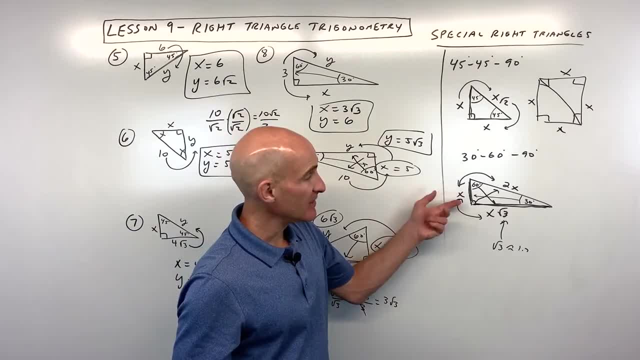 So the main thing is, if you can get to that short leg, then you're, it's easy. So if they give you this one divide by root, 3? They give you this one divide by 2. once you have the short leg, It's easy. 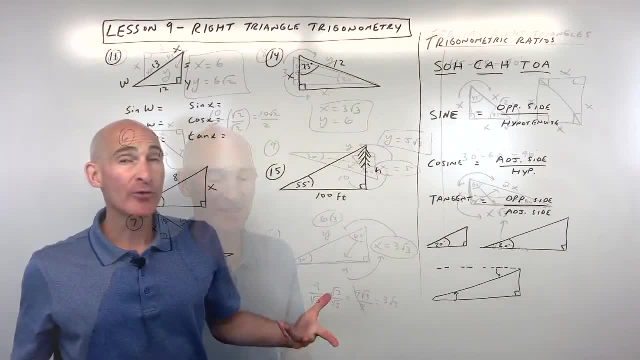 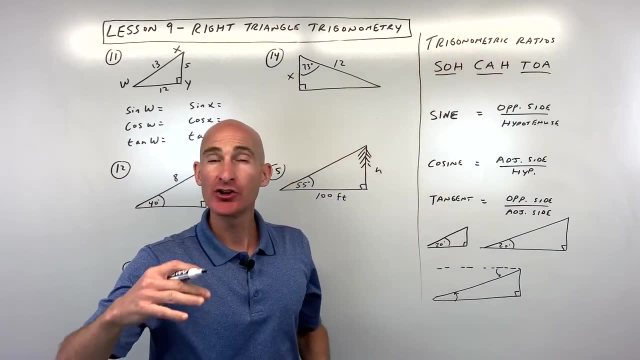 You can just multiply by root 3 or double to get the hypotenuse. Okay, Now we're going to talk about trigonometric ratios. What are trigonometric ratios? Well, ratios when you're comparing two quantities, like in a fraction form generally, and we talk about 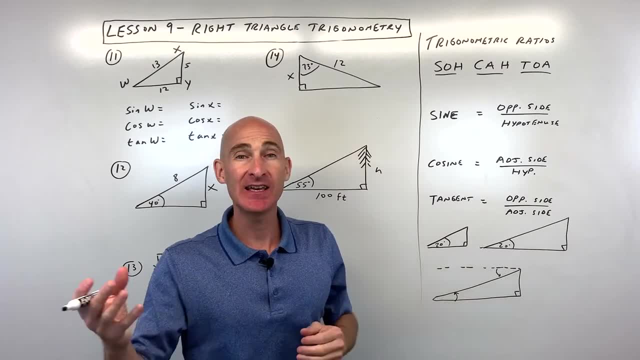 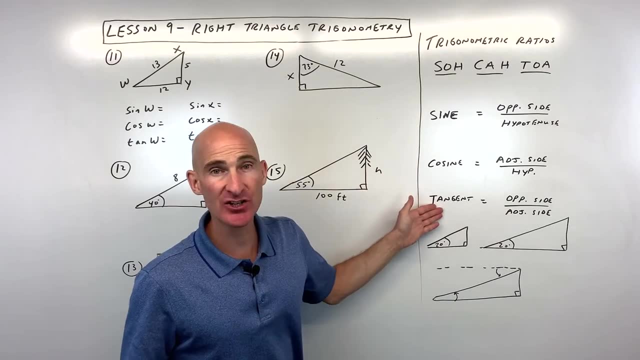 Trigonometric ratios. we're talking about the ratios of the side lengths in a triangle, and there's three important trig ratios We're going to talk about now, and that's the sine ratio, the cosine ratio and the tangent ratio. you've probably seen this on your 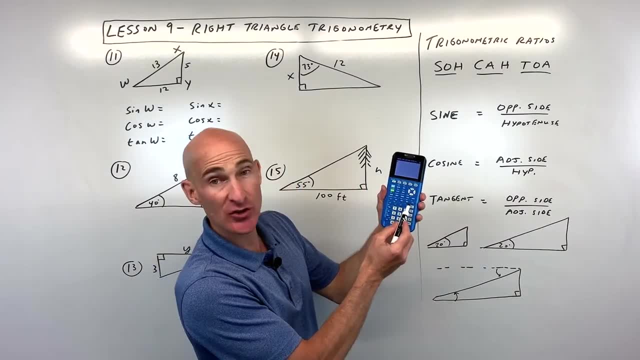 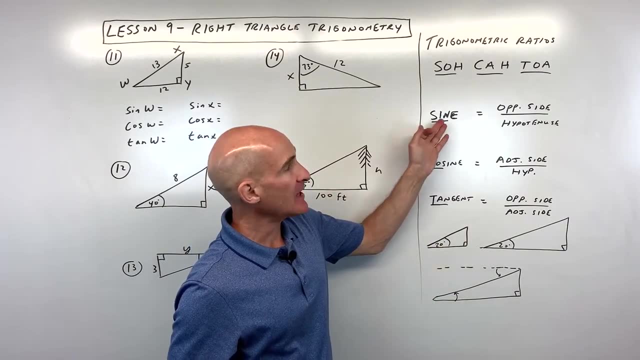 Calculator before you. it looks like SIN, COS or TAN. They just use those first three letters as an abbreviation and the sine Okay is the ratio of the opposite side over the hypotenuse. So, for example, if I have a triangle like, say, this one right here: 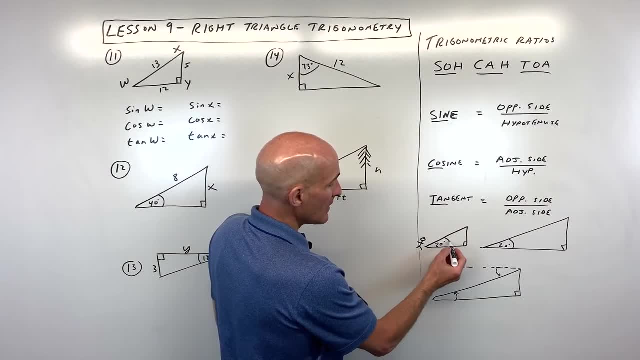 What you want to do is you want to position yourself at the angle. The opposite side is the one that's across from that angle. The hypotenuse is the one that's across from the right angle. So that's the ratio of this side over this side. 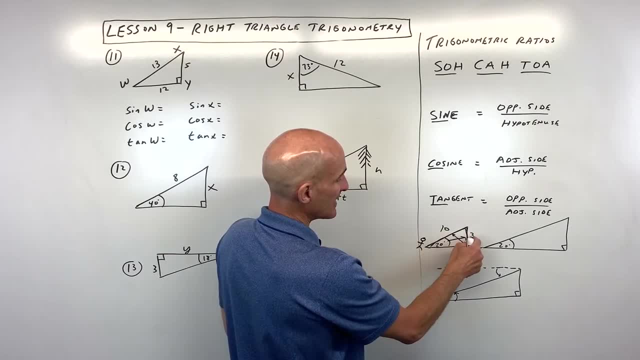 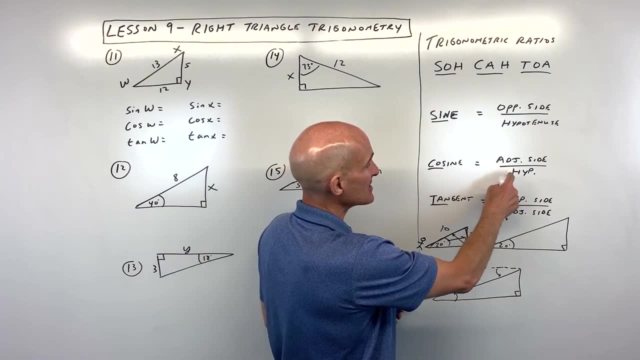 So, for example, say this was 3 and this was 10, we'd say the sine is 3 over 10. now the cosine- Okay, COS is the adjacent side over the hypotenuse. now we talk about adjacent, we mean next to. so if you're here at this angle, 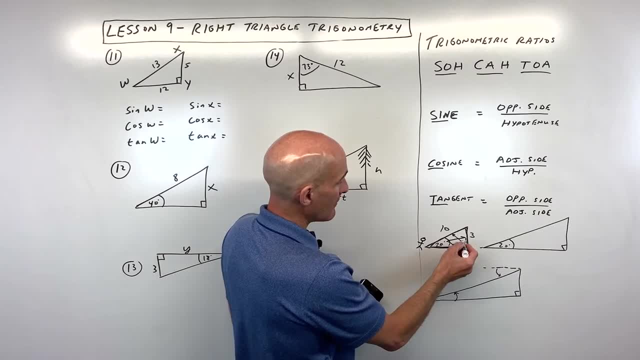 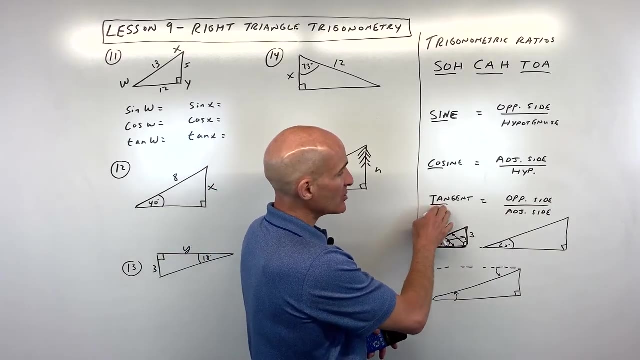 Adjacent would be the side next to that angle, Divided by the hypotenuse, That's the one across from the right angle. Now, sometimes students will say, Mario, Isn't 10 adjacent to this angle here? Well, that's True, but you want the other one, not the hypotenuse, not the one across from the right angle, and then the tangent ratio. 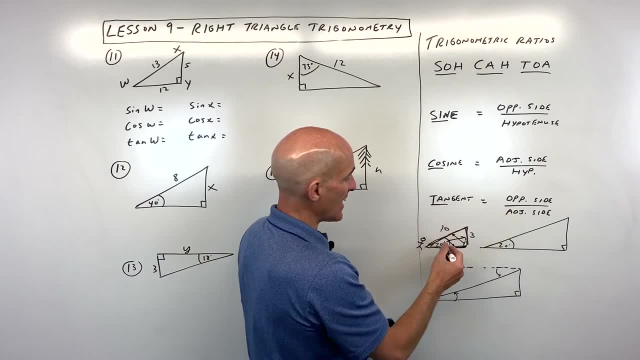 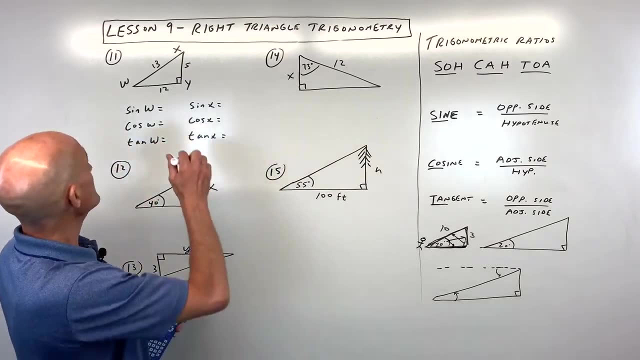 It's the ratio of the opposite side over the adjacent side, So the one across divided by the one next to. let's look at some examples. I'll show you how that works first. So say for number 11, let's say you want to find the sine of. 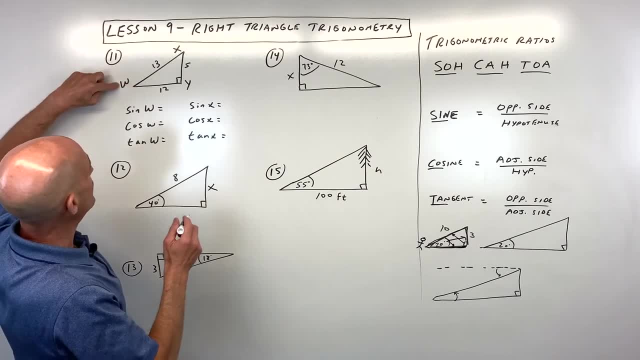 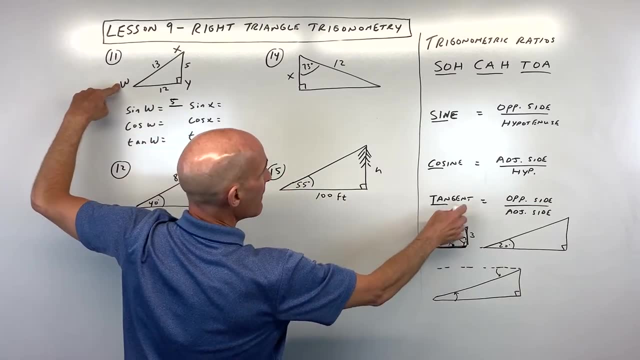 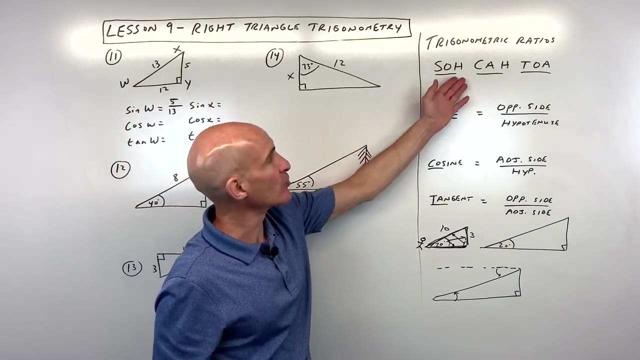 W. so what you do is you'd pretend like you're standing right here at this angle and you say: sine is the opposite side. That's 5 over the Hypotenuse right, which is 13. now, one thing I didn't mention is there's an acronym that students learn when they're doing this. 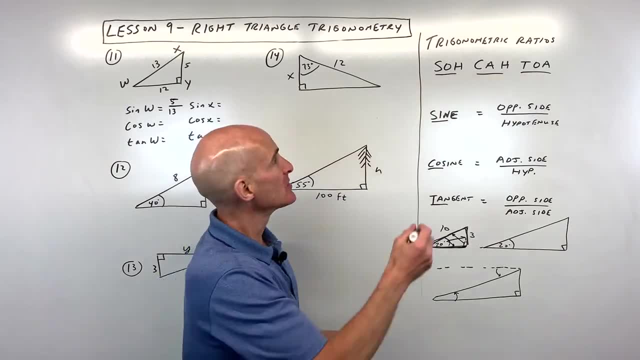 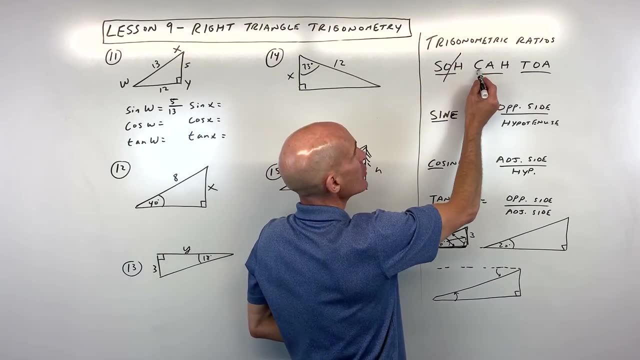 And that's the SOH, CAH, TOA acronym. So what it stands for is: sine is the opposite, over the hypotenuse. So you the second, divided by the third letter. Cosine is the adjacent divided by the hypotenuse and tangent is the opposite divided by the adjacent. 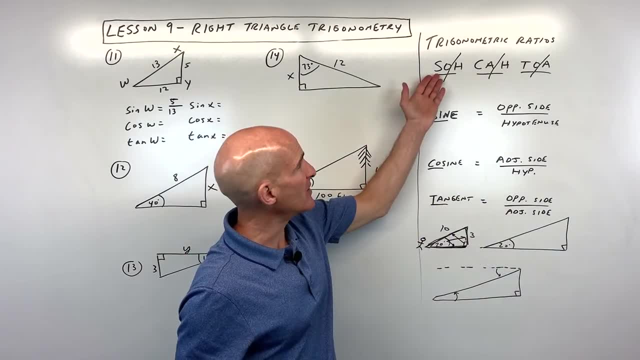 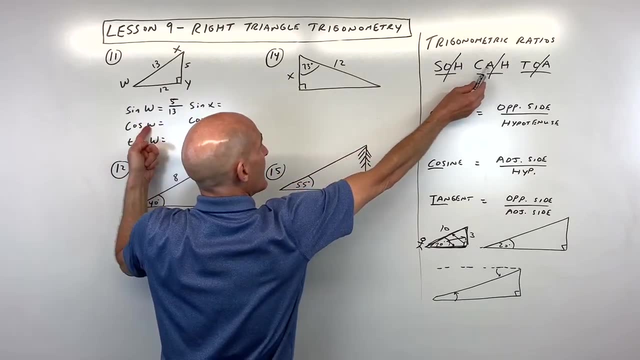 So it's always the second letter divided by the third letter and you can just memorize SOH CAH TOA. So if I'm doing the cosine now, we could say the cosine of angle W, that's a over H. So the adjacent which is next to that's 12 over hypotenuse, which is 13. 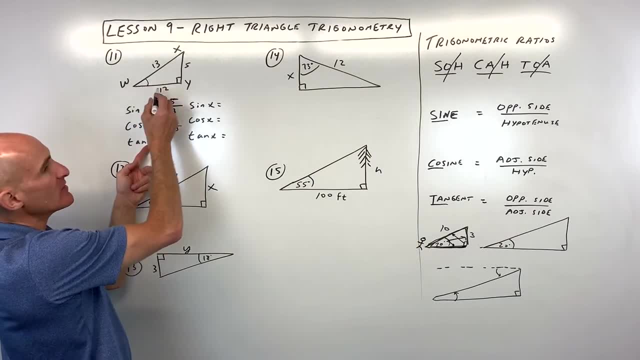 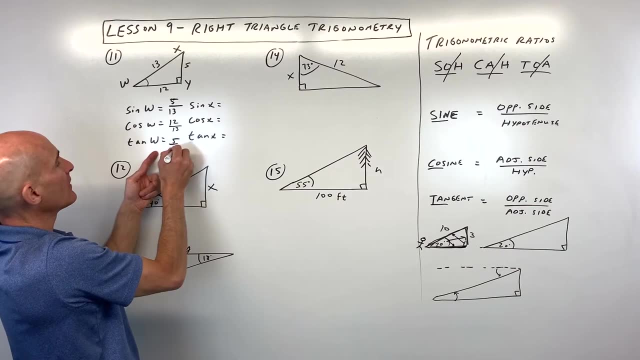 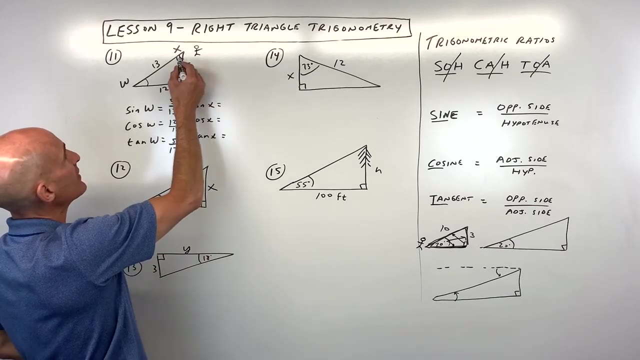 And then the tangent of angle W is going to be TOA, That's the opposite over adjacent. So the opposite, 5 over adjacent, which is 12. Okay Now, if we move to angle X, now we're gonna position ourselves, pretend like we're standing here at angle X. the sine of angle X would be: 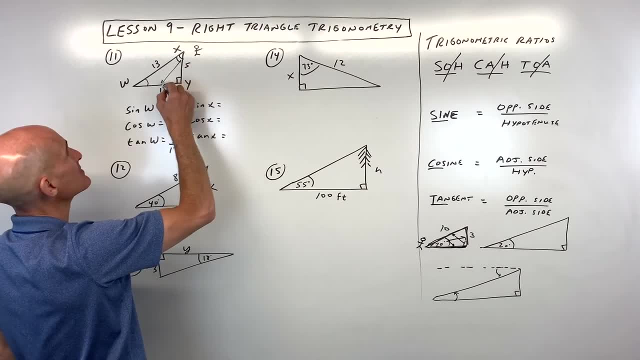 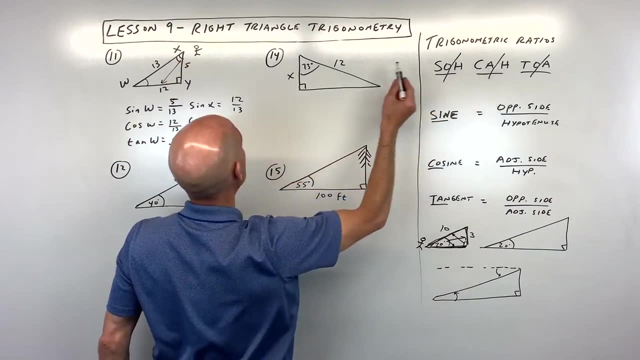 SOH. so that's opposite over hypotenuse. That'd be opposite 12 over hypotenuse 13. The cosine of X would be CAH. This is adjacent over hypotenuse. That would be adjacent which is next to 5. 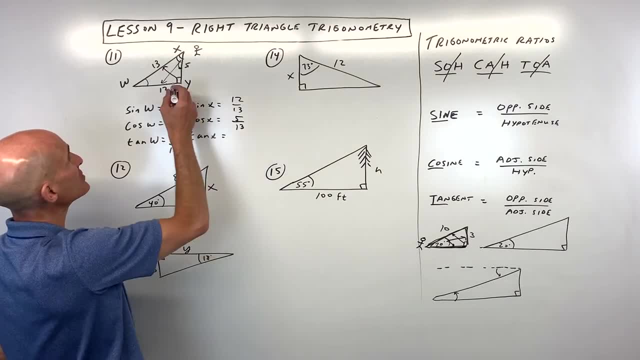 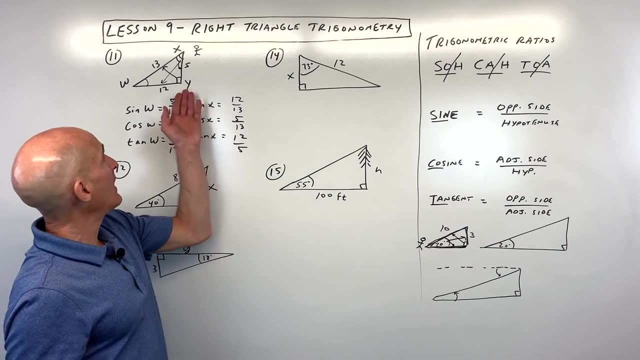 over hypotenuse, which is 13, And tangent of angle X. that's going to be opposite over adjacent, That's the TOA. So that's going to be 12 over 5. Now, what about angle Y? Well, angle Y is the right angle. 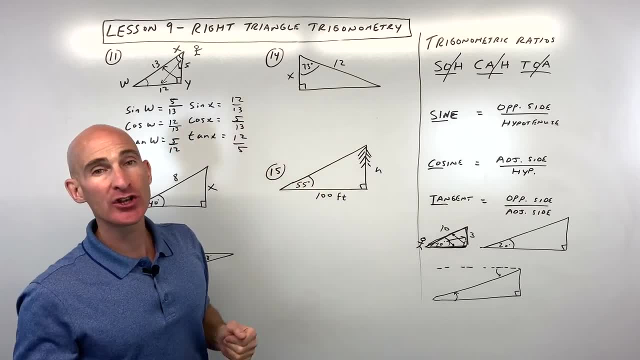 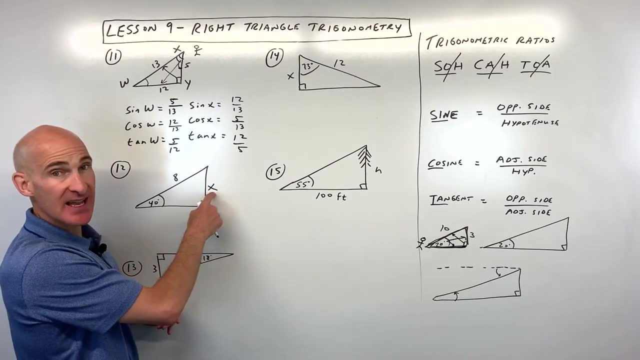 You just use the trigonometric ratios with either of the two acute angles, not the right angle. Okay, so for number 12, we're gonna get into how do we solve for like a missing side length if we know this angle and another side, and we're gonna use 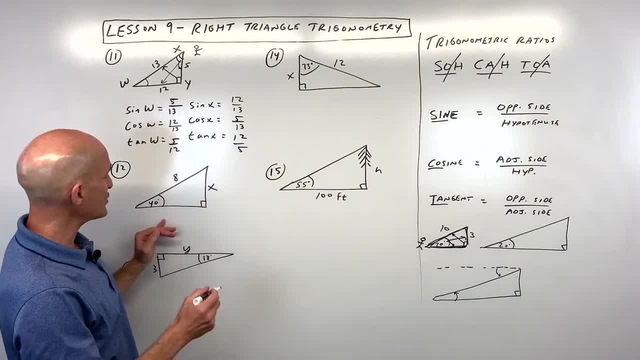 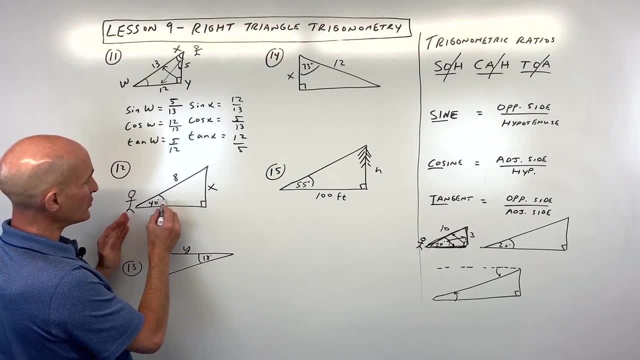 our trigonometry here, our trig ratio, sine cosine and tangent. What you always want to do, though, is you want to position yourself at the angle, and you say: okay, What trig function ties together this angle? 40 degrees, the opposite side and the hypotenuse? Okay, so, opposite hypotenuse. 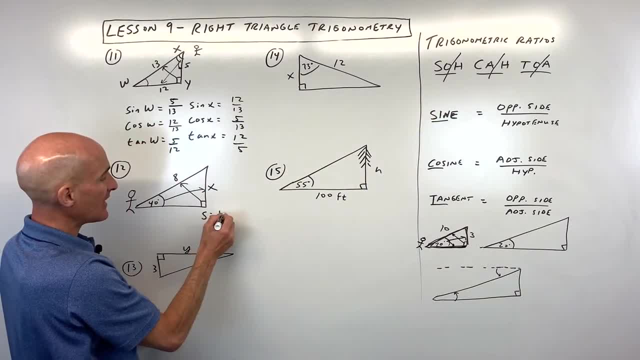 O and H. that's the sine. So we would say the sine is the sine of the angle. sine of 40 degrees equals the ratio of the opposite side, x over the hypotenuse 8.. Now all we have to do is multiply both sides by 8 to get x by itself and x equals 8 times the. 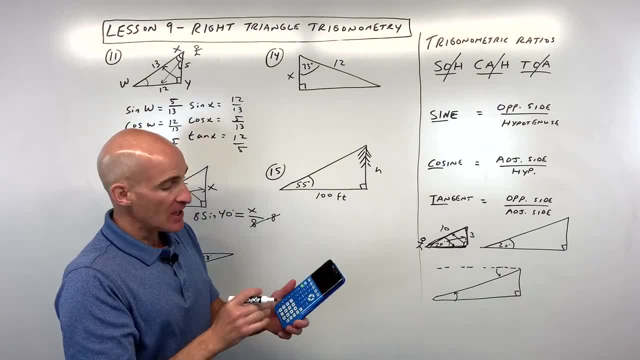 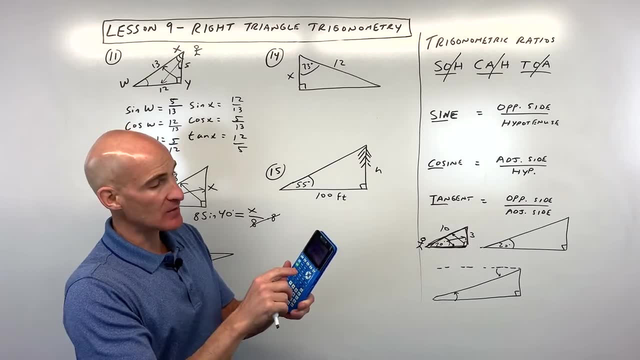 sine of 40. Now you're going to want to go to your calculator. you want to check your mode. so somewhere, depending on what calculator you're using, you're going to go to mode and you want to make sure you're in degrees, not radians. okay, so then you can exit out of there and we're going to go 8 times. 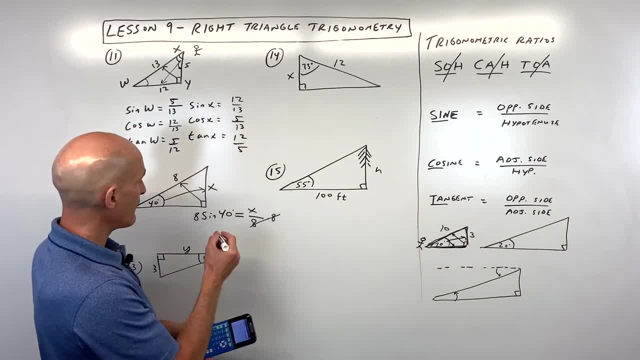 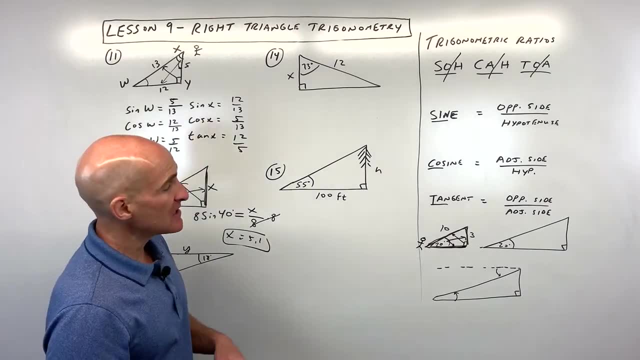 the sine of 40 degrees and you should be getting 5.1. so that's going to be the length of this side right here. okay, so you see the application, see whether you're working with a little triangle, like see this little triangle with a 20 degree angle, or if you're working with this larger triangle here. 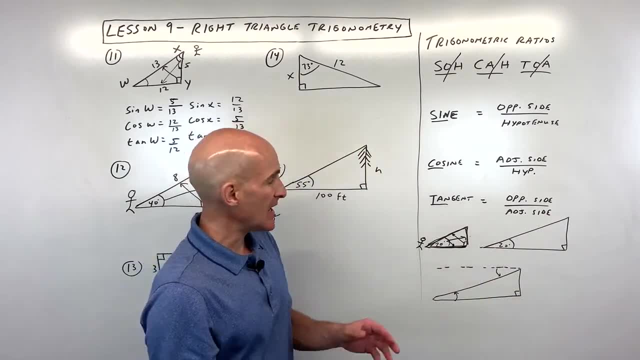 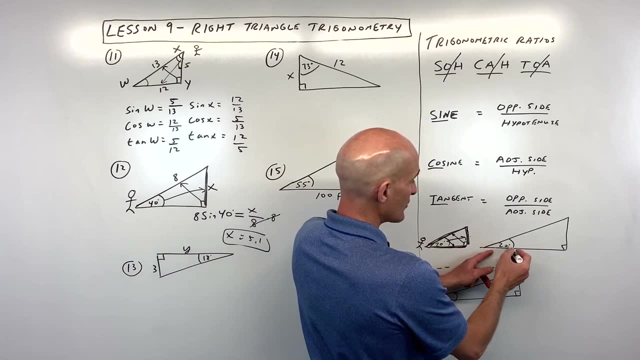 with a 20 degree angle, the ratio of the sides are going to be the same, like if i do the sine of in this triangle. i would do opposite over hypotenuse. if i do sine of this triangle here, this sine of this angle, it's going to be the ratio of. 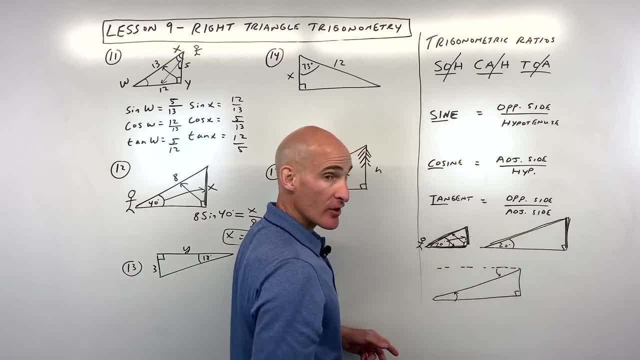 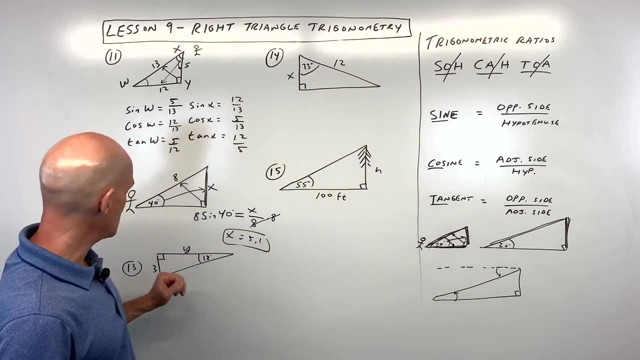 the opposite side over the hypotenuse. even though this is bigger, the ratio of this side over this side is going to be the same. okay, so that's where it has wide ranging applications. so let's look at for number 13 now. we want to find this missing side. right, we know, this angle is 18 degrees. we 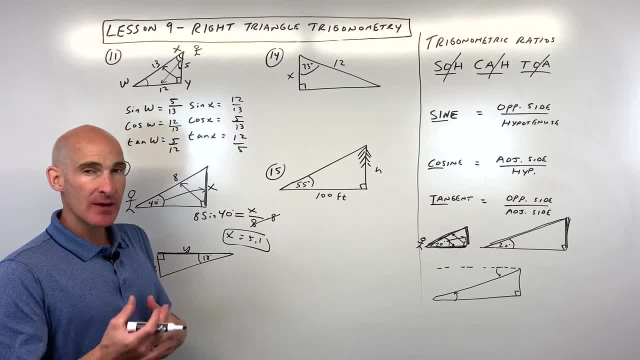 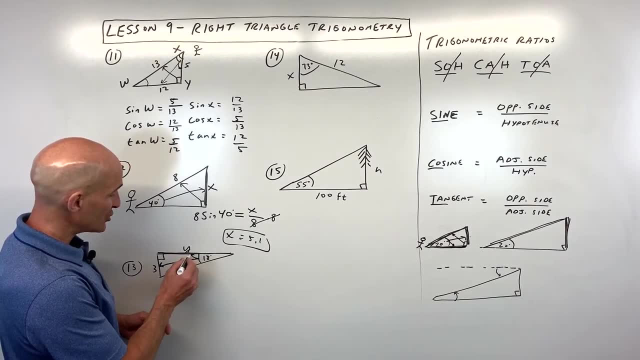 know this is 3, we know this is y. we need to set up some type of a, an equation that relates 18 degrees, 3 and y. so what trig function ties together opposite and adjacent? opposite and adjacent, that's toa, that's tangent. so we say the tangent of 18 degrees equals the ratio of the opposite. 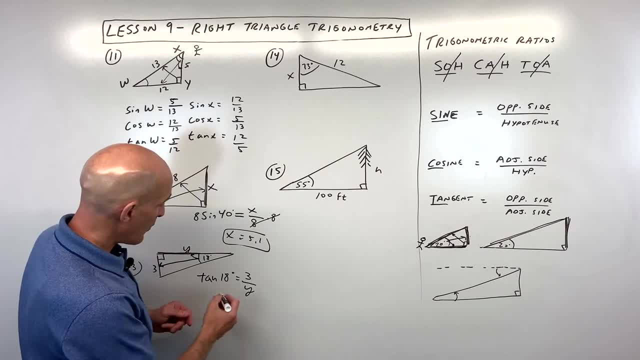 side 3 over the hypotenuse y. now what we can do is we can think of anything. divided by one is it's, you know, it's going to be itself. we can cross multiply, so that's going to be y times. the tangent of 18 equals 3 times 1, which is 3. so i'm just cross multiplying on the diagonal, and if i divide, 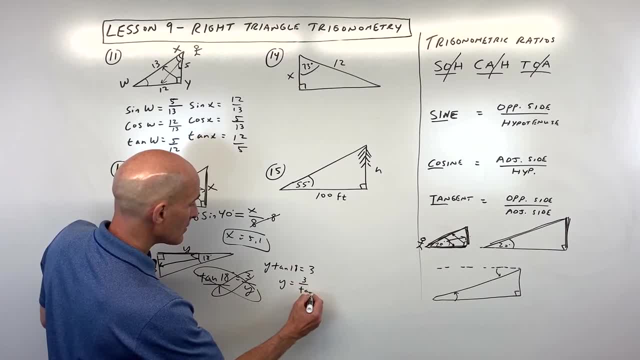 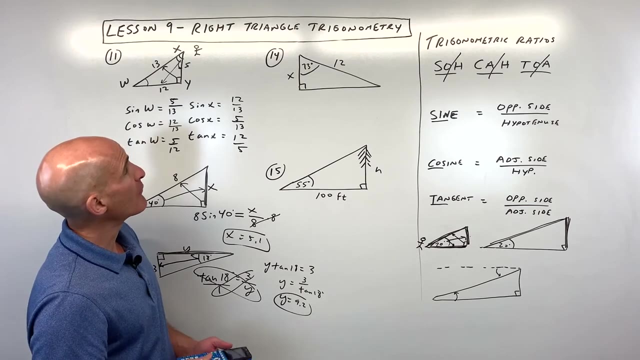 both sides by tangent of 18.. let's see what that comes out to on the calculator. so we have 3 divided by tangent of 18.. i'm getting 9.2. i'm just rounding a little bit here. so that's going to be this missing length of that side. okay, how about for number 14? what do? 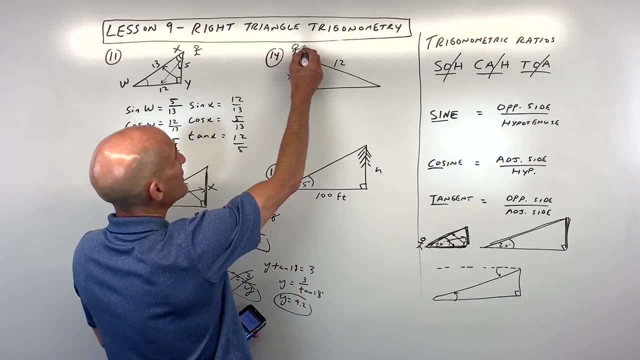 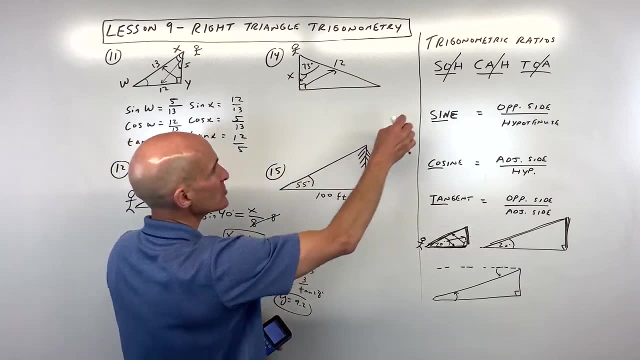 you think for this one. well, again, you want to position yourself at the angle. okay, so this is our perspective. we've got the adjacent and the hypotenuse. so adjacent, hypotenuse, that's ka, that's cosine. so we say the cosine of the angle, it's always cosine. 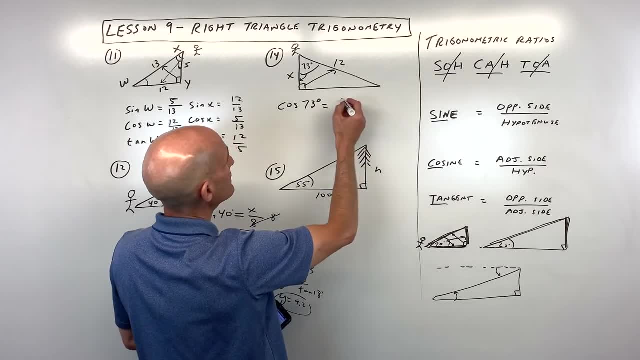 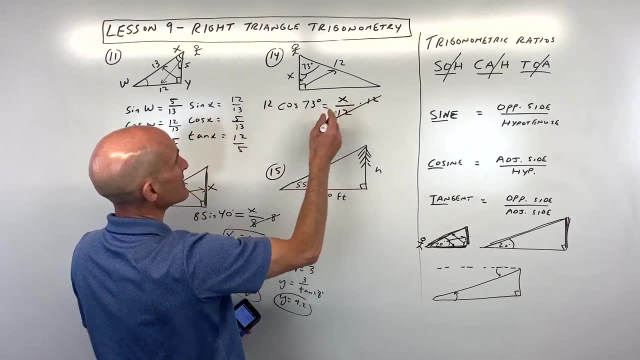 of the angle or sine of the angle. tangent. the angle equals the ratio of the side, so in this case the adjacent over hypotenuse. multiply both sides by 12 to get x by itself. and let's go to our calculator: 12 cosine of 73, i'm getting 3.5 approximately. okay, so number 15. now what i? 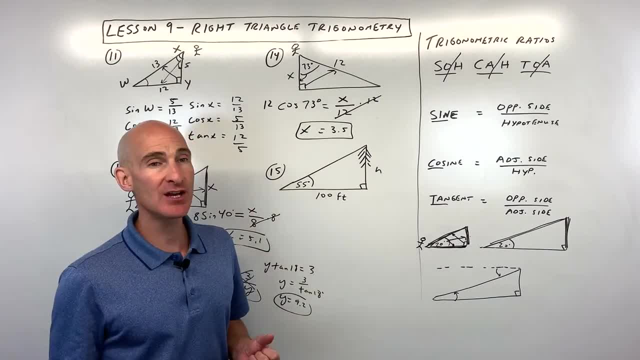 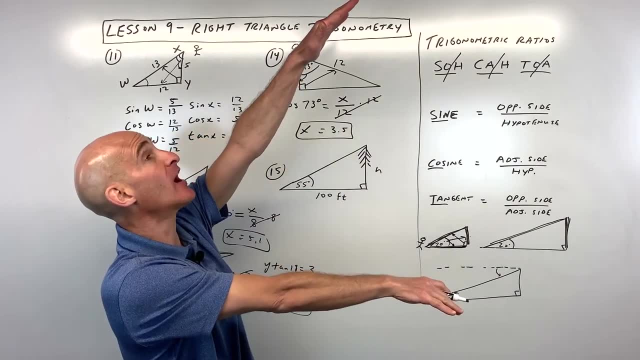 want to talk about here is some kind of real life applications. when you look at these triangles, there's something called angle of elevation, like if you were to elevate or look up, see this angle right here. that's angle of elevation, whereas if you look down from the horizontal, 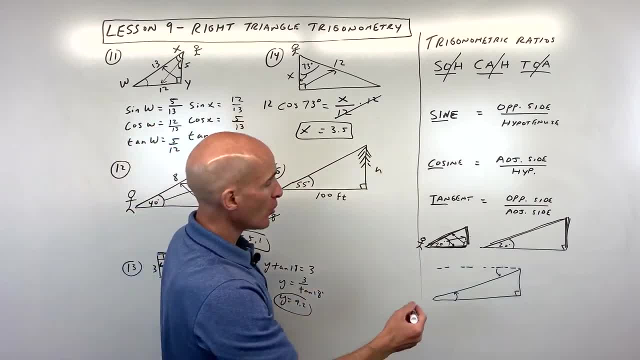 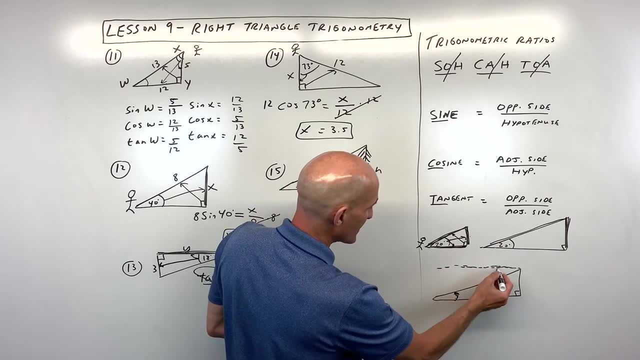 this angle here is going to be your angle of depression. so what you'll notice here- see in this diagram, if i go elevation, where here i have to kind of draw a dotted line- i'm going down from the horizontal, that's depression. but when you have parallel lines cut by a transversal, 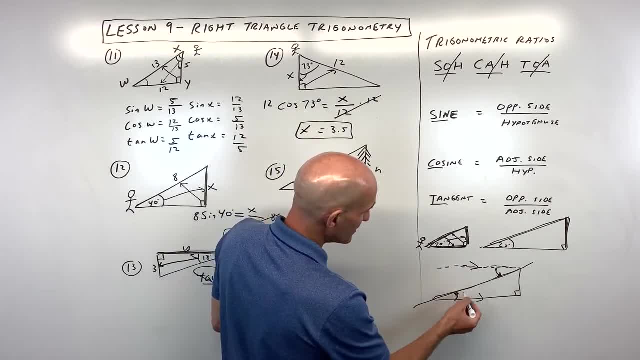 remember we talked about this earlier in the course. these are alternate interior angles. these are actually going to be congruent. sometimes students mistakenly think this is our angle of depression, but it's actually c on the outside. you can draw this as a rectangle. the opposite sides are going to be congruent and these alternate interior angles are going to be congruent. 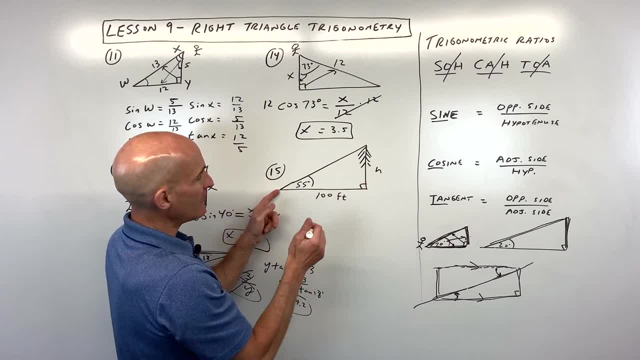 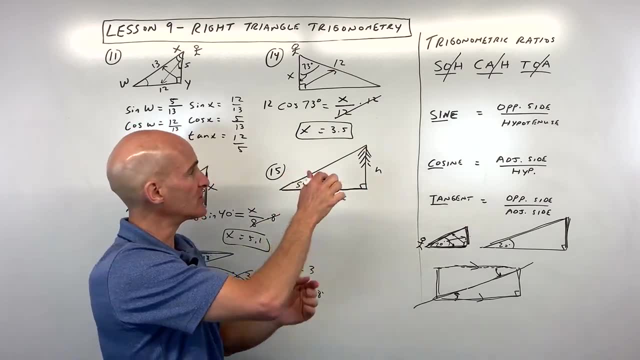 but for this one, like, say, if you wanted to find the height of a pine tree, right, and you walk back like say 100 feet from the pine tree, and then you estimate or use a protractor, you find out that angle to the top of the tree- let's just say it's 55 degrees- how can we find the? 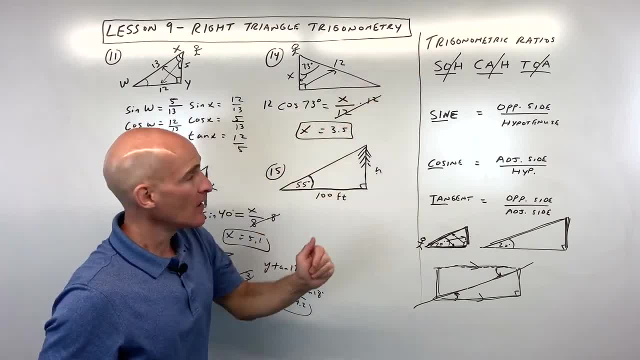 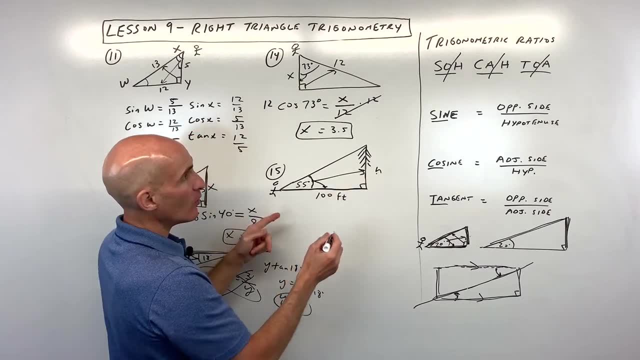 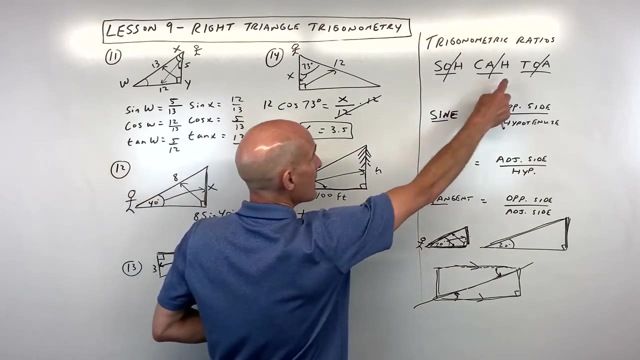 height of that tree, using triangles or trigonometry. well, let's see what trig function ties together opposite and adjacent. well, opposite and adjacent, that's toa, that's tangent right. so we have tangent of the angle. tangent of 55 equals the opposite of adjacent, second over. 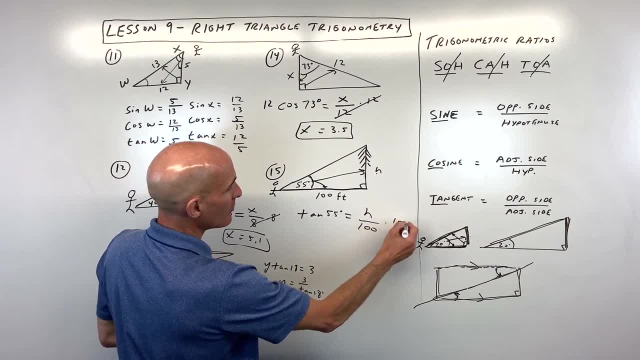 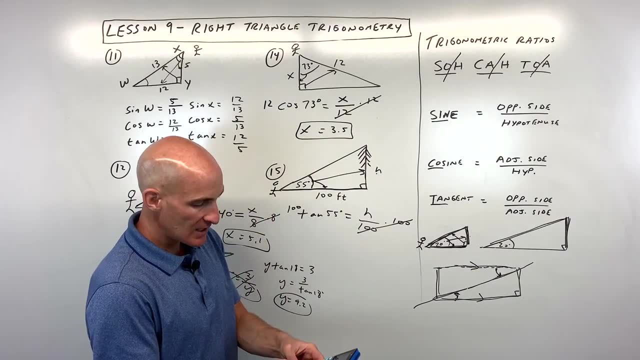 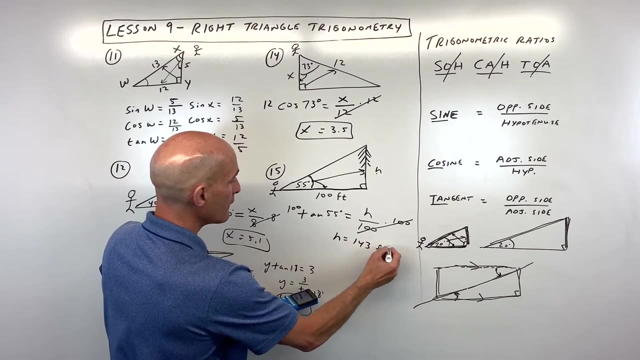 third, that's h over 100. that's our equation. now we just have to multiply both sides by a hundred to get h, the height by itself. so let's go to the calculator. so let's just take the angle tangent of 55, i'm getting 142.8. let's just round it to about 143. 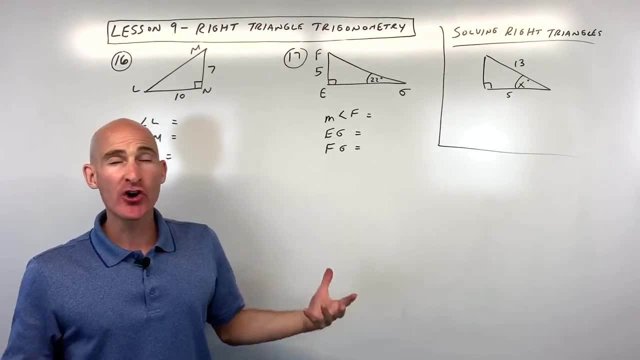 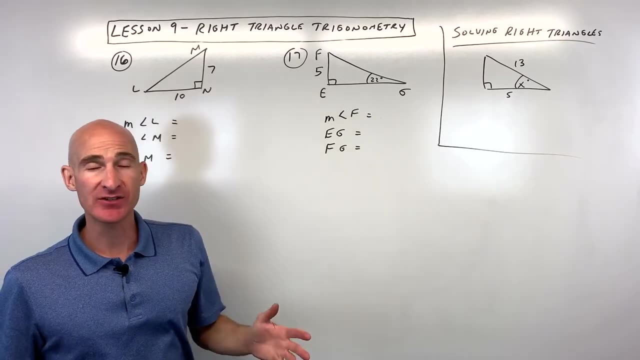 feet. that's how tall that pine tree is. okay, now we're going to talk about solving right triangles. what does that mean to solve right triangle? well, it means you want to find all the angles and all the sides. so it's really six pieces of information, three angles, three sides. but they're going to give. 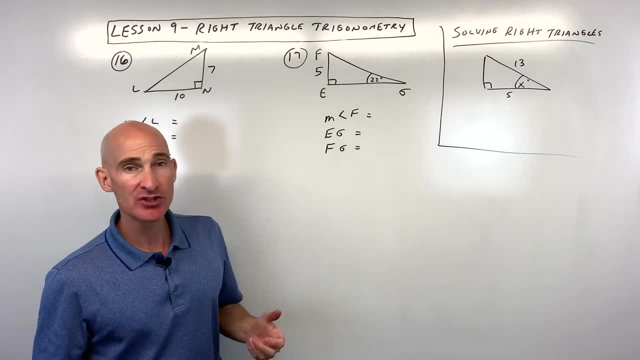 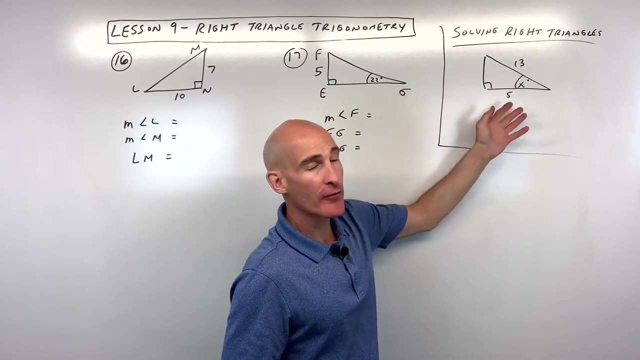 you three pieces of information, so you'll be able to just have to solve for the missing three. but what i want to show you in this particular part of the video is that you can find the angles of the part of this lesson is. we've talked about how to solve for the missing side. How do 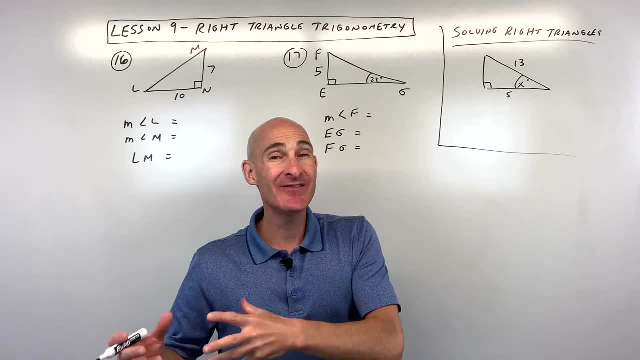 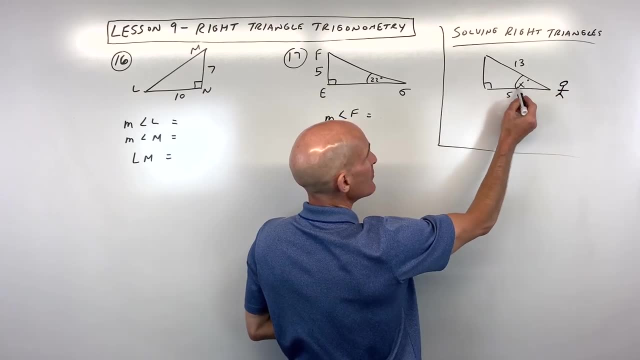 you solve for the missing angle. And that's where inverse trigonometric functions come into play. So for example, like we've been doing, we position ourselves at the angle, Say we want to solve for angle x. We say what trig function ties together the adjacent side. 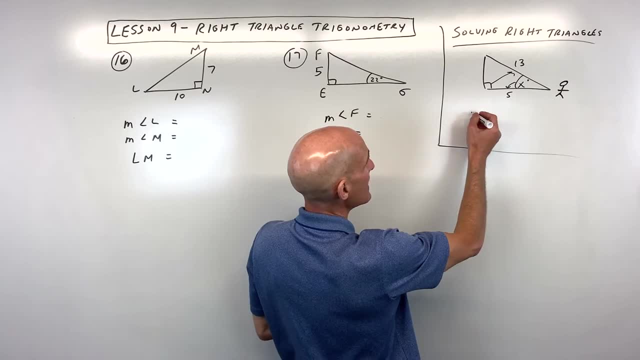 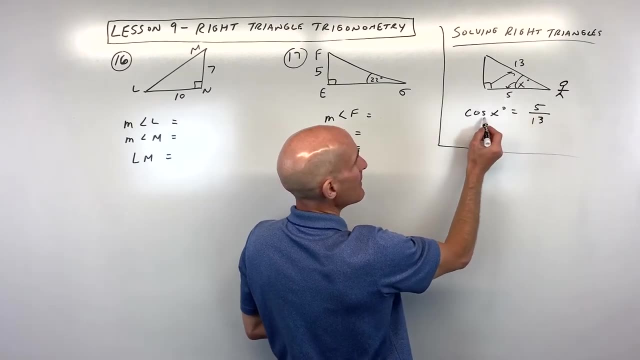 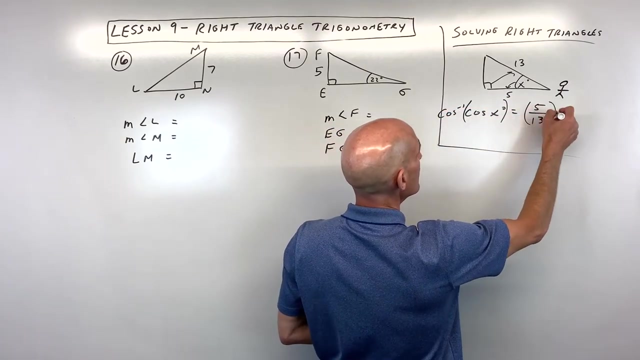 and the hypotenuse. Well, that's cosine, Remember cah c-a-h. So we say cosine of x degrees equals adjacent over hypotenuse, But we want to get that x by itself. So what we do is we take the cosine inverse of both sides of the equation. So really what we have here. 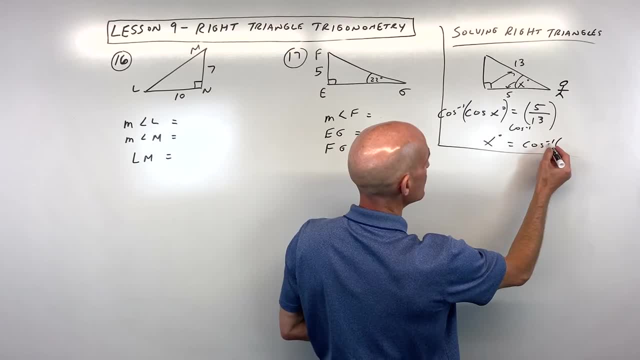 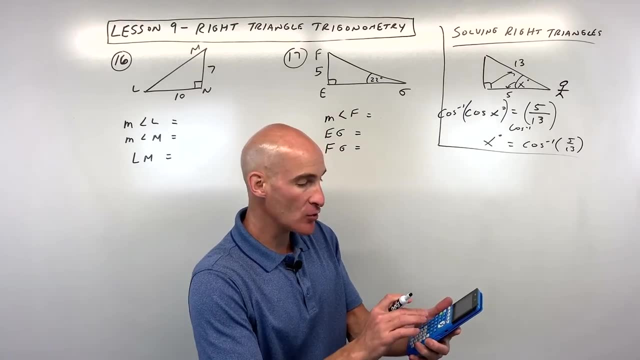 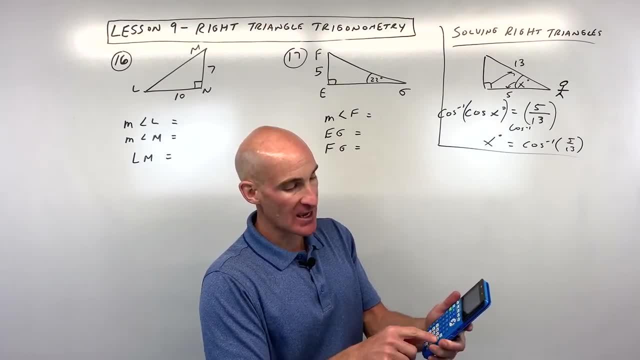 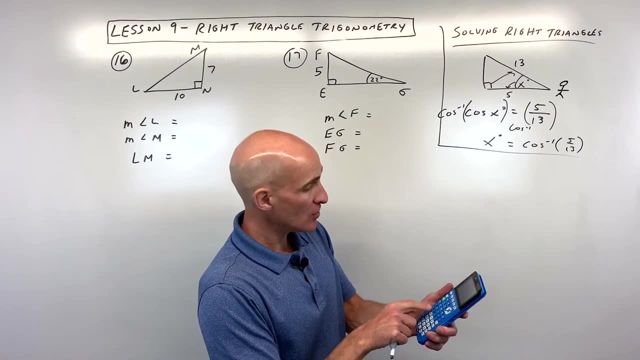 minus one tangent minus one, that means the inverse, And they should be right above the sine cosine and tangent, So you should be able to access that, depending on what type of calculator you have. We're going to go to second cosine, that's our cosine inverse. 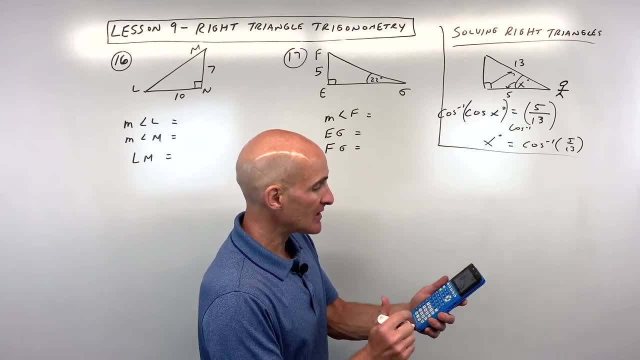 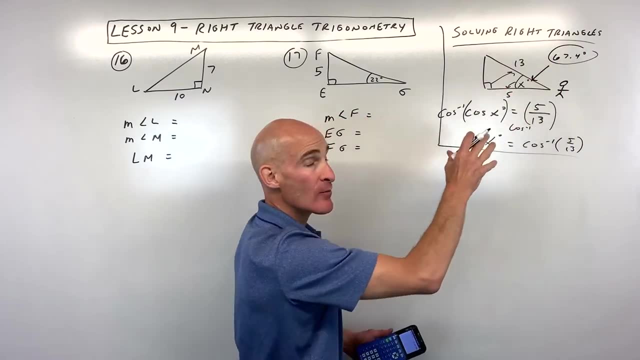 of five divided by thirteen, And I'm getting sixty-seven point four degrees. So that's how much that angle is right there. So just remember, when you're solving for the angles, you're going to have to use the inverse trig functions. If you know the angle, you're just 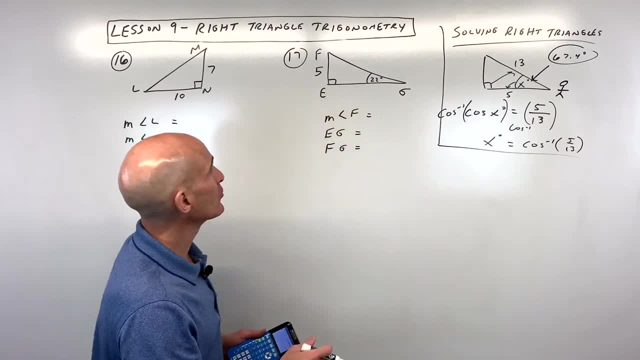 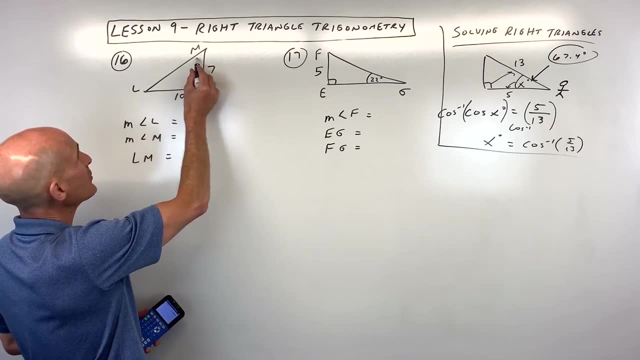 going to use the regular sine cosine and tangent. So we're going to go through a couple different problems You can practice here. Let's say, for number sixteen, I want to find these two angles as well as this missing side. So they 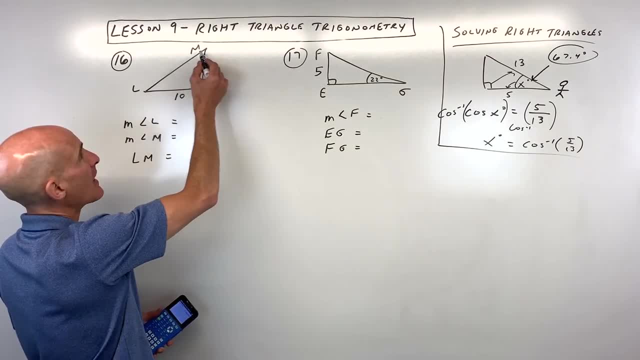 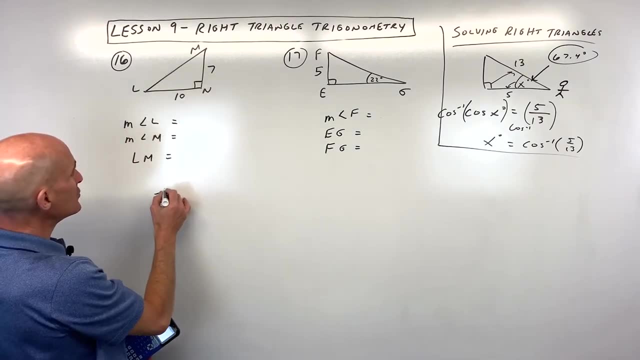 give us these two side lengths. Let's go ahead and find this hypotenuse first. Well, we talked about at the beginning of this lesson Pythagorean Theorem. a squared plus b squared equals c squared. So let's go ahead and do that. We've got seven squared plus ten squared equals. 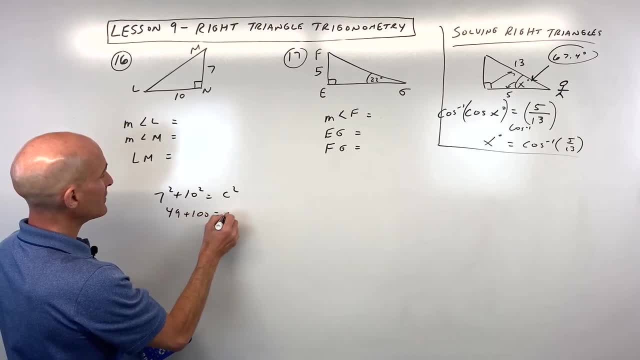 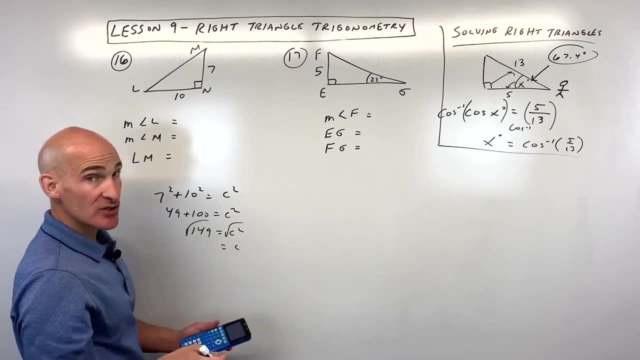 c squared. So forty-nine plus a hundred equals c squared. One hundred and forty-nine equals c squared. And if we take the square root of both sides, we can either leave it as a square root of one hundred and forty-nine or we can get 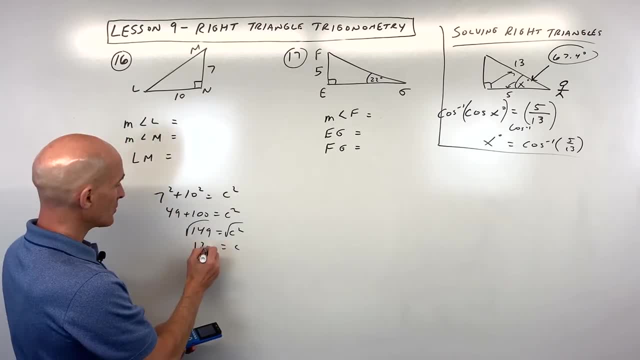 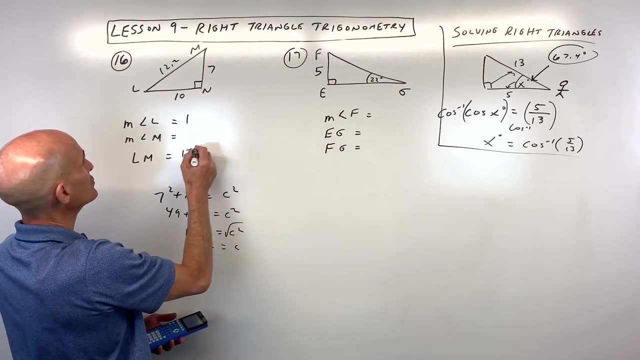 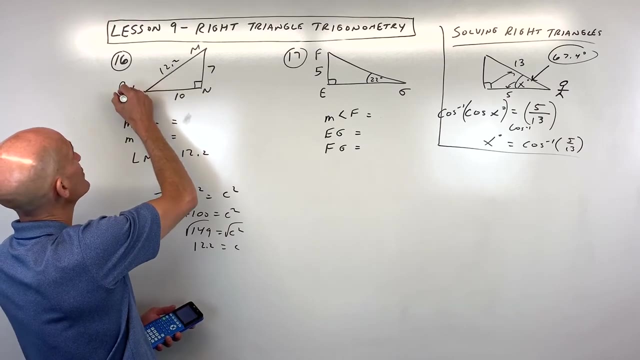 a decimal approximation. It's about twelve point two. Okay, so that was for side lm And that's twelve point two. Okay, now we have to solve for the angles. Which angle should we do first? How about we do angle l? We'll position ourselves here, And this is an important 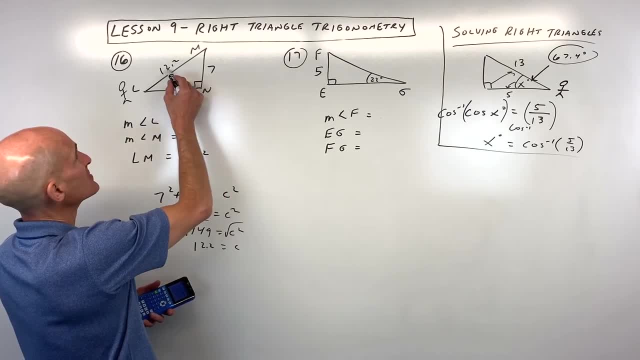 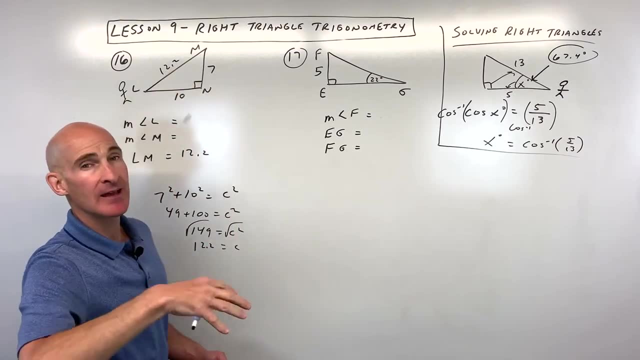 point. Do we use these two sides, Or do we use these two sides, Or do we use these two sides, Or should I use this hypotenuse? Well, I probably wouldn't use the hypotenuse, just because it's a rounded answer. So if I round and then I round again, my answer might be: 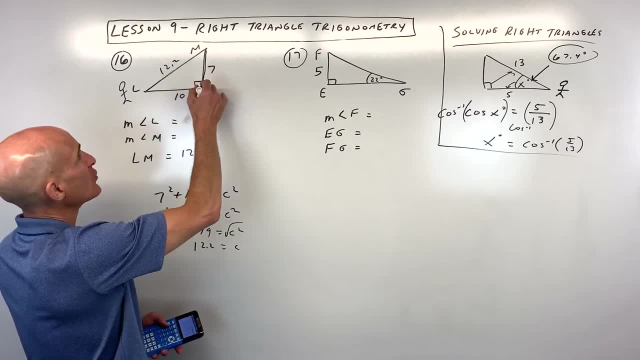 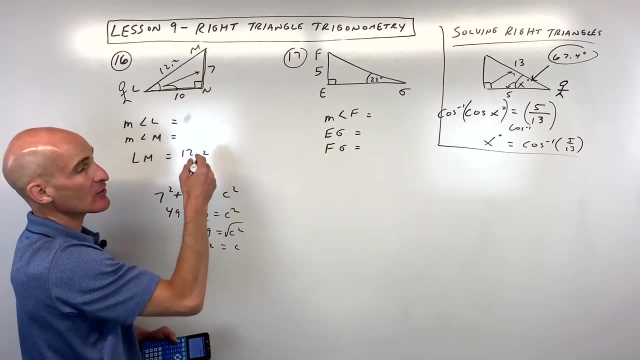 a little bit further off. So I try to go back to the original values if at all possible. So in this case it looks like to find angle l we could use the opposite side, the adjacent side, Remember the opposite. adjacent, that's TOA, that's tangent, So we can say the tangent. 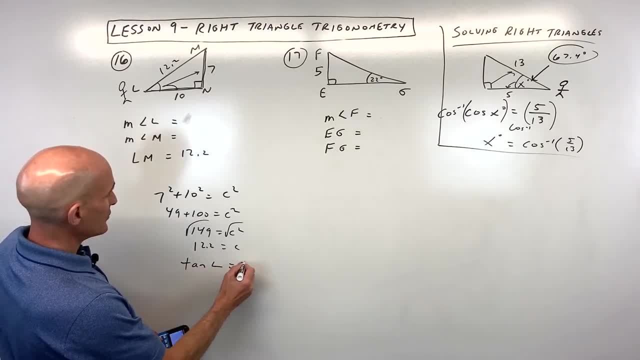 of angle l is equal to opposite only. So we're adjacent. Now remember, we're trying to solve for this angle l here. Whenever we solve for the angle, we have to do the inverse trig function. So what it's like doing it's. 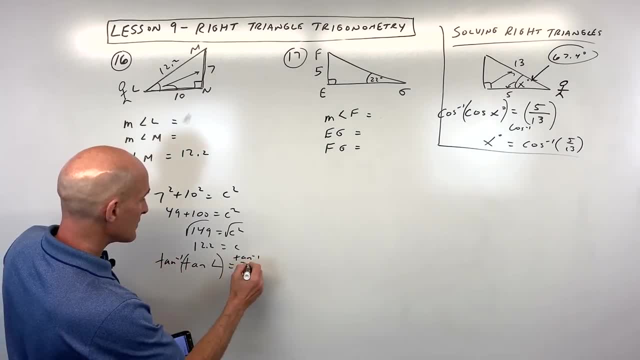 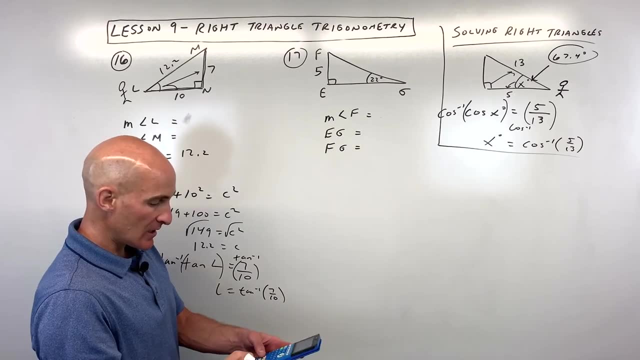 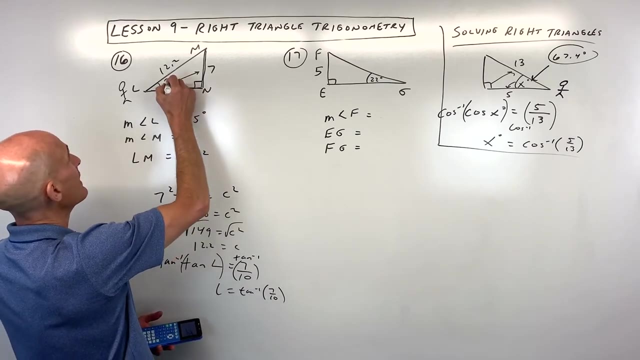 like taking the tan inverse of both sides. Okay, so you could say l equals the tangent inverse of seven tenths. So, going back to the calculator again, I'm getting about 35 degrees. So this is about 35 degrees. Now, if this angle is 35, this angle here has to. 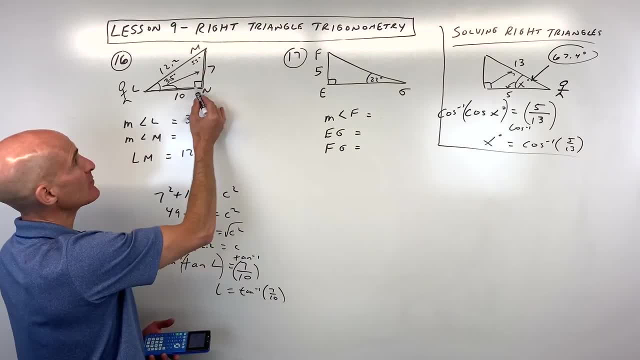 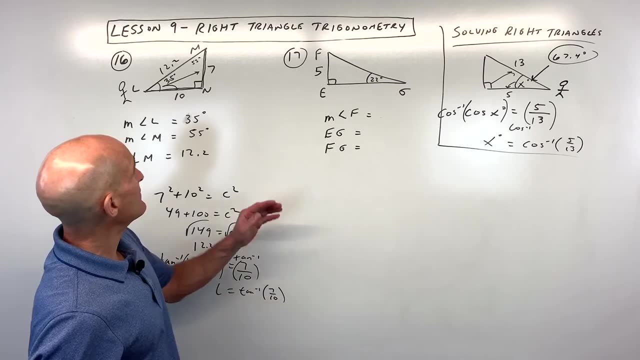 be 55.. because these two angles have to add up to 90, plus 90 gives us 180 degrees for the triangle angle measures, right. So now let's go to number 17,. a little bit different problem here. Here we have the angle, we have this side and we have the. 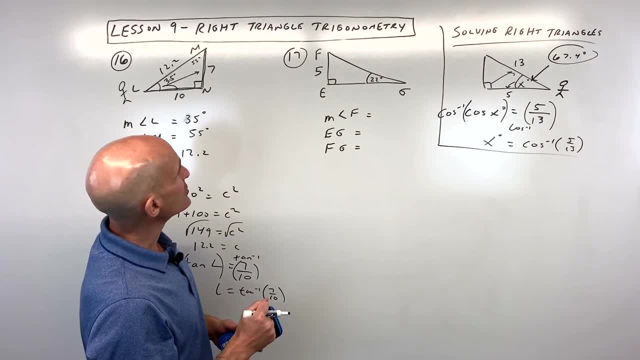 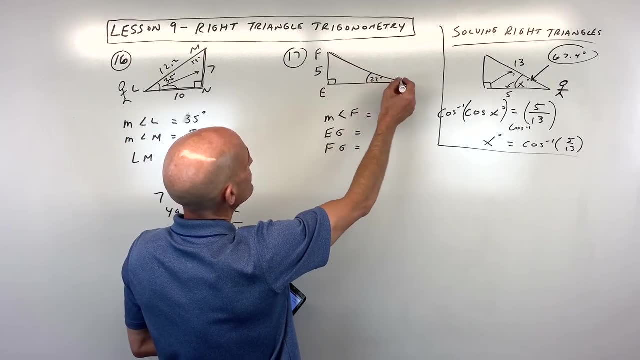 right angle. So what do you think we should solve for first? Well, it doesn't matter too much. Why don't we go ahead and solve for the hypotenuse here? So what trig function ties together opposite and hypotenuse? Well, that's. 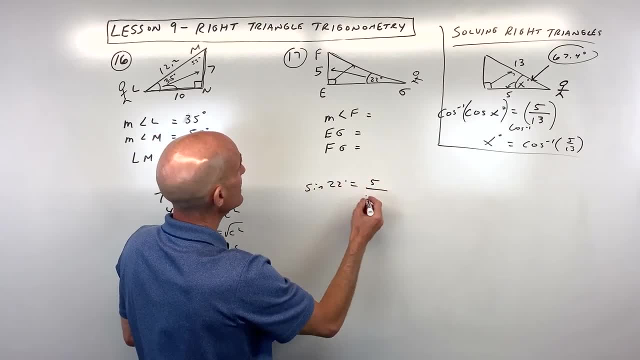 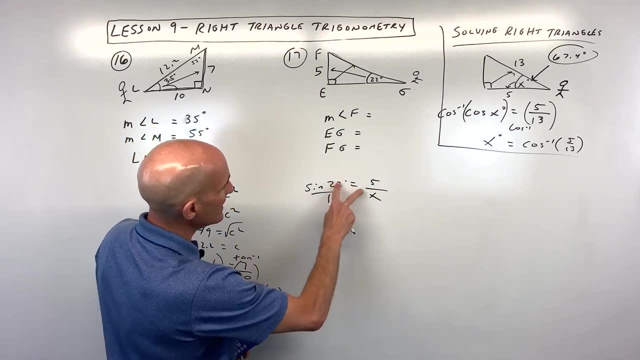 going to be the sine, So we see sine of 22 degrees, equals opposite over hypotenuse. so let's call that x. We can cross multiply. or there's a neat technique with proportions where you can interchange these on the diagonal, so that's the property of proportions. X over 1 is just going to be x, So we get 5. 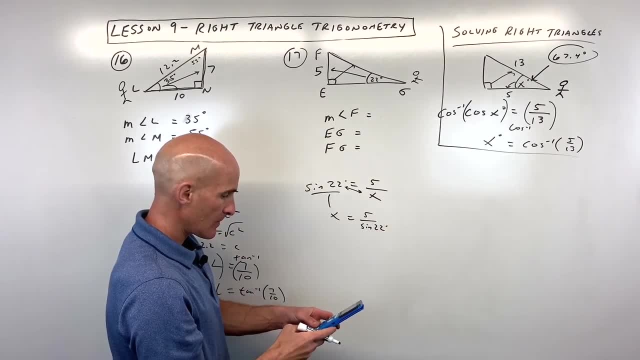 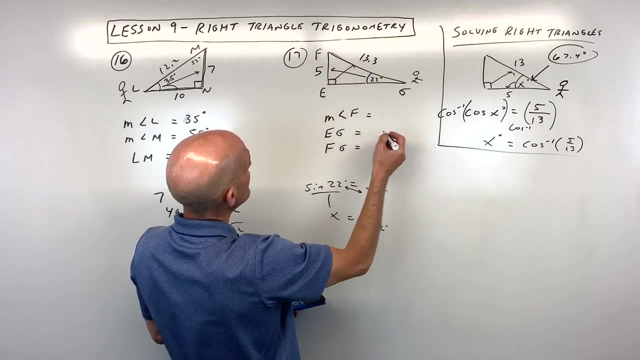 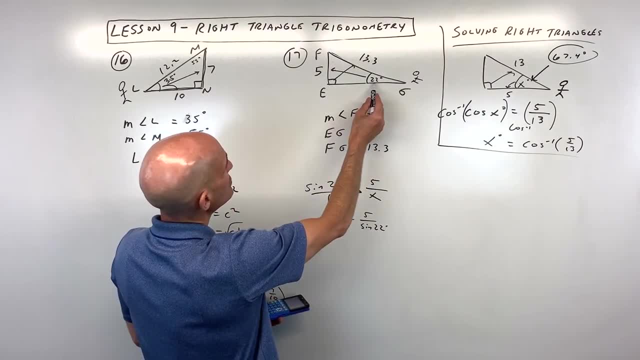 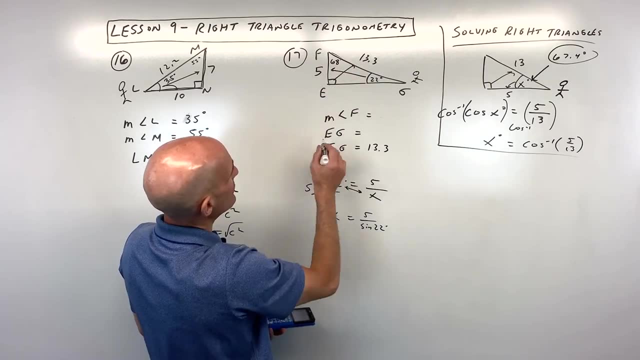 Okay, so that's a good number. Okay, so that's a good number. How about measure of angle F? Well, if this is 22,, this has to be 68,, right, Because that would be 80,, 90, right? 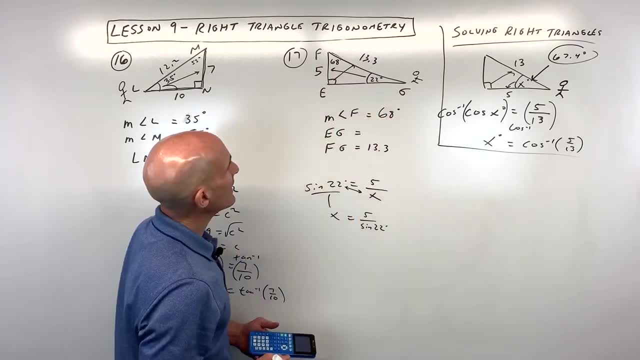 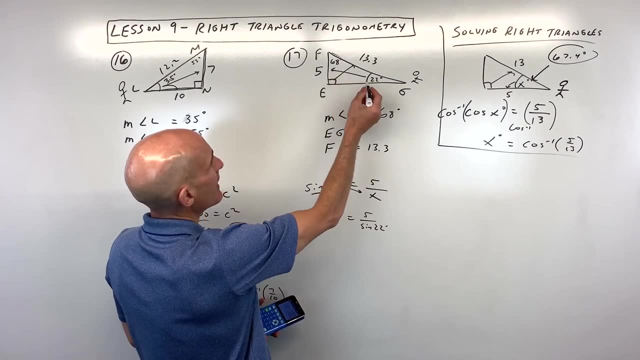 So these two angles have to add up to 90 degrees. Okay, and then now, how about EG? Well, again, I like to go back to the original values. I've had all possible: this 22-degree angle and the 5.. 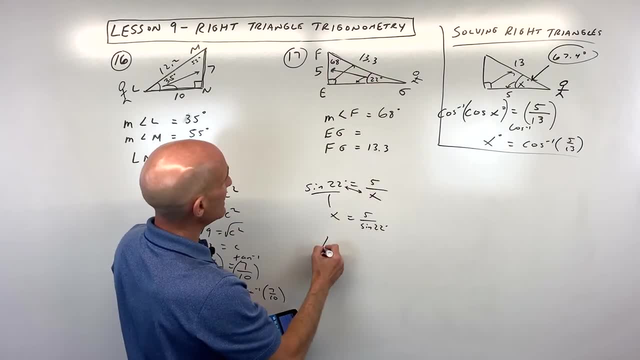 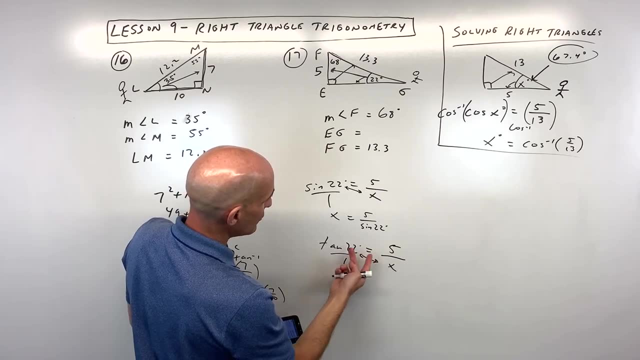 So I've got opposite and adjacent So it looks like we're looking at tangent. So tangent of 22 degrees equals opposite over adjacent. Again, I can switch these on the diagonal. X over 1 is just: X equals 5 divided by the tangent of 22.. 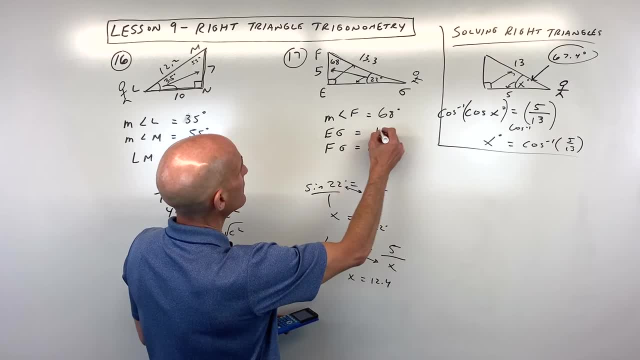 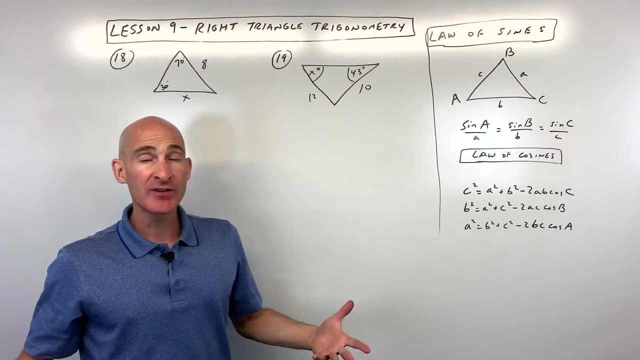 And that's coming out to 12.4. is this missing side right here And you solve the triangle. You found all the sides, all the angles. Okay, up to this point we've been talking about right triangle trigonometry. 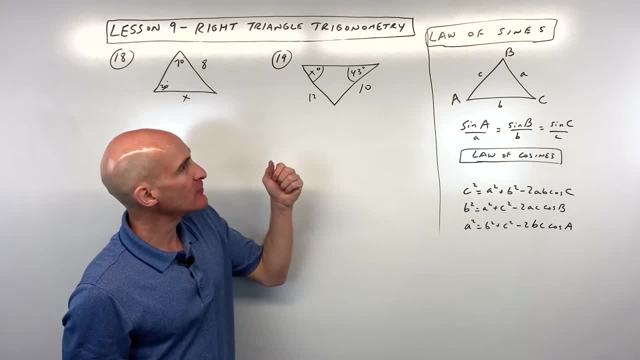 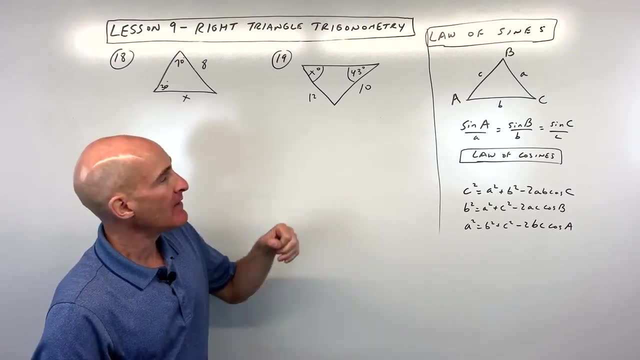 when you have a 90-degree angle, that right triangle. But what happens if you don't have a right triangle? How do you approach solving for a missing side or a missing angle? That's what we're going to talk about now And that's referred to as using the law of sines. 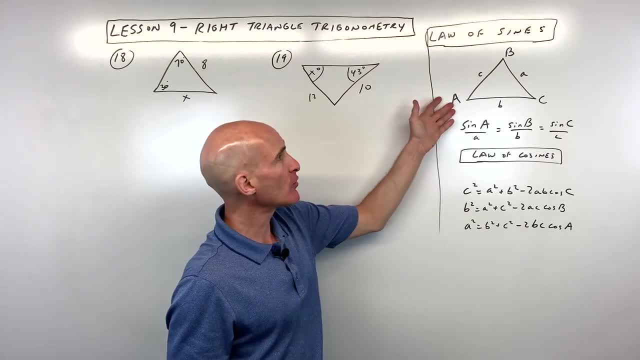 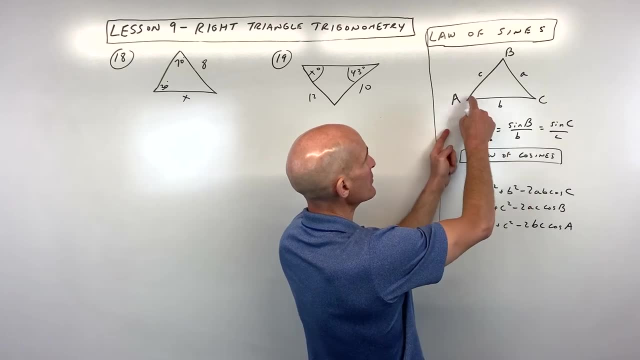 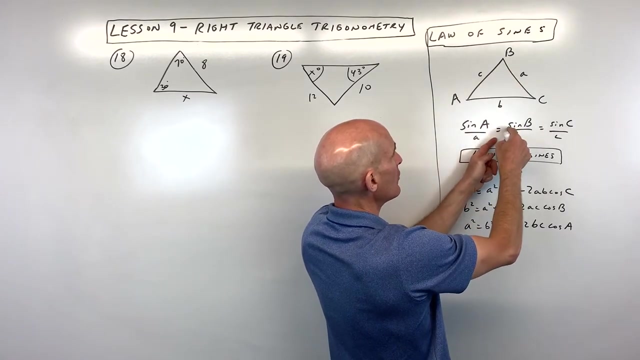 or using the law of cosines. Let's start with using the law of sines first. So the way the law of sines works is: you have this extended proportion where the sine of angle A divided by its side opposite, that ratio is equal to the sine of angle B over its side opposite. 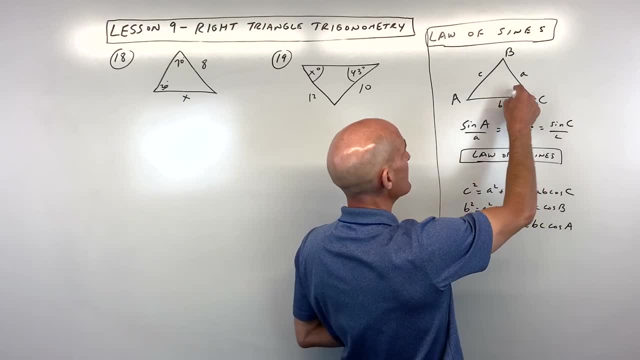 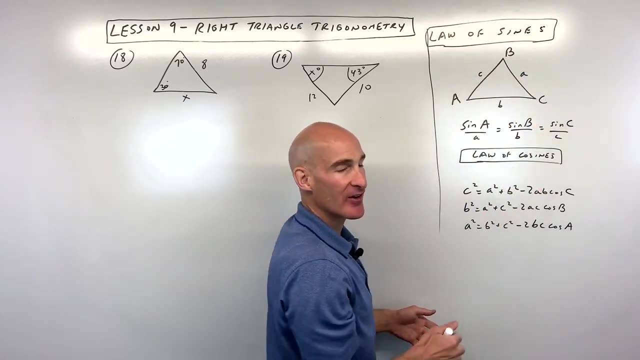 Okay, and that ratio is equal to the sine of angle C over its side opposite. So what I like to think of is the angle on the side across the triangle, The angle on the side across from one another as like a pair. Okay, they kind of go together. 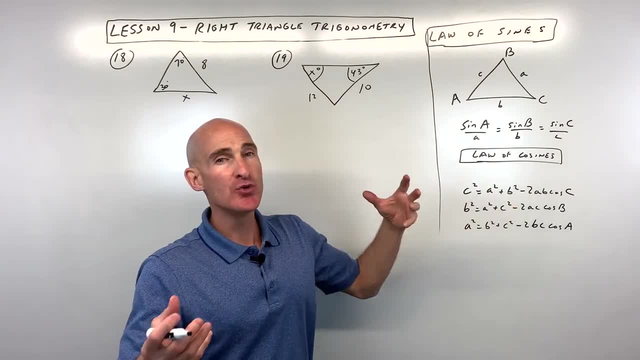 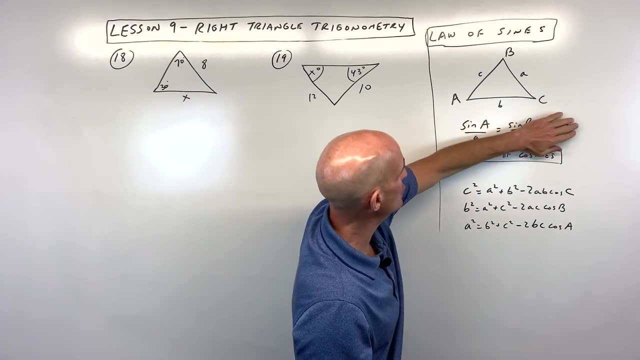 And what you can do. if you have only one unknown, one missing quantity, you can solve for that missing quantity. You only need to use two of these ratios to form a proportion, Like you could use the last two or you could use the first two. 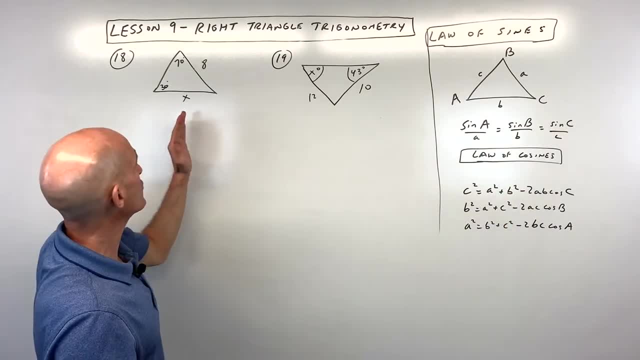 or the first and the last. I'll show you a couple examples so you can see how this works. So you can see we don't have a right triangle. We can't just use our regular SOHCAHTOA or sine cosine tangent. 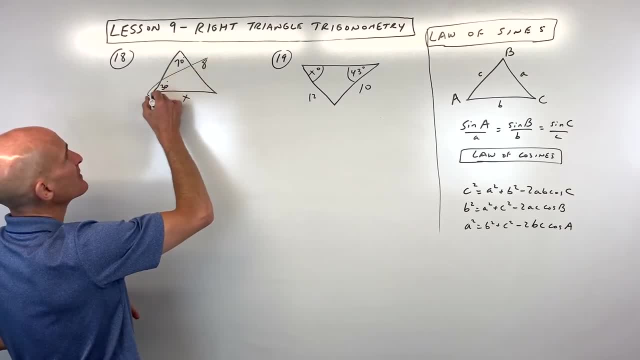 But we may be able to use the law of sines. So what I do is I usually draw, like I kind of capture the ones across from each other. I think of them as a pair. So here I can see that, okay, the sine of the angle, sine of 30 degrees. 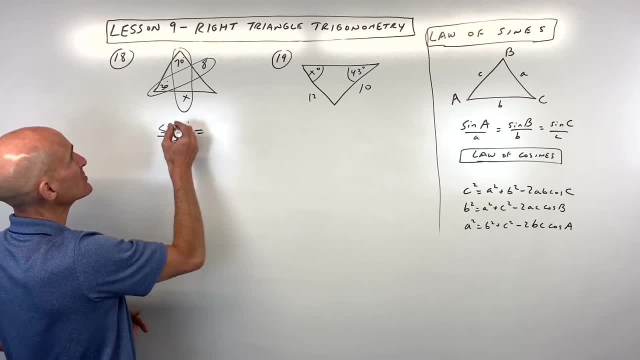 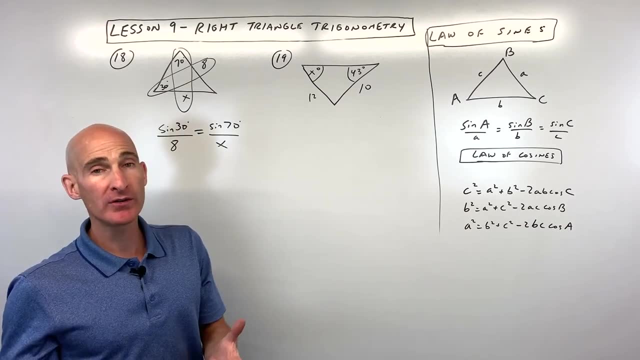 over its side opposite 8,. that ratio is equal to the sine of this angle in the triangle over its side opposite x. We only have one unknown, okay, one variable. We can solve for it. We're going to cross multiply. 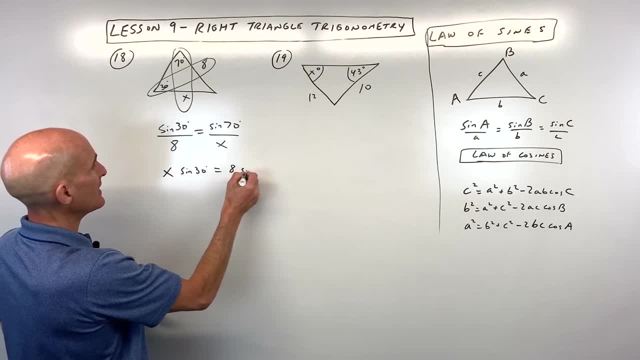 So x times the sine of 30 degrees equals 8 times the sine of 70 degrees. Divide both sides by sine of 30, okay to get x by itself. Whatever we do to the left, we have to do to the right. 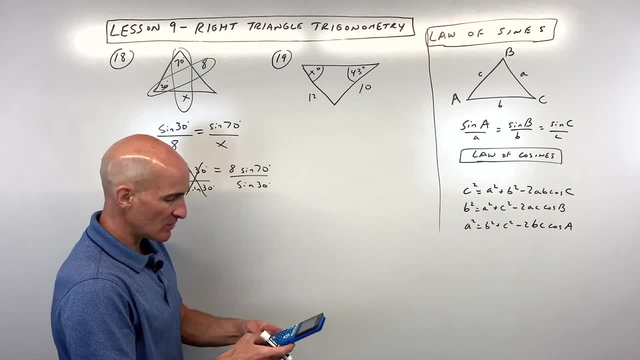 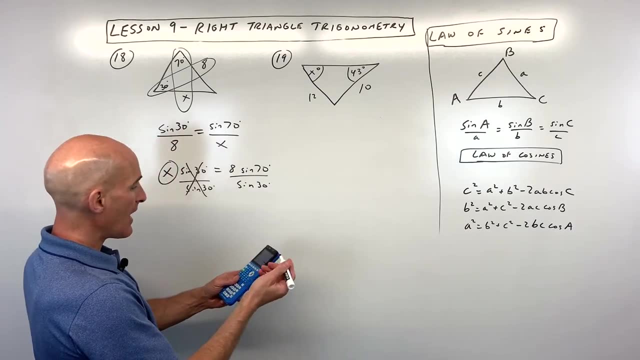 And now we're going to go to the calculator and see what that comes out to. So let's see, We've got 8 sine 70, divided by sine of 30. Okay, so I'm getting about 15 approximately. So that's the length of this missing side right here. 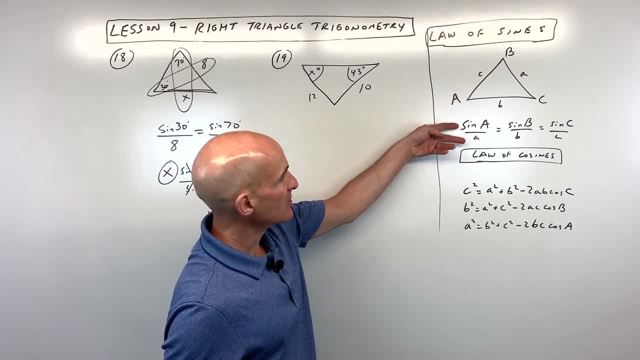 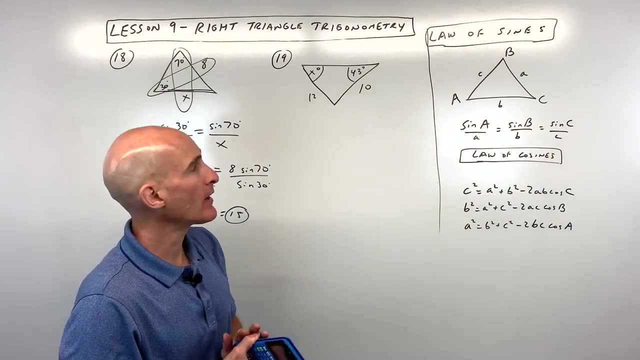 Now sometimes in some books, what they'll do is they'll write this as the reciprocal. They'll say: a over the sine of angle a, b over the sine of angle b, c over the sine of angle c. Another important point I want to mention is notice how all the angles are denoted with capital letters. 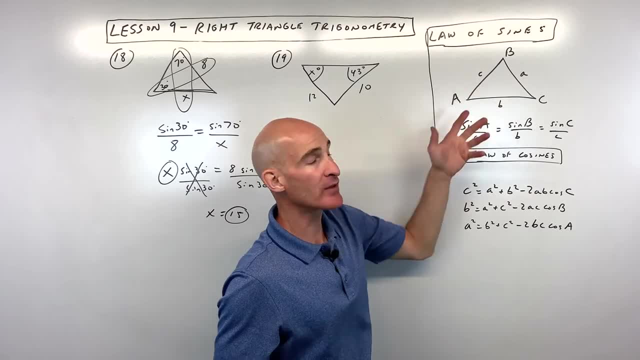 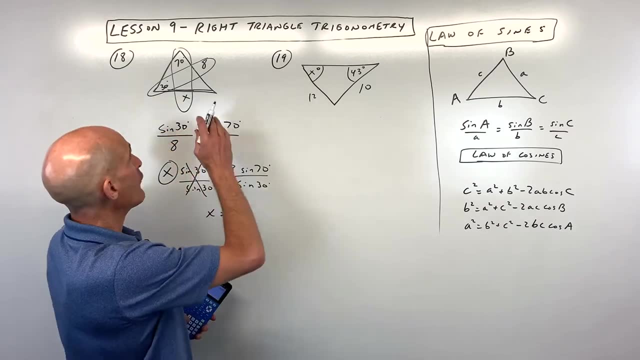 and the side lengths. okay, the sides are denoted with lowercase letters, So that's how you can kind of tell in these formulas if you're working with an angle or a side. Now, if we had more than one unknown, we wouldn't be able to solve it using the law of sines. 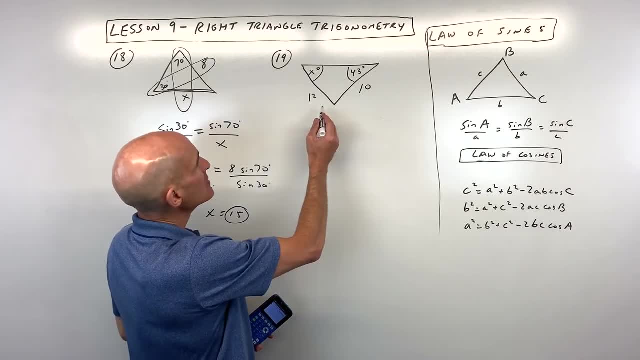 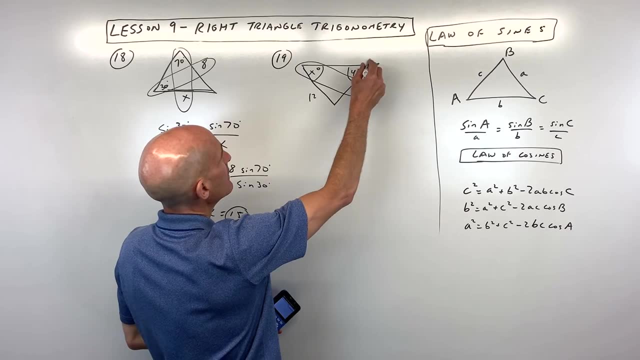 We'd have to use some other technique. Let's look at number 19 now. Here we're trying to solve for the missing angle, Here we're trying to solve for the missing side. But let's look, here We've got a pair. 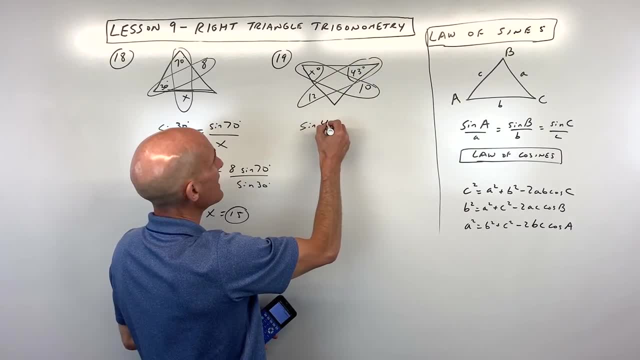 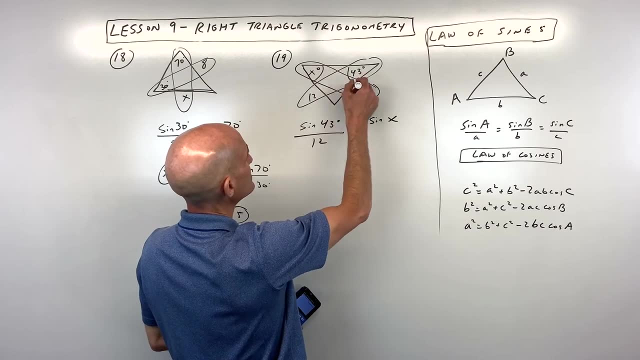 We've got a pair, Okay, so it looks like we're going to be able to do this using the law of sines. We have the sine of 43 degrees over its side opposite, which is 12.. That ratio is equal to the sine of x degrees over its side opposite, 10.. 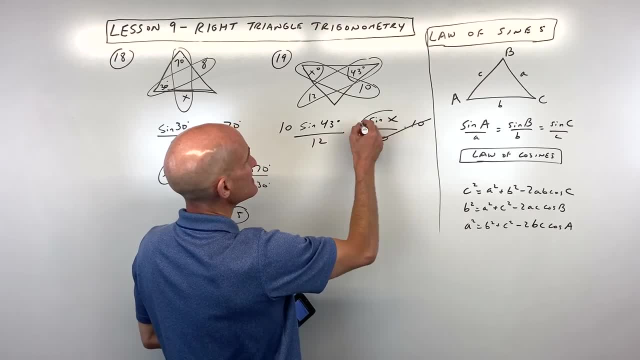 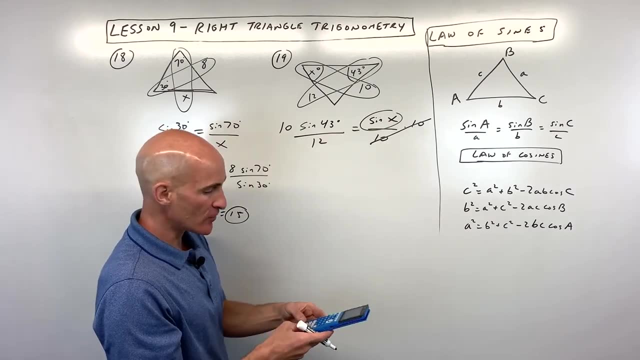 All we have to do is multiply both sides by 10 to get sine of x by itself. But whenever you solve for the missing angle you have to do the sine inverse. Let me see what this comes out to first, just to do it in steps so you can kind of see how this works. 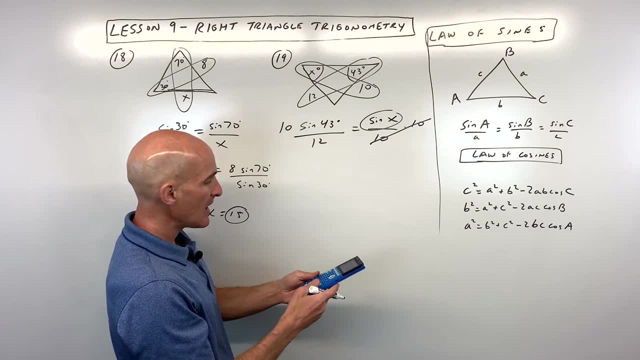 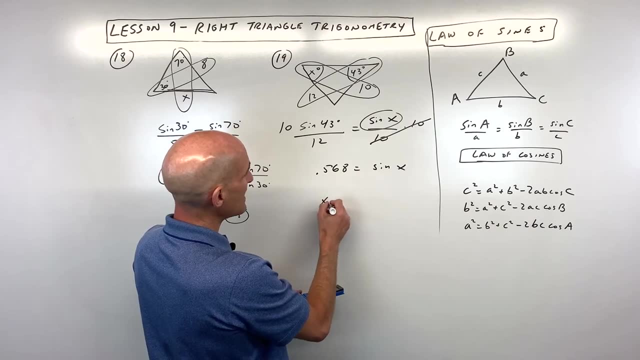 So it's 10 times the sine of 43 divided by 12.. I'm getting about 0.568 equals sine of x. If you take the sine inverse of both sides now we get x equals the sine inverse of 0.568.. 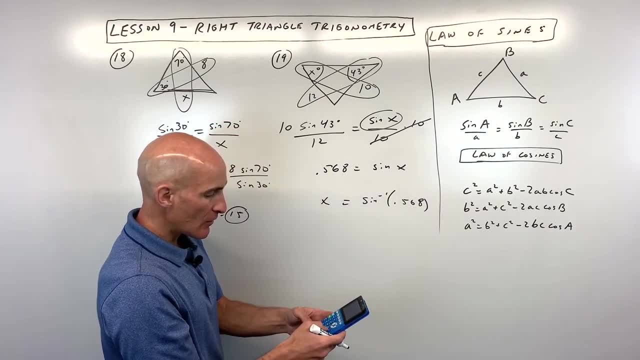 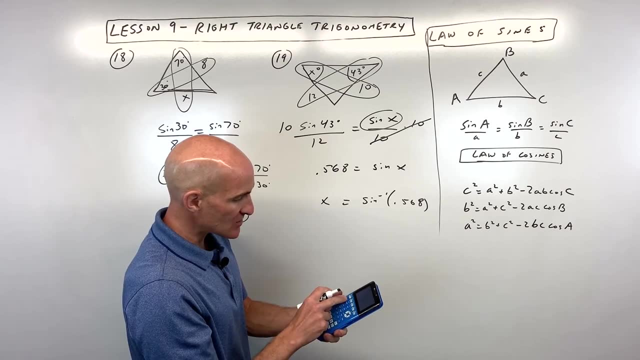 So whenever you solve for that missing angle, you always want to. Now, another thing you can do too when you're doing this on the calculator, if you're doing it in steps, is use that long decimal, Or you can use the previous answer key Just to get a little bit more accuracy. I'm getting about 34.6 degrees. 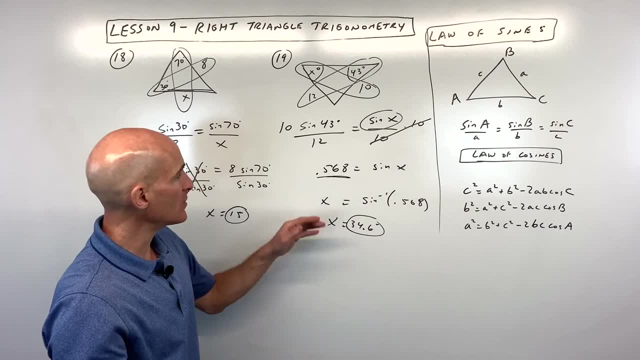 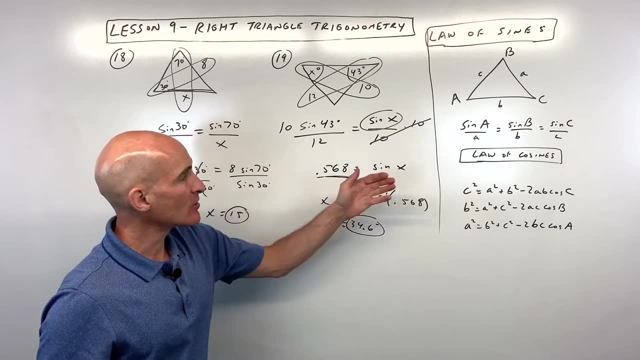 If you do use a decimal, try to carry it a little bit further. You know, don't just use .5 or .6, because you'll be quite a bit off here. And so that's the law of sines. Now we're going to talk about the law of cosines. 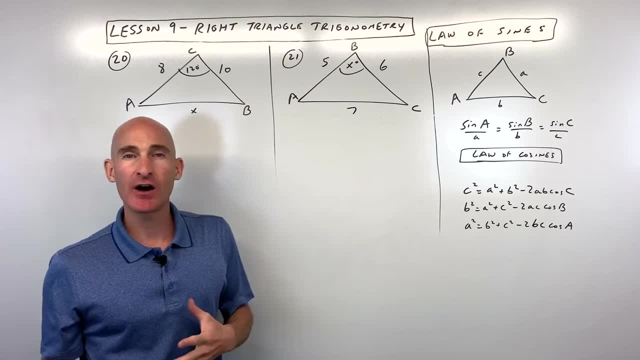 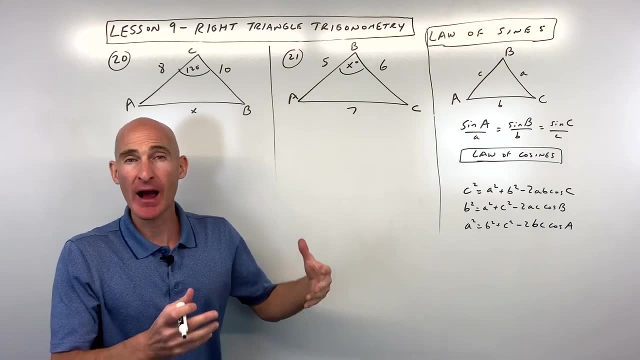 Some books, some courses. they save this law of sines, law of cosines, for like Algebra 2 or even pre-calculus. So if some of this seems kind of challenging, you'll have another opportunity where you'll revisit in those future courses. 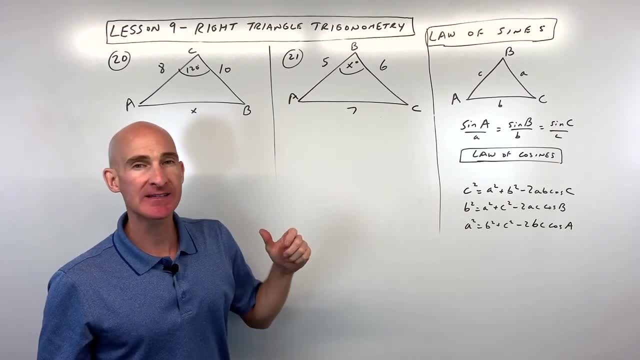 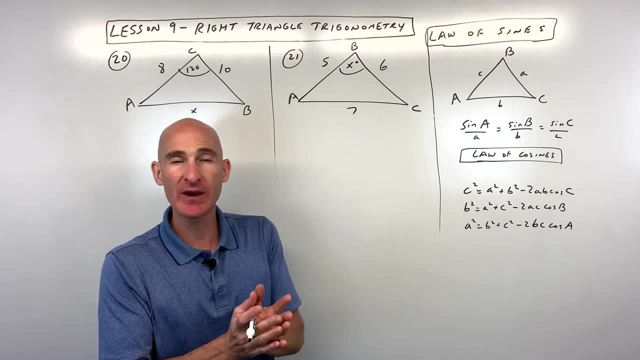 But we'll try to lay the groundwork here. When I was working with the law of sines, I was just showing you some simple examples As you go further on and further deeper into this. when they give you limited amounts of information, sometimes you can actually construct a triangle in such a way that you might be able to make the triangle two different ways. 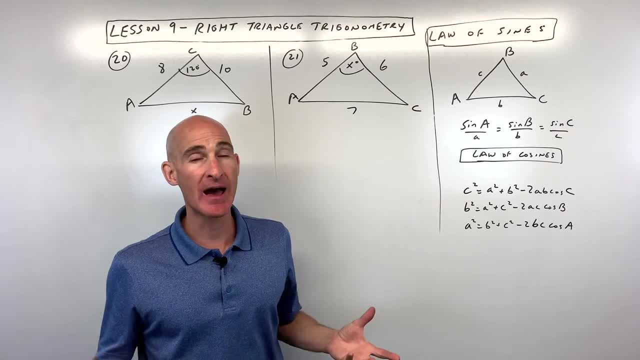 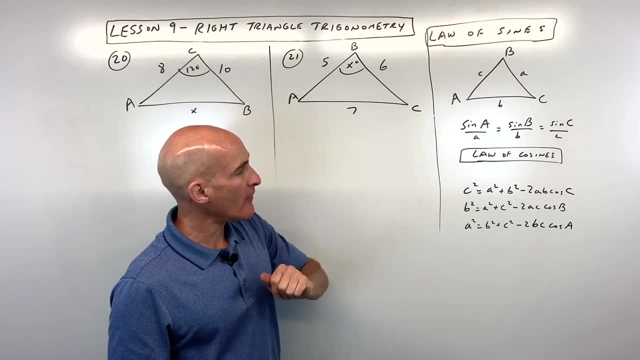 Or maybe the triangles can't even be made with those dimensions, so it's not possible. But I just showed you some basic ones where there was just one triangle possible. So when you talk about law of cosines, when do you use the law of cosines? 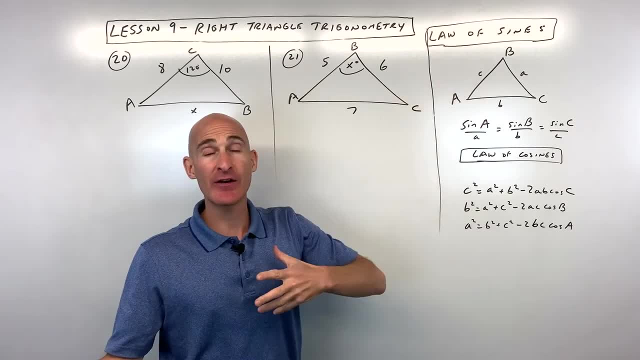 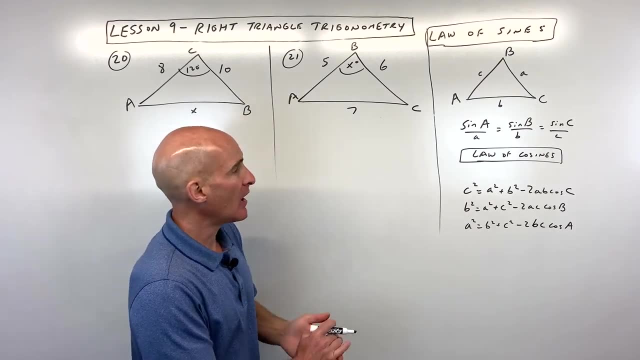 Well, you can try to use the law of sines. and if you find out you have more than one unknown and you say, well, the law of sines isn't going to work, then you can try to use the law of cosines. But an easy way to remember when to use the law of cosines is if they only give you three sides. 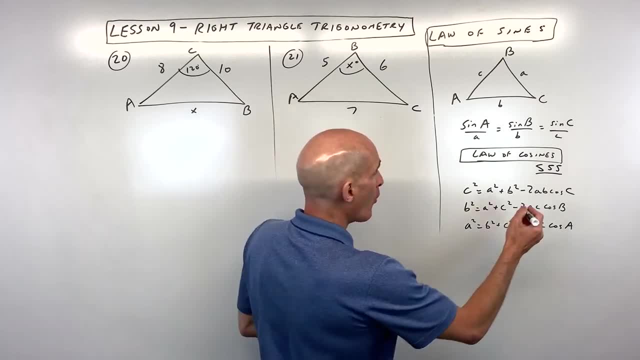 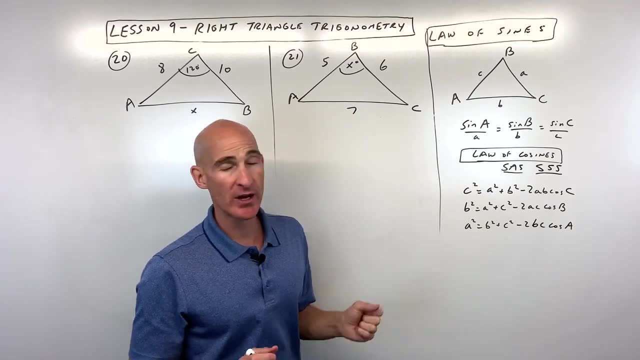 like side, side, side, but nothing else. Or if they give you side angle, side, like the angle in between the two sides. So if they give you those three quantities, then you'll also want to use the law of cosines. So that's an easy way to remember the law of cosines. 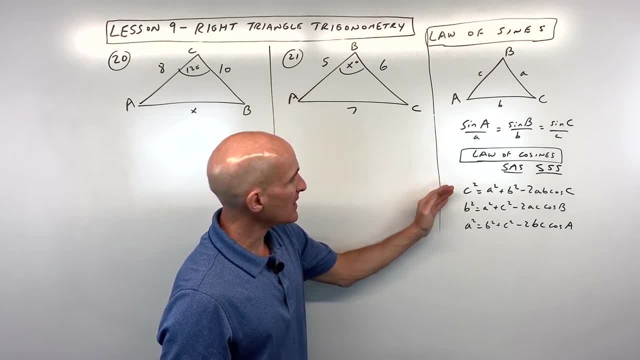 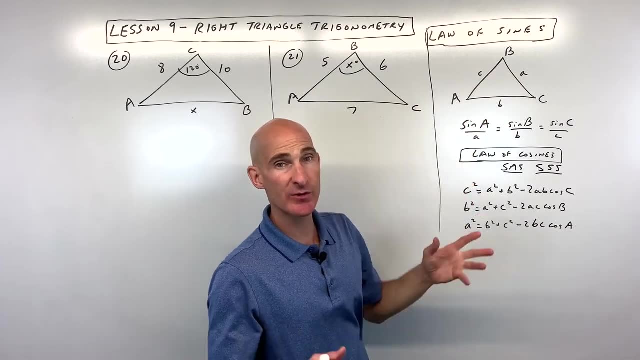 So let's look at an example here. So first of all let me kind of show you So these triangles. we're going to use the same kind of setup here with angle ABC and the sides across from angle AB and C with the lower case letters. 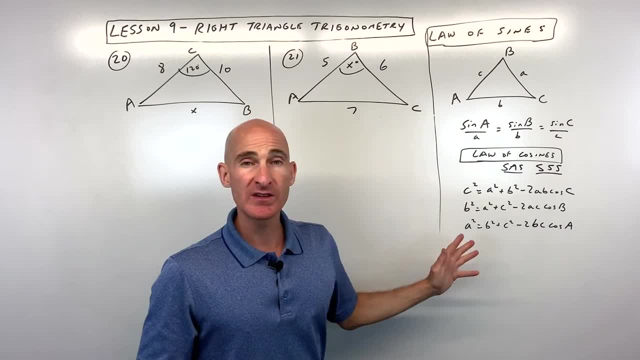 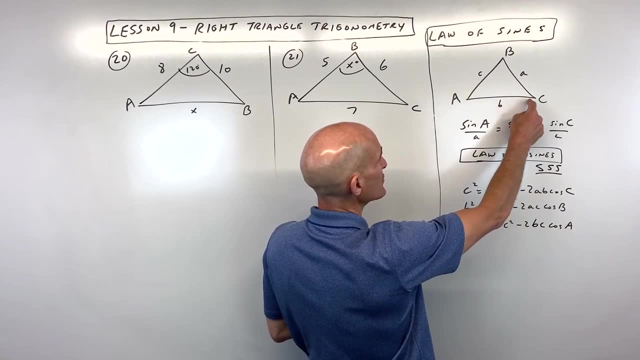 So we've got three different forms of the equation, depending on if you're using. let's say, you're trying to solve for side C and you know angle C, you would use this formula. If you were trying to solve for side B and you knew angle B, you would use this formula. 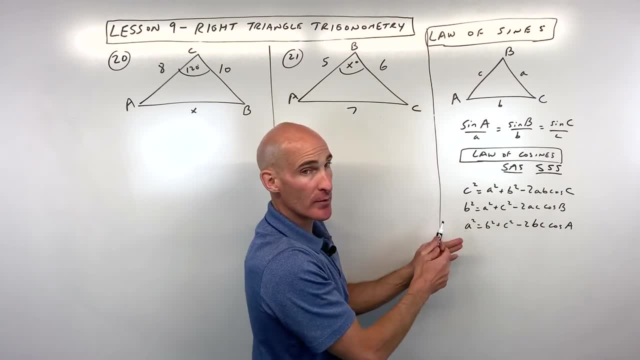 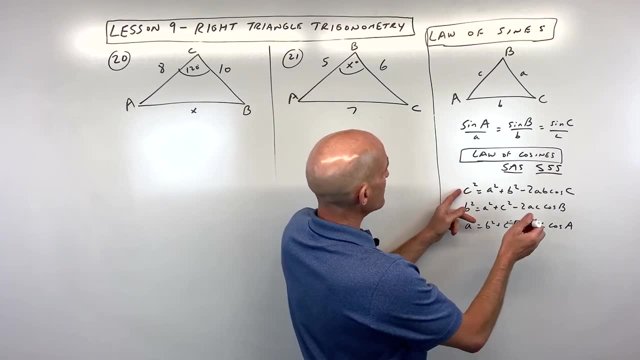 If you were trying to solve for side A and you knew angle A, you would use this formula. But the way that I sometimes remember these formulas and I tell students to remember them is: see you can think about. see how the side C and the angle C- they're across from each other in the triangle. 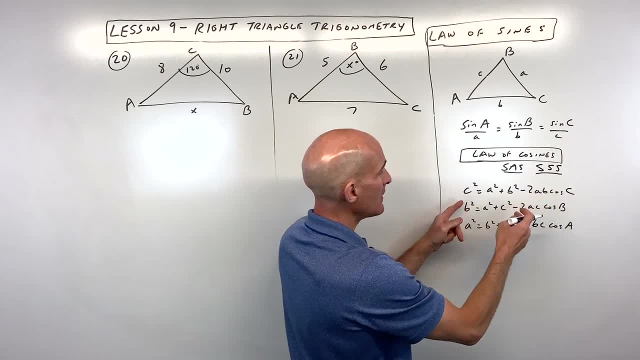 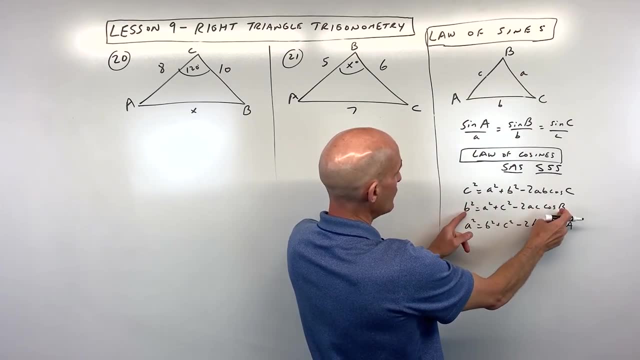 and they're also across from each other at opposite ends in the formula. And then you can see A and B. A and B, those are the two sides that make up, you know, angle C, Whereas over here, if you look at angle B and side C, they're opposite ends in the formula. 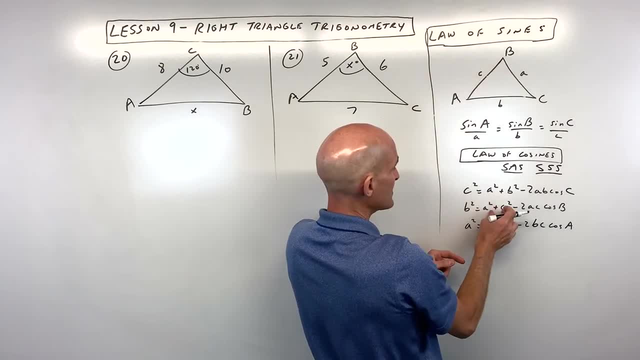 And then you can see A and C, A and C. those are the two sides that make up angle B. Same thing here: angle A and side A. they're across from each other in the triangle, across from each other in the formula. And then we have B and C, B and C. those are the two sides that make up angle A. 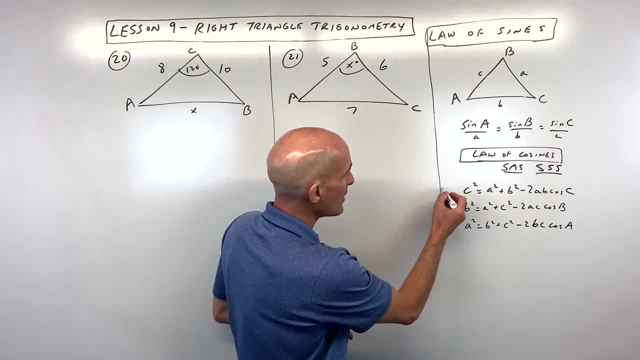 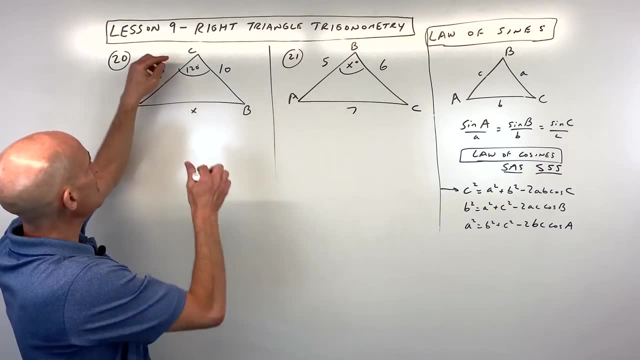 So kind of a way: if you memorize one of these formulas- I usually memorize this top one- you'll be able to remember the other two fairly easily. So let's jump over to number 20. here You can see we're given side, angle, side. 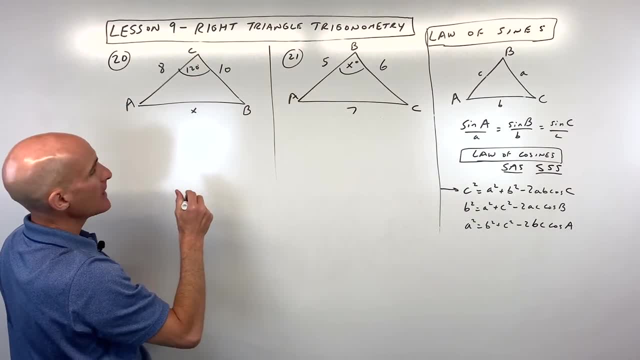 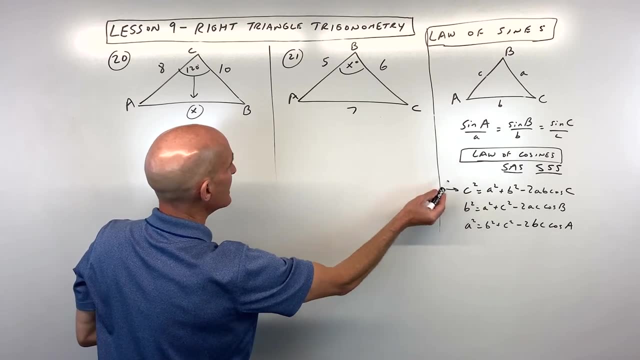 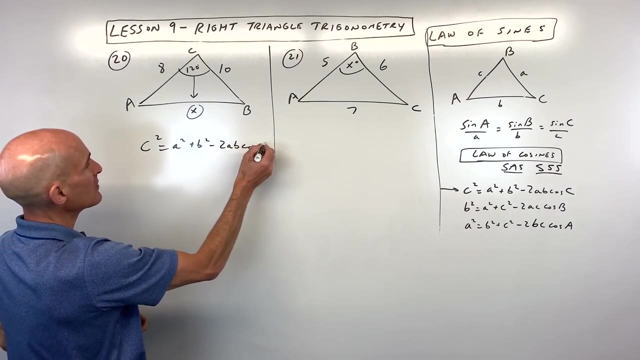 Okay, side, angle side. So we're going to use law of cosines and we're trying to solve for the side across from angle C. Okay, I just labeled it X, but we're really trying to solve for this side C here. So let's write down our formula: C squared equals A squared plus B. squared minus 2AB. cosine C. 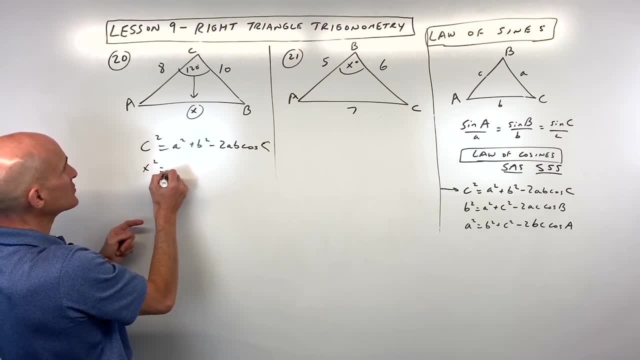 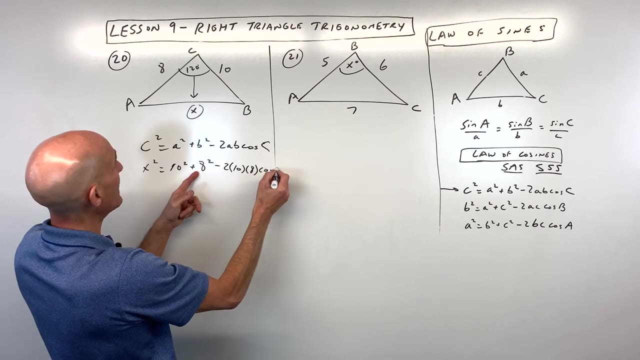 Okay, so we're trying to solve for side C, that's X. so we'll say: X squared equals A squared, that's the side across from angle A. that's going to be 10 squared plus B squared, that's the side across from angle A. So angle B, that's 8 squared minus 2 times A times B, times the cosine of angle C, which is 120 degrees. 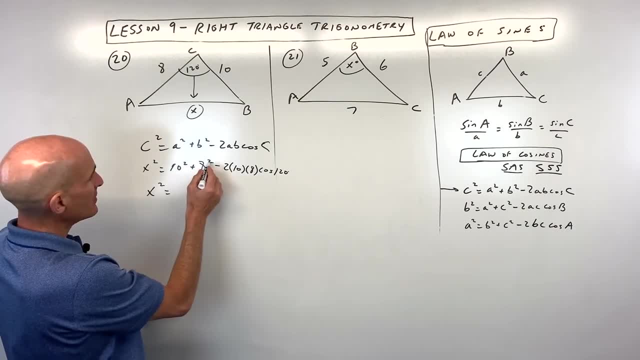 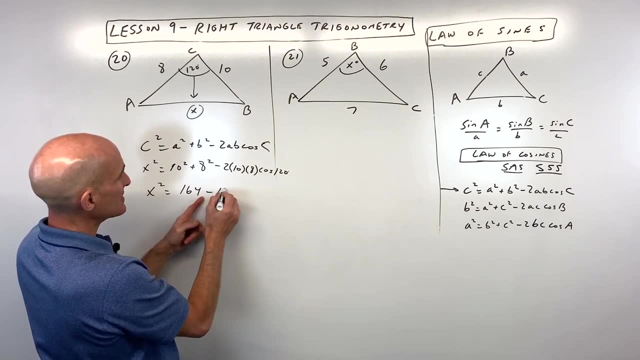 So now let's go ahead and simplify this. We've got: 10 squared is 100, 8 squared is 64.. We add those together, that's 164.. 2 times 10 times 8 is 160. so minus 160, cosine of 120.. 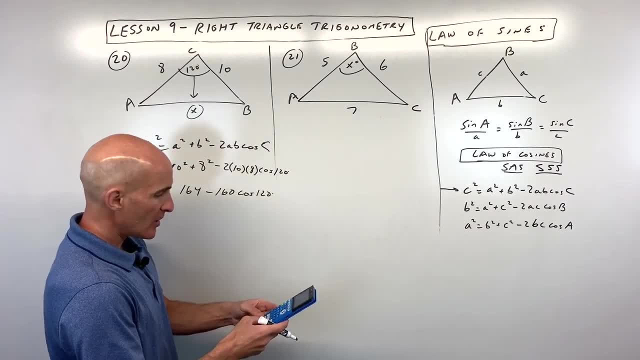 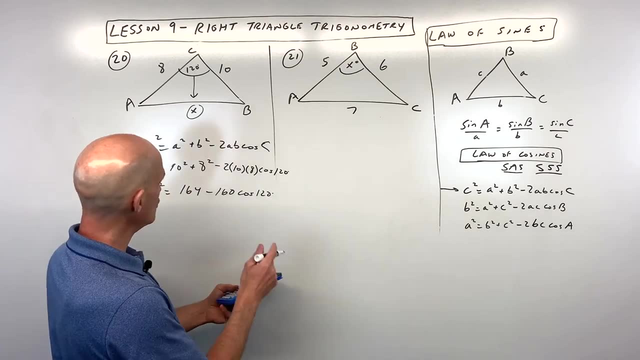 Let's see what this comes out to on the calculator. We've got 164 minus 160.. That's 160 times the cosine of 120.. Now one thing to pay attention to: you don't want to make this 4 times the cosine of 120.. 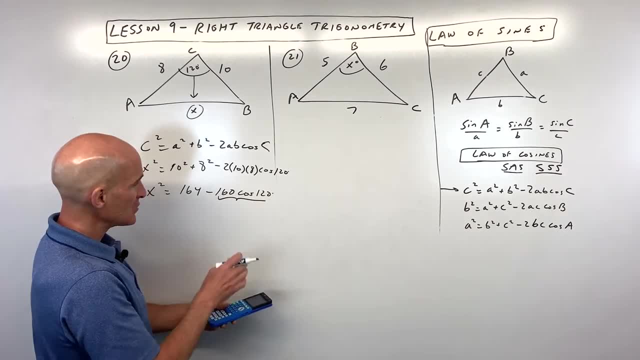 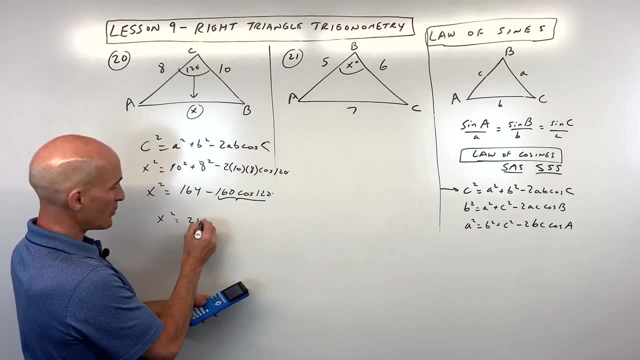 You want to do this part first and then subtract, So you want to do the PEMDAS. multiplication comes before subtraction, So this comes out to X squared equals 244, and if we take the square root to get just the side length by itself, we get about 15.6.. 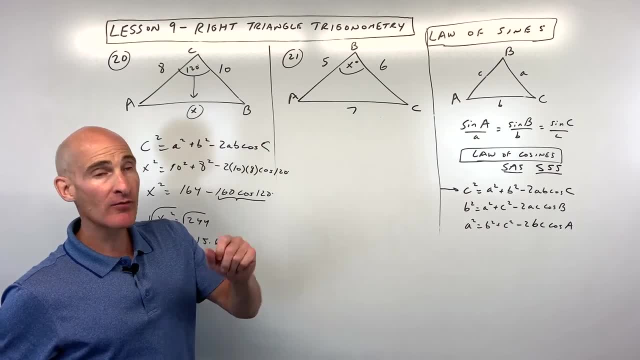 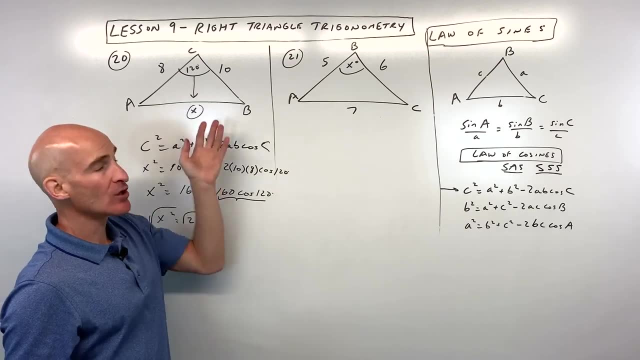 So that's the missing side. Now, if you're solving the triangle, you want to find all the angles, all the sides. You only have to use the law of cosines at most one time, Then you can switch to the law of sines. 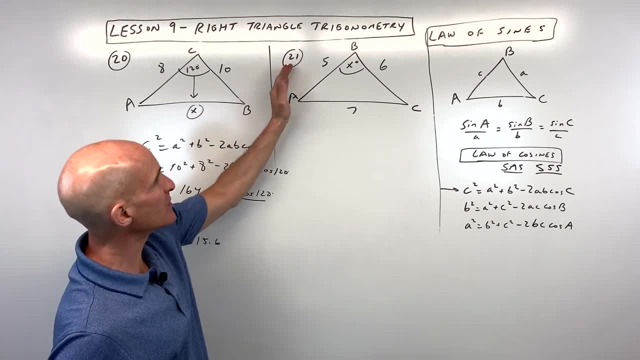 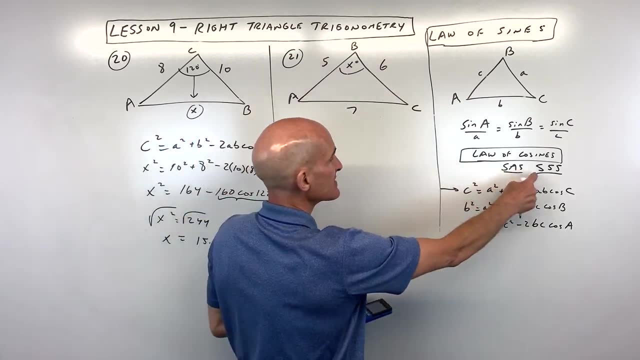 Okay. So for number 21, this one's a little bit different, because now we're solving for the angle, not the side length. And notice, we're given side side side, See side side side. So we're going to use the law of cosines again. 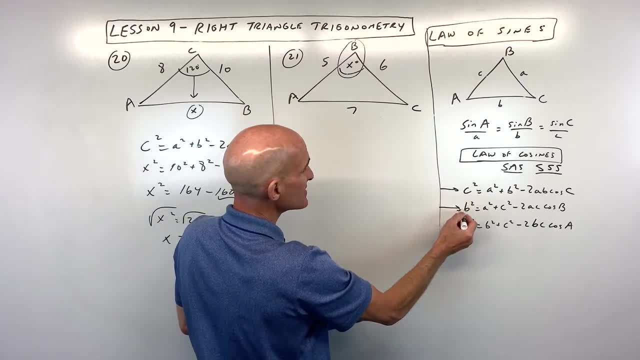 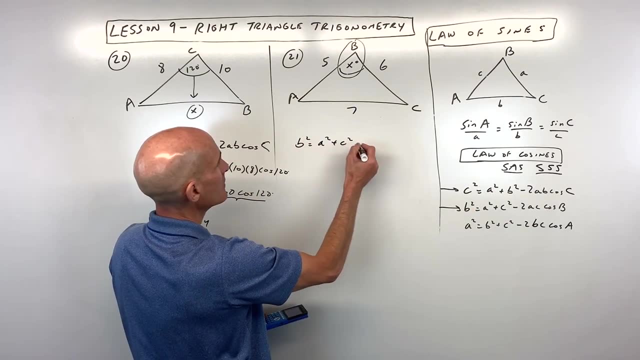 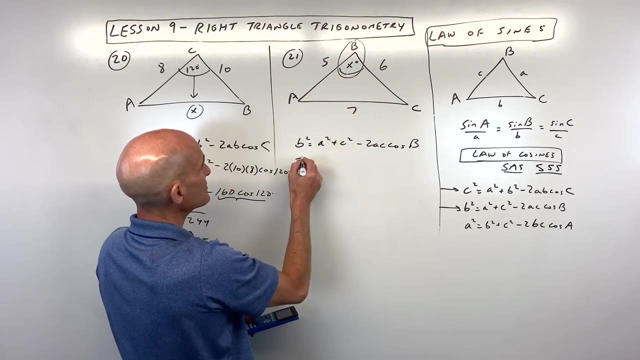 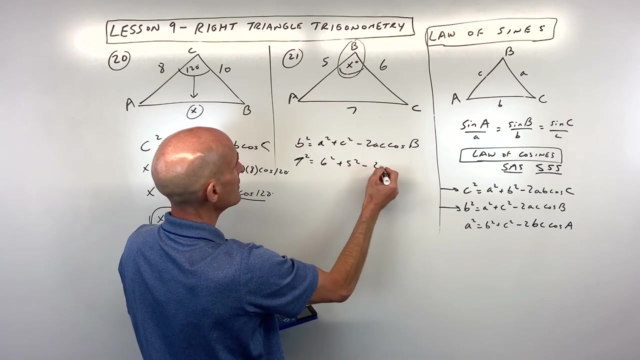 But notice how we're trying to solve for angle B. So I'm going to use the second formula here that contains angle B. So we have B squared equals A, squared plus C squared minus 2AC cosine angle B, So this is: B, is going to be 7, squared equals A squared, which is going to be 6, squared plus C squared, which is 5 squared minus 2 times, 6 times 5 times the cosine of X degrees. 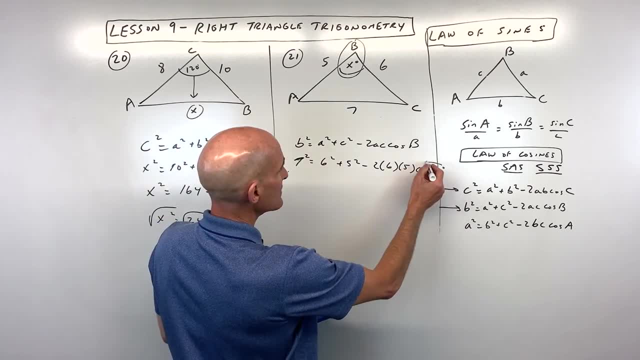 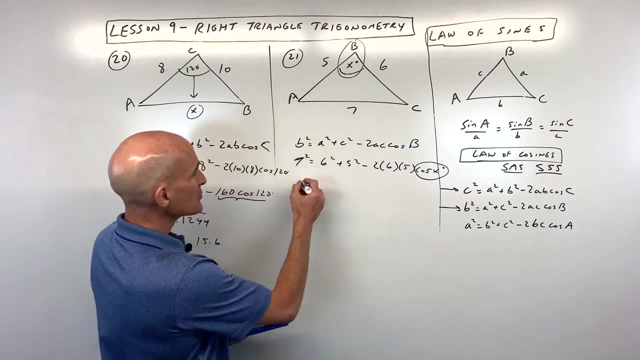 Now this one's a little bit more challenging, because what we have to do is get this cosine X by itself on one side of the equation And then take the cosine inverse to solve for the missing angle. So let's just do this step by step. 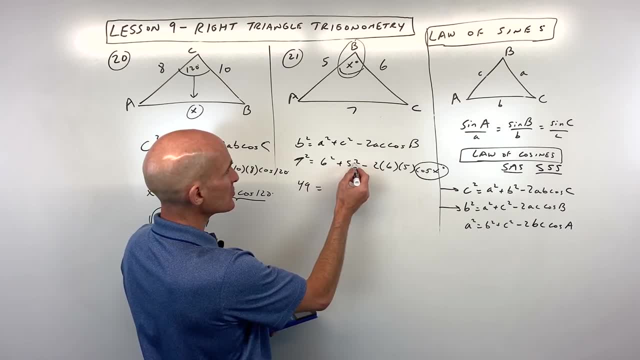 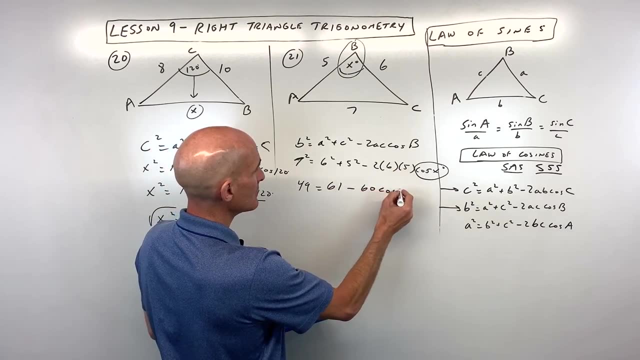 So 7 squared is 49.. 6 squared is 36.. 5 squared is 25.. So if we add those together we get 61.. 2 times 6 is 12, times 5 is 60.. Let's subtract the 61 from both sides. 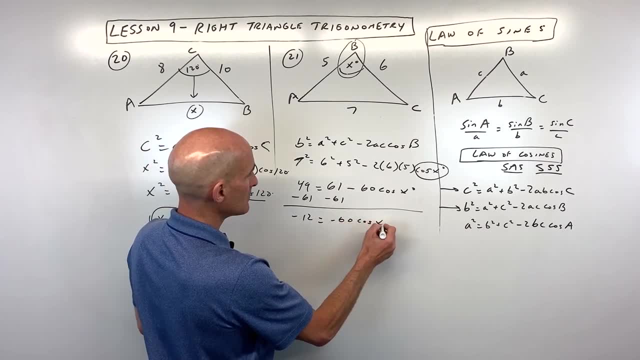 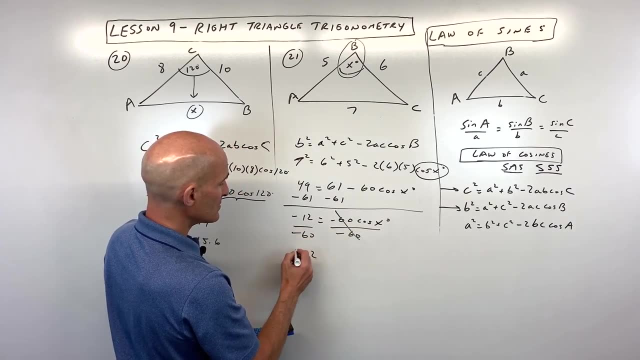 That gives us a negative 12.. And if we divide both sides by negative 60. That gives us 1 fifth, which is like 0.2.. But now what we have to do to get X by itself is: take the cosine inverse. 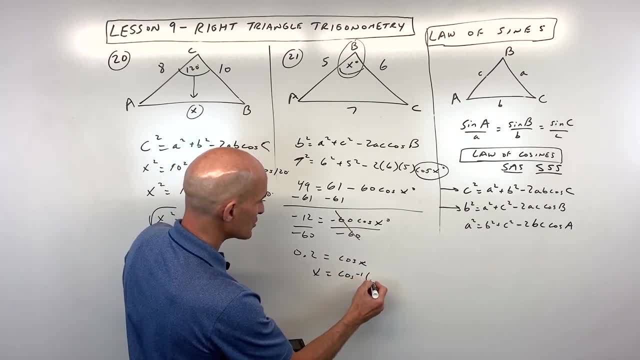 Whenever you're solving for the angle, you're going to use the inverse trig functions, And so let's see what that comes out to: I'm getting 78.5 degrees and you've solved for the missing angle. So law of sines, law of cosines. Remember, this is when you don't have a right triangle.